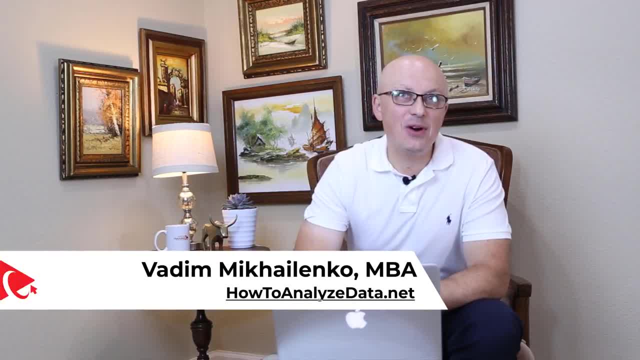 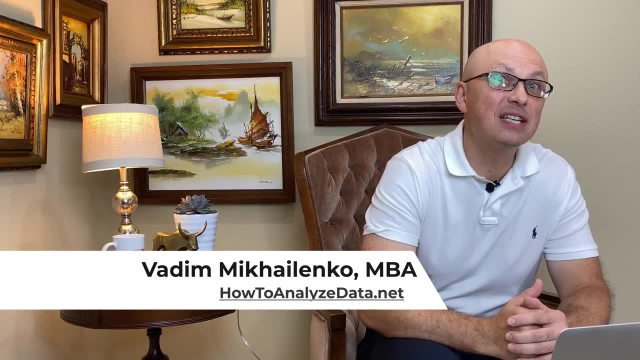 Hi there, this is Vadim Mikhailenko, and in this video I'll share with you how to pass an employment assessment test. In this video I will share with you sample questions we see on the tests. I will have some questions for you to try and I'll show you tips, tricks and hacks on how. 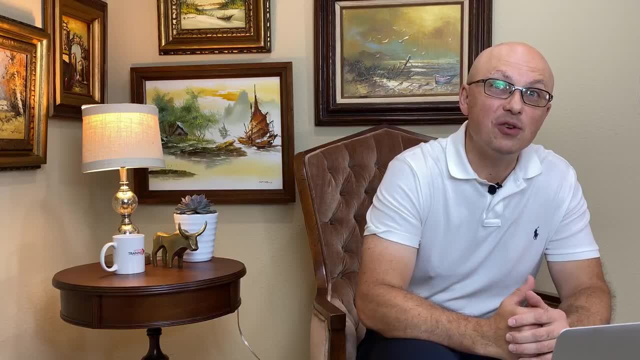 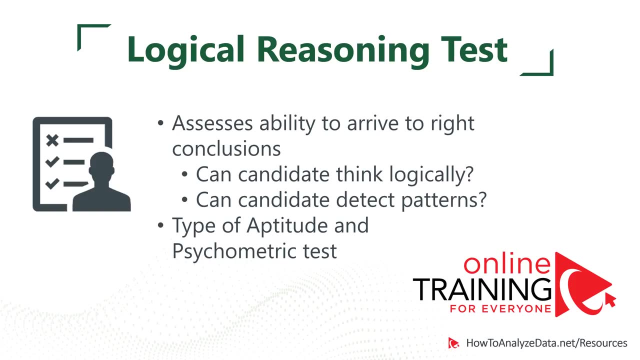 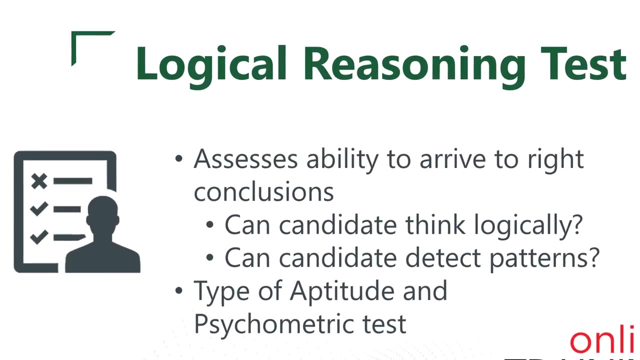 to get ready and pass the test. I will also share with you some additional test resources that might benefit you and might help you to get ready for the test quickly. Logical reasoning test is designed to assess candidates ability to think consistently at the correct conclusions. as a result of this, 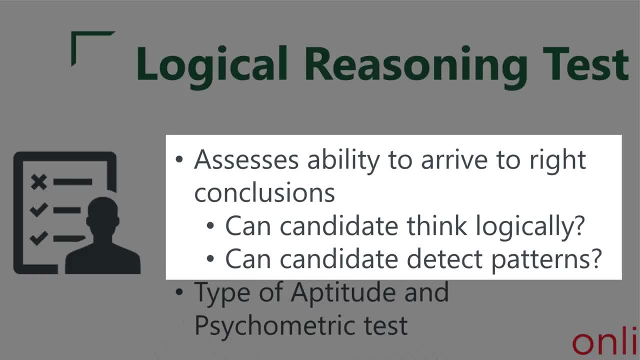 thinking. The main purpose of the test is to assess the logical thinking in dealing with the problem. The main purpose of the test is to assess the logical thinking in dealing with the logical reasoning test. The main purpose of the test is to assess the logical thinking in dealing 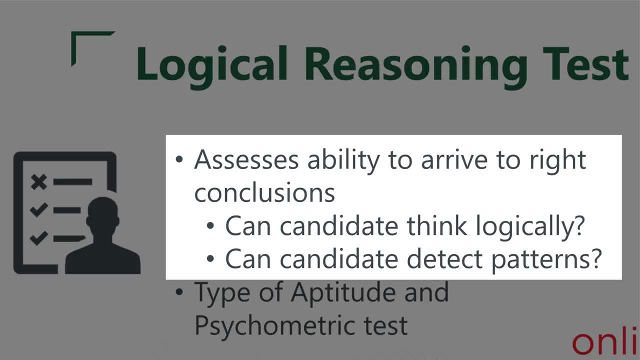 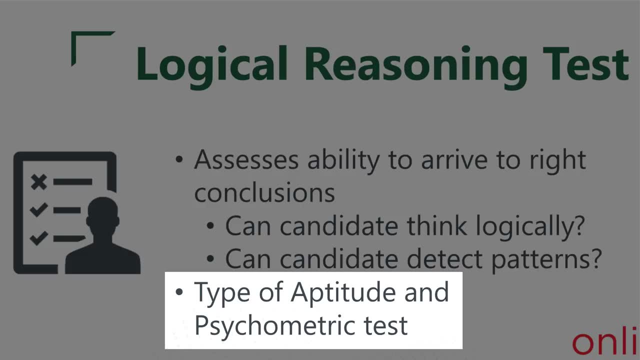 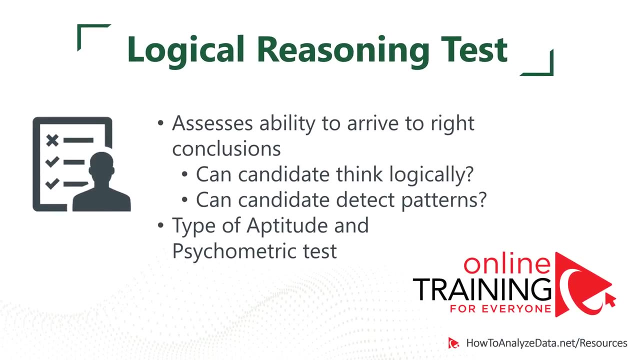 with the problems and situation encountered during work. Logical reasoning test is a type of aptitude and psychometric tests that helps employers to screen candidates in their recruitment process. This test is used as a tool to measure mental ability of the candidate and their logical reasoning. Let me tell. 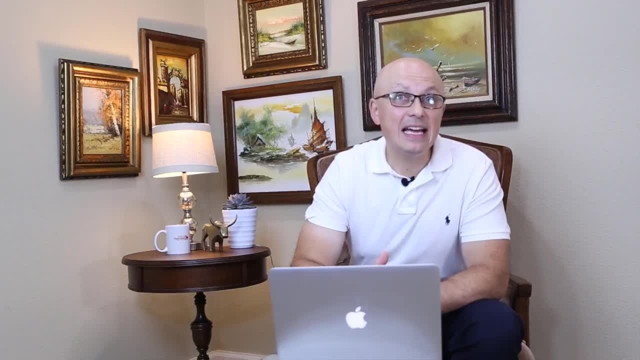 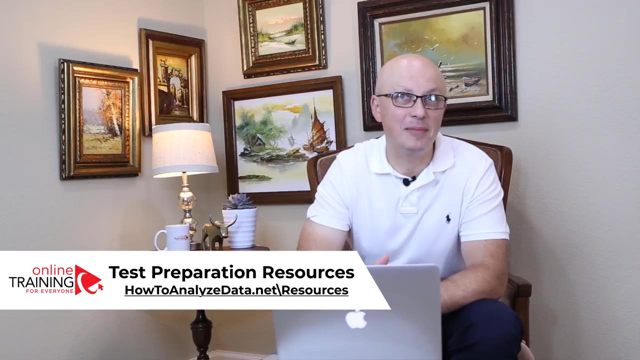 you a little bit about myself. My name is Vadim Mikhailenko and I have MBA and master's degree in computer science. I have been helping people for more than 25 years to get hired and find jobs. I have founded howtoanalyzedatanet website with only intent to help people get employment. 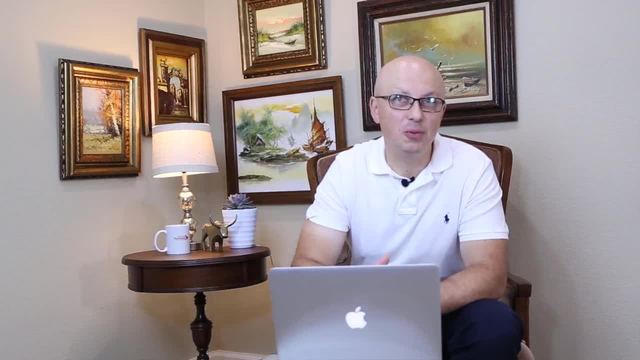 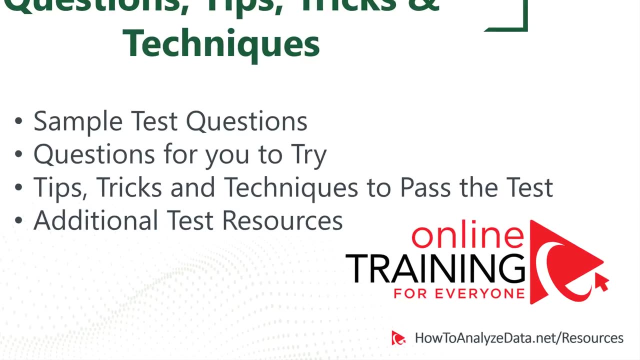 This site helped a lot of people and I'm pretty sure it will help you as well. In this video tutorial you will have everything you need to get ready and pass the test. I'll show you sample test questions with answers and explanations. I will have practice questions. 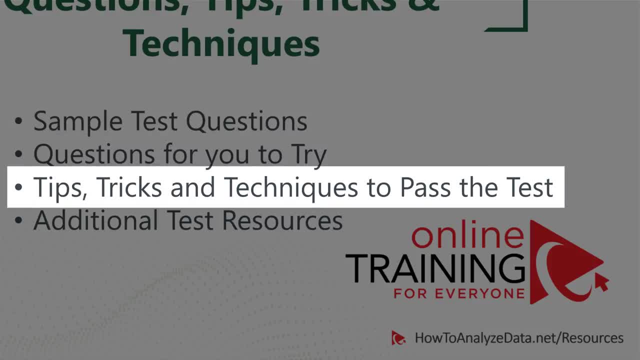 for you to answer. I'll share with you tips, tricks, hacks and techniques that work now to get you ready for the test. I'll share with you tips, tricks, hacks and techniques that work now to get you ready for the test. 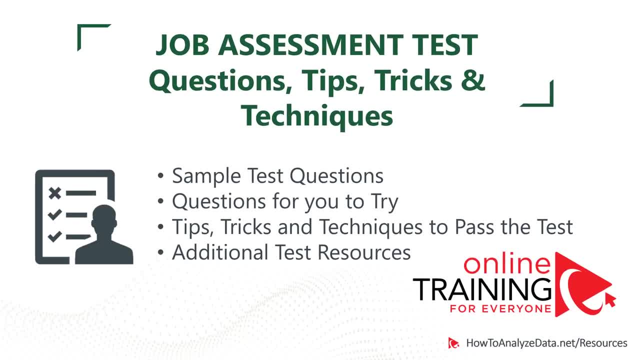 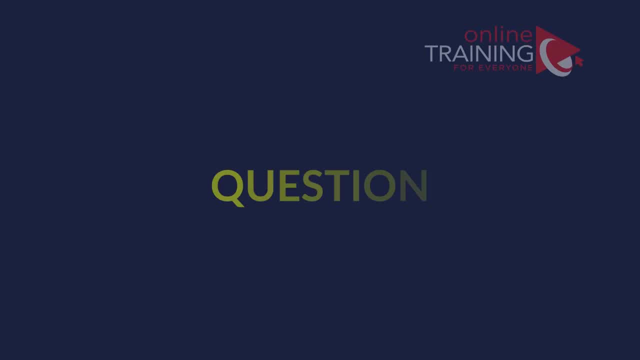 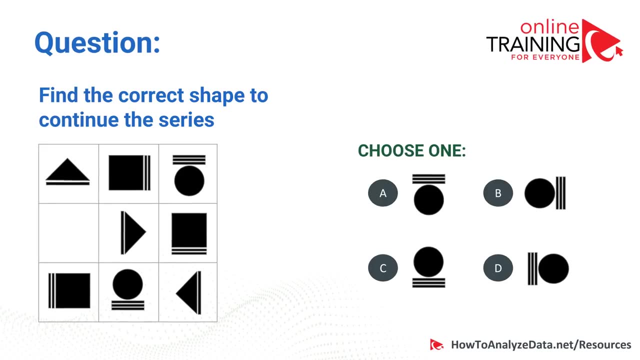 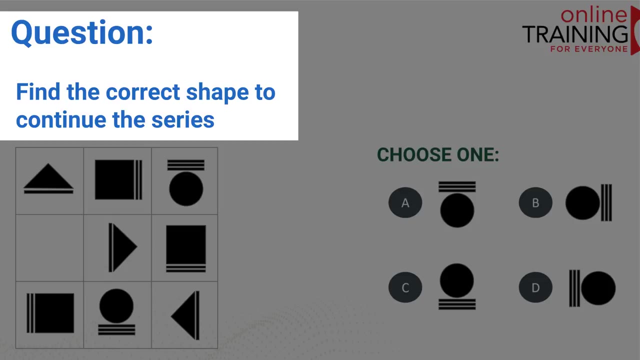 and I'll share with you some additional test resources to get you prepared quickly. And now let's go ahead and jump right to the questions. Now let's look at the very complex question which you see a lot during logical reasoning tests, psychometric tests and the numerical reasoning tests. Find the correct shape to 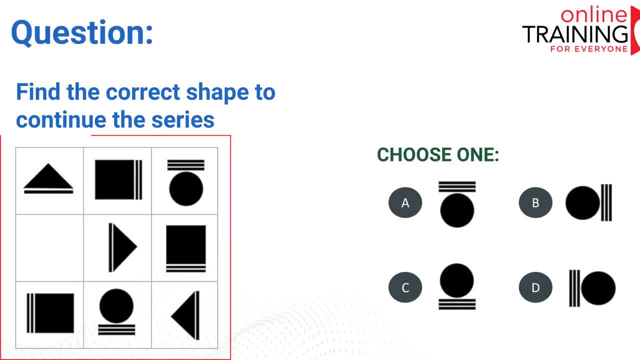 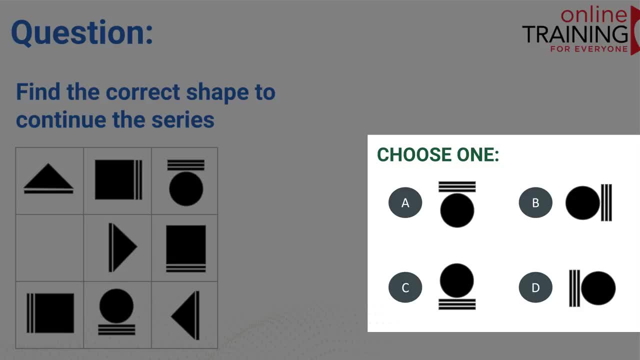 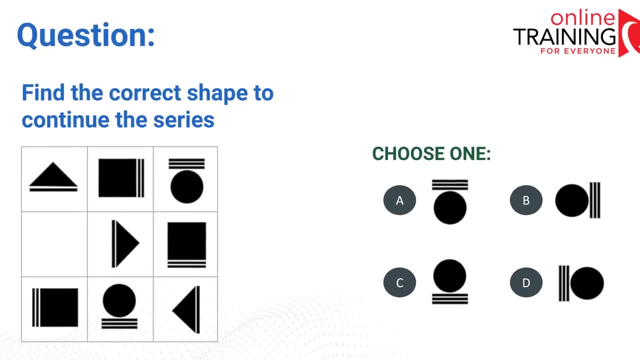 continue the series And what we have here? we have a 3x3 matrix with eight shapes populated and one shape is missing. There are four choices, as usual, but in order for you to calculate the right shape, you need to determine the pattern, And in fact, there are two patterns here on this. 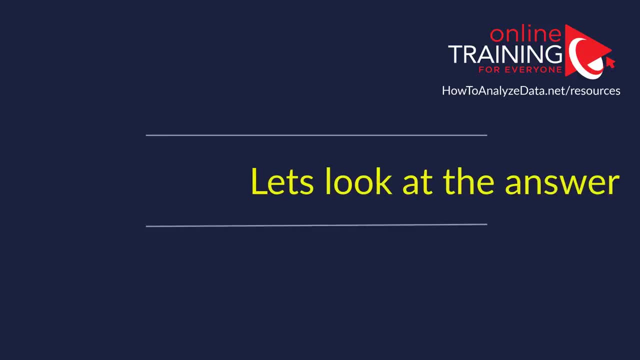 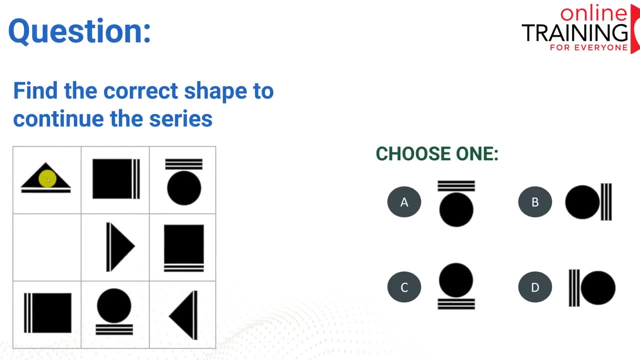 screen. Can you figure it out? Do you know what the right answer is? As I mentioned, there are two patterns here. One is there is a pattern for the shape- Which shape would you choose? And second pattern is the pattern, the lines, and where is the right location for the line itself. now let's go through the detection of 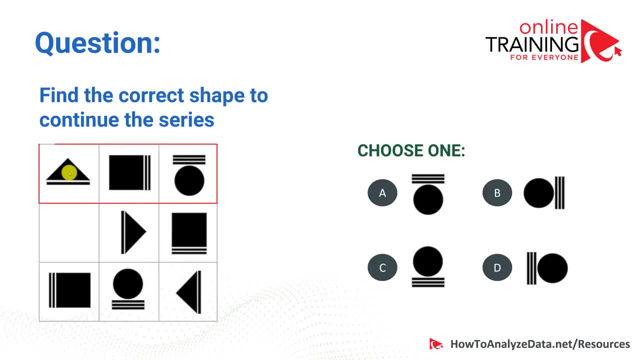 the shape pattern first. so the shape pattern is triangle, square, and then the circle right, so triangle, square, and the next one would be the circle. so we have a circle. that's, uh, the right value here, but all of this other circles. so this was helpful, but not by much, but it just tells us. 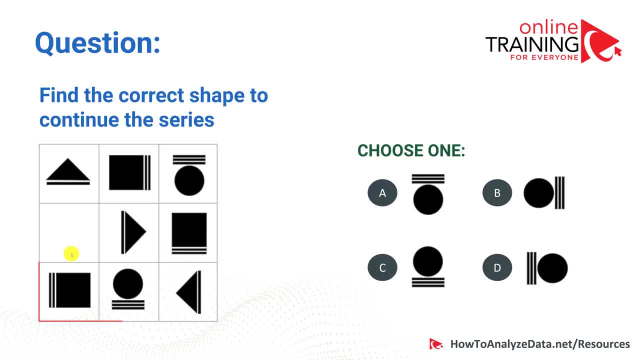 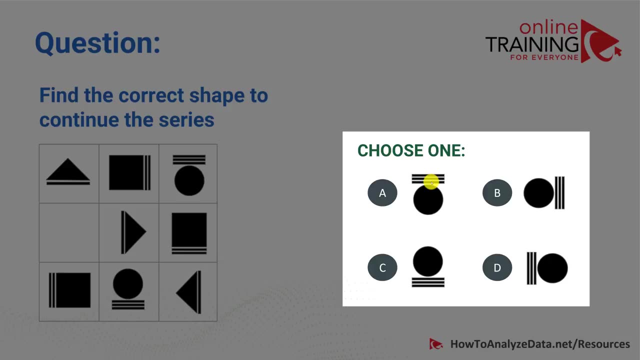 that we are detecting the first pattern and here, if you want to confirm, we have square, circle and then triangle. now the most important part here is to determine on which side of the shape the lines should be located and what we have here. we have four locations, as you can see in the answer. one: 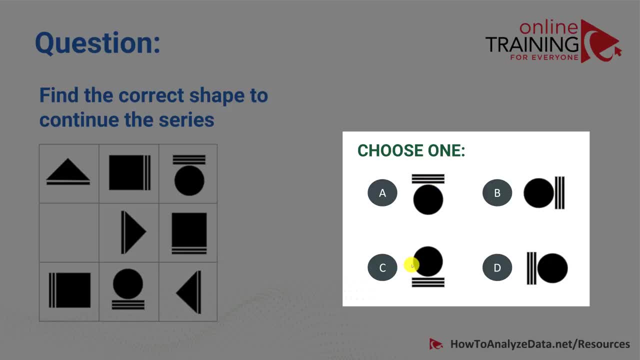 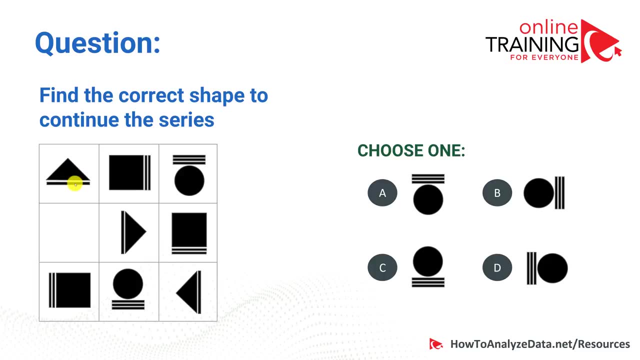 location on the top, right, left and bottom. so how would you know where's the right location for the circle shape? so let's look closely here and let's detect the pattern here for the line location. the line location starts with the bottom, right and then top. so you see it's going. 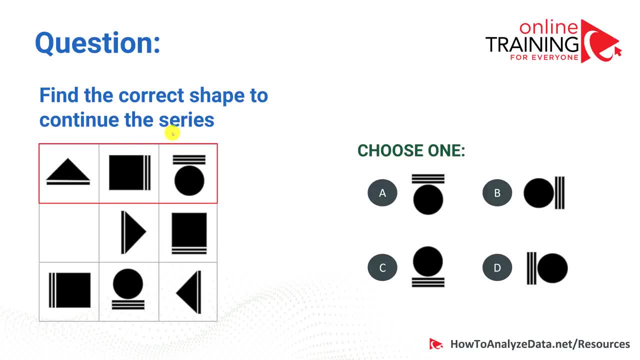 counterclockwise. so if, if you imagine the clock with the clockwise rotation, then this would be counterclockwise. and let's see if we are correct and we have a pattern here, so we have bottom, right, top, then we have left bottom, so that still matches the counterclockwise pattern, and then we have left. 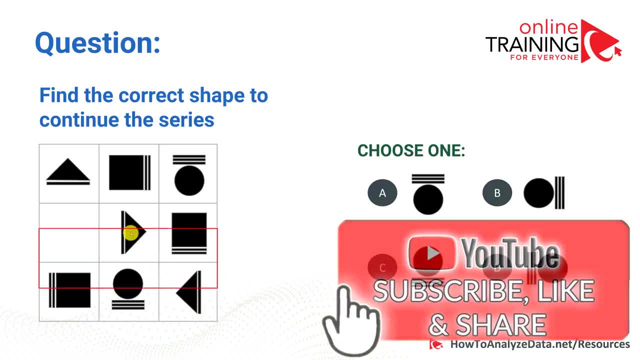 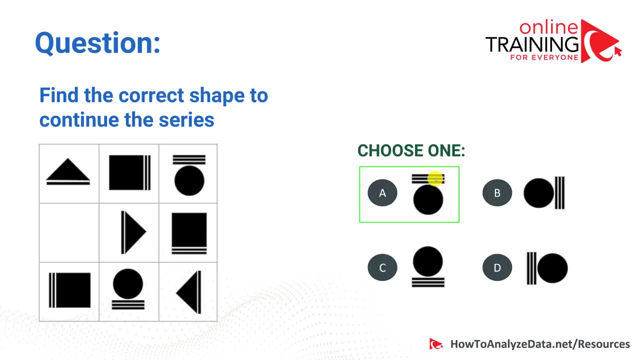 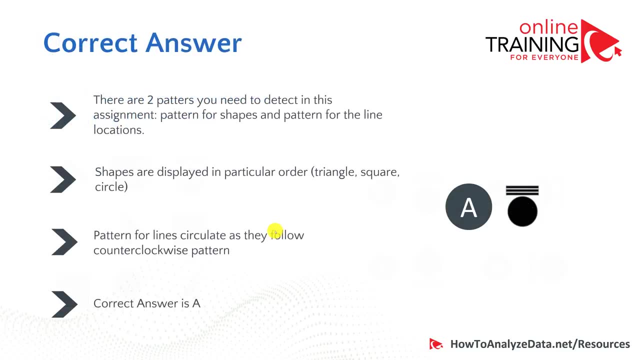 bottom right. so i think the missing shape here would be the one before the left, which would be the right answer. in this case would be a, because here we have a circle which matches the circles pattern and then we have lines located at the top. let's verify to confirm that and, as you can see, 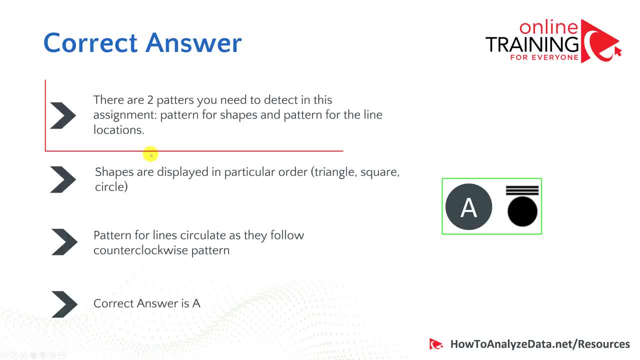 the correct answer is a. so let's recap. there are two patterns you need to detect in this assignment: patterns for the shapes and pattern for the line. location. shapes are displayed in a particular order: triangle, square circle. that's really the pattern for the shapes and patterned for lines. 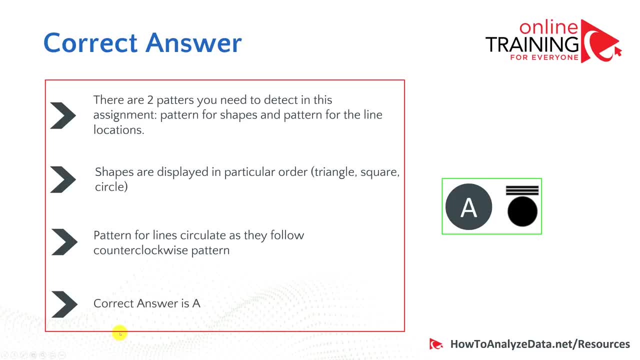 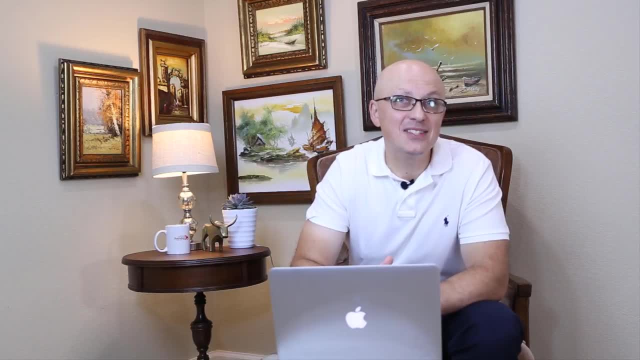 are in the counterclockwise order, so correct answer: A. Hopefully you've got this one right. You will see a lot of these types of questions in the assessment test. In addition to showing you questions and answers from the real test, I also have questions for you to answer. Most of the 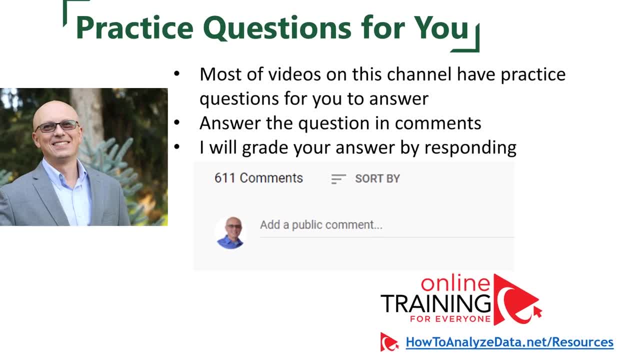 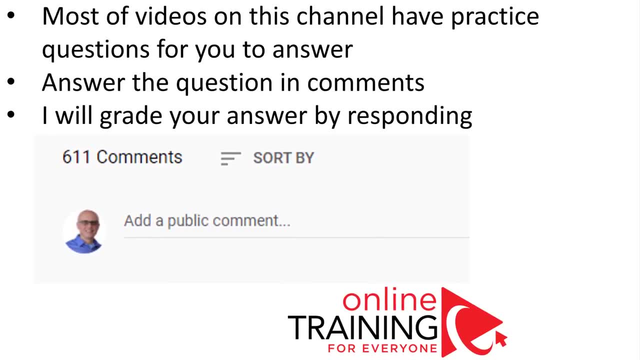 videos on this channel have practice questions for you to answer. Please make sure to post your answers in the comment section of the video. This will allow me to validate your answer and give you the grade. Now let's continue and get you ready for the assessment test. 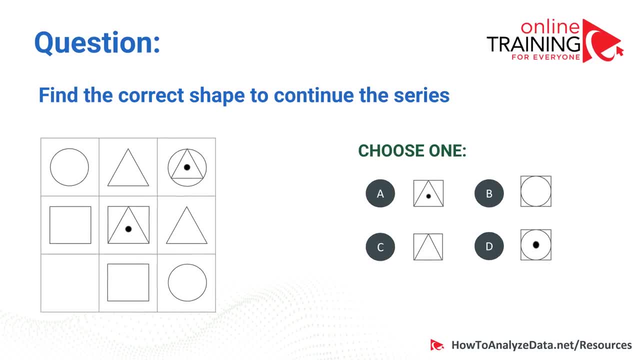 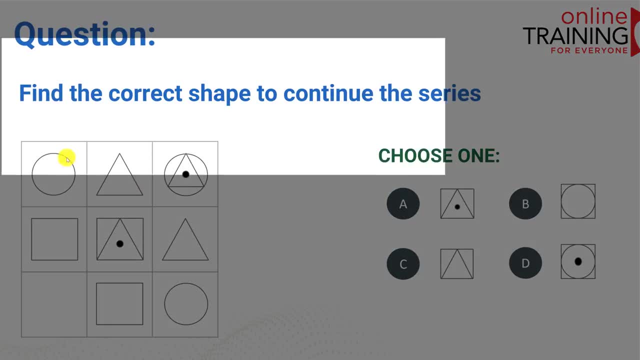 Let's look at the question which is frequently used as part of numeric reasoning test and aptitude test. Find the correct shape to continue the series and you're presented with the three by three box, which contains multiple shapes, and one shape is missing in one of the 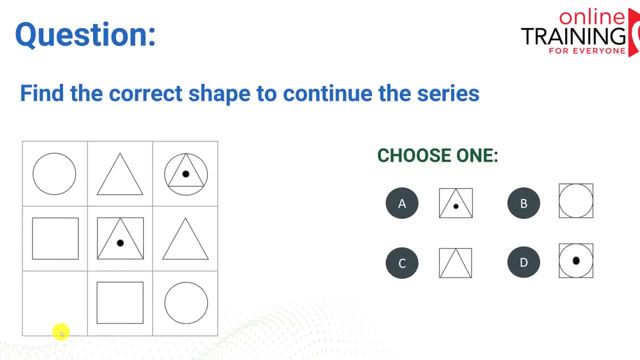 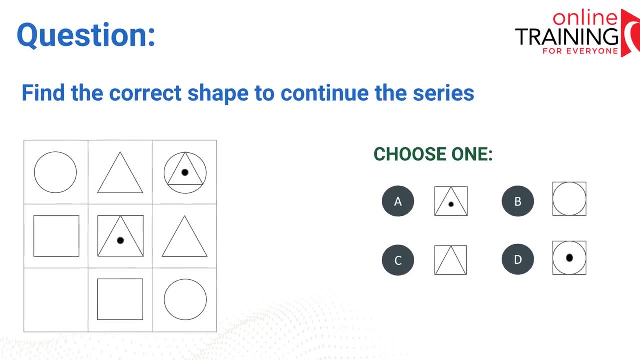 boxes. There are four choices. Can you detect which one is the correct one? Before I jump to the final answer, let me teach you how to detect patterns in these types of questions. There are three different patterns that we can see here. First pattern is pattern in the shapes We have, circle and triangle in. 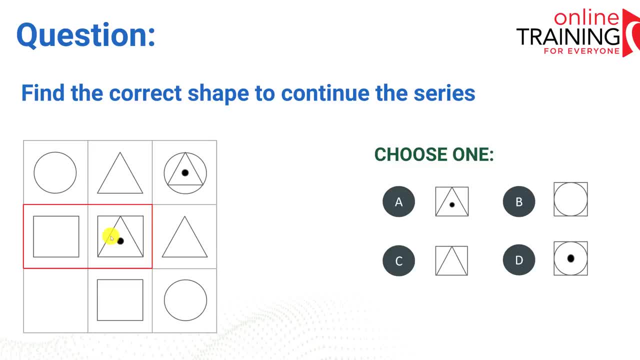 the first row, We have square and triangle in the second row, And then we have square and circle in the third row. The second pattern here is the pattern of one shape inside of the other. So what you see here is that every row contains: 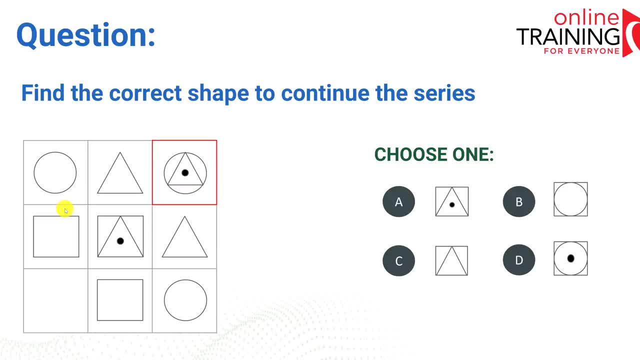 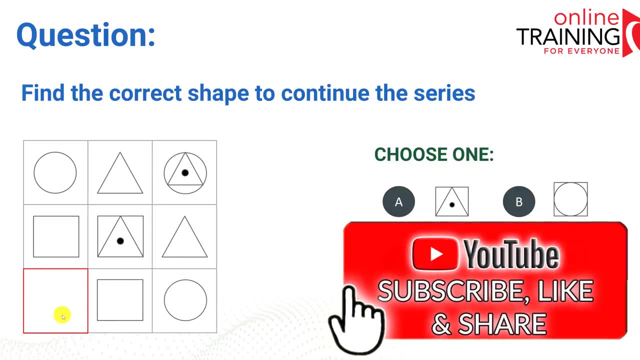 one shape inside of the other. In the first row, it's a triangle inside of the circle. In the second row, it's the triangle inside of the square, And the third one is missing. this pattern Which tells us that it should be the pattern of one shape inside of the other. 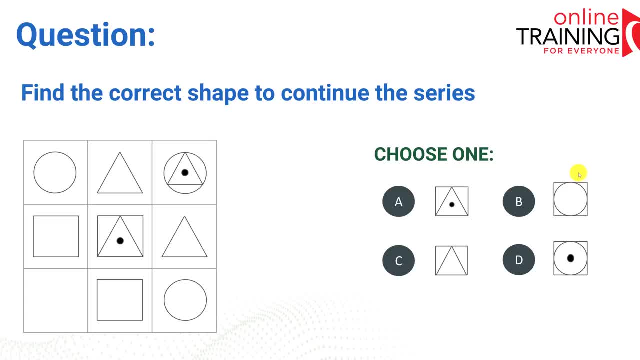 Which is not a big help, because all of the four choices here do contain the shapes, one shape inside of the other. But let's keep that comment and let's just jump to the third pattern. And the third pattern is the dot in the middle of the shape. So you see. 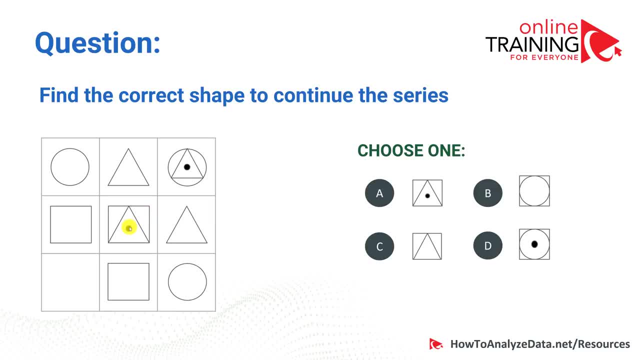 that every row contains at least one shape where a dot is inside of the shapes that are one inside of the other. So, knowing this information, we have a choice: A and D, because we narrowed it down and recognized that we have to have a dot inside of the shape. Now, which one do you think is right? Knowing the first, 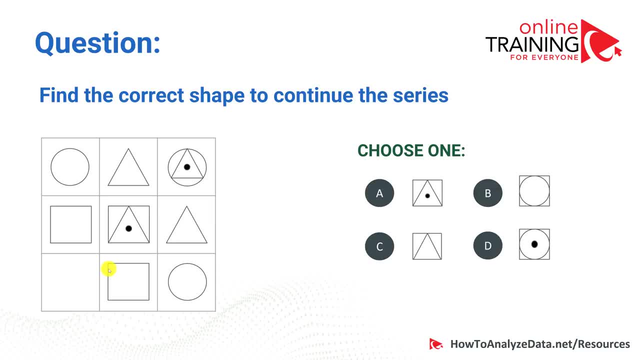 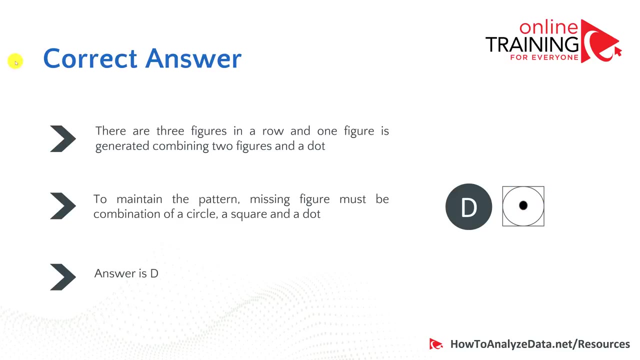 pattern. we can exclude choice A because in the third row we have a combination of squares and circles, So the correct choice is D, because it matches all three patterns. We have a circle inside of the square and then we have a dot in the middle, So the correct answer is D. Hopefully you've got this one right. 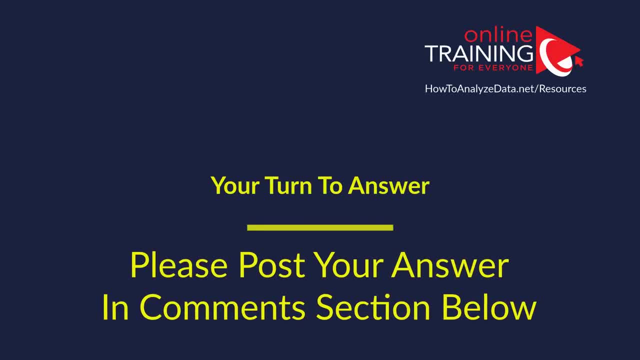 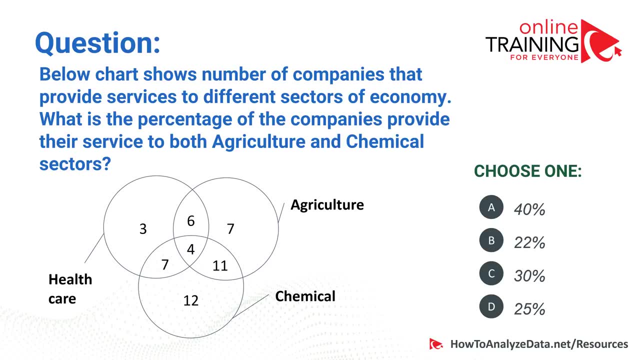 And it's your turn. Please make sure to post your answer in the comment section below this video so I can give you the grade. Here's the question for you to answer. Below chart shows the number of companies that provide services to different sectors of the economy. What is the percentage? 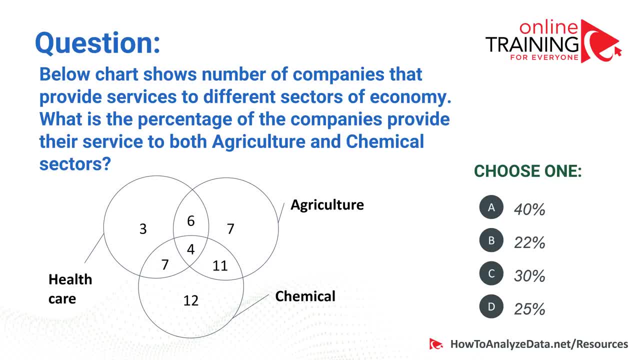 of the companies that provide their services to both agriculture and chemical sectors, And you have four choices here: 40%, 22%, 30% and 25%. Please make sure to post your answer in the comment below this video so I can give you the grade. 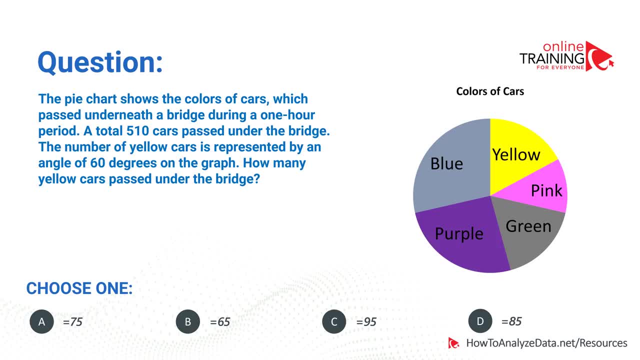 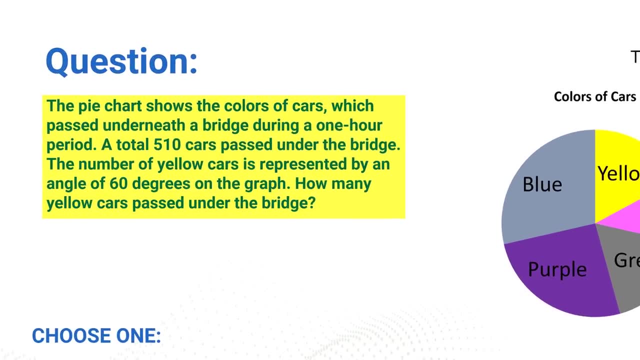 Now let's look at the question which frequently used as part of logical reasoning tests. It tests your knowledge of math, abstract reasoning and numerical reasoning. The pie chart shows the colors of cars which passed underneath of the bridge during the one hour period. 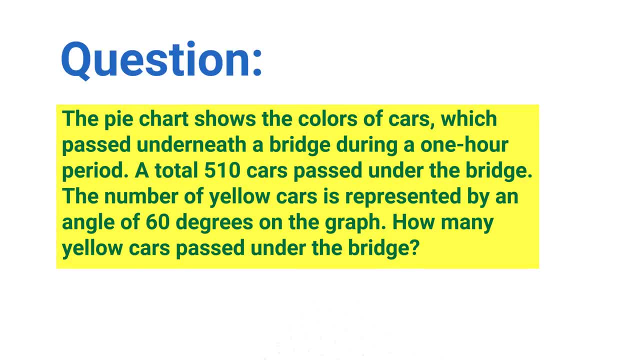 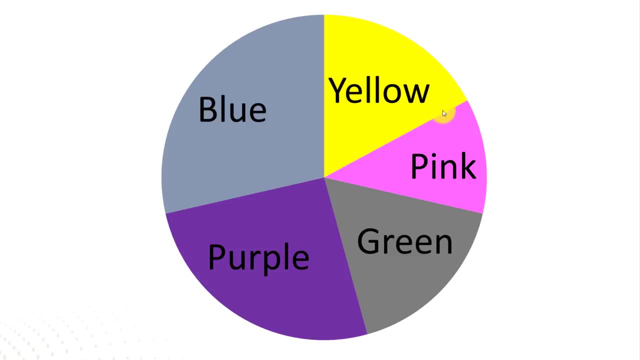 A total of 510 cars passed under the bridge. The number of yellow cars is represented by an angle of 60 degrees on the graph: How many yellow cars passed under the bridge. You're presented with the graph which shows yellow segment, which we know is 60 degrees. 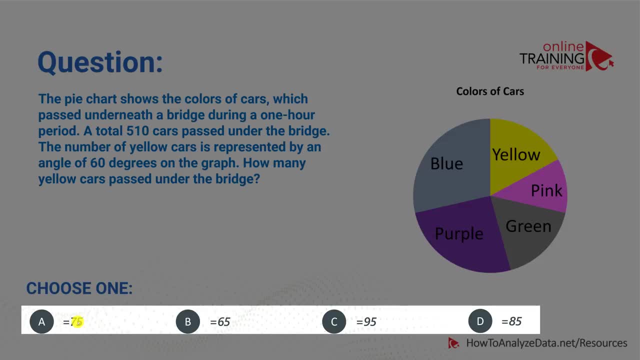 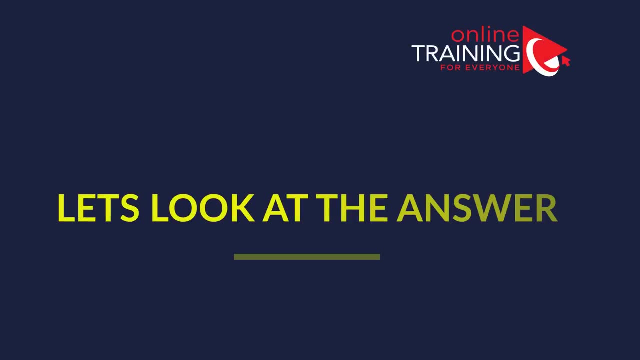 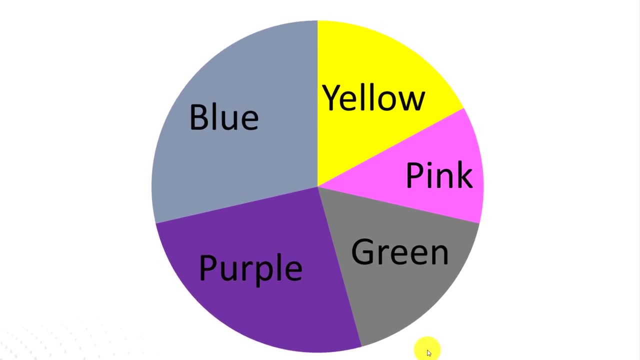 And there are four choices: 75 cars, 65 cars, 95 cars or 85 cars. What do you think is the correct answer here? To answer this question correctly, you need to understand the ratio between the entire circle which has 360 degrees, and yellow portion of it. 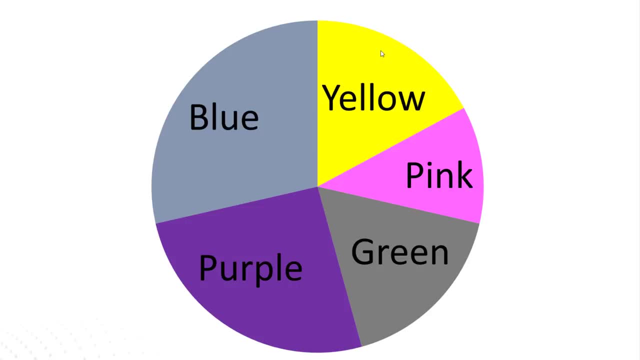 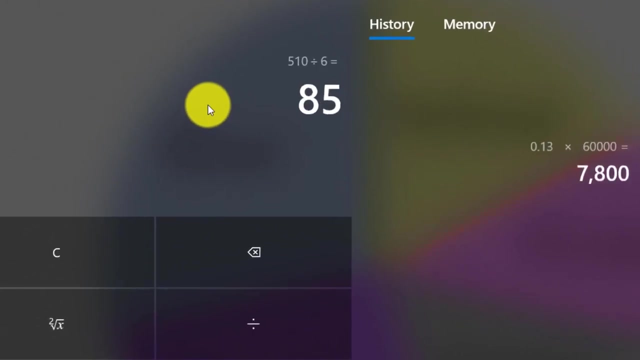 which represents the cars passed underneath of the bridge in one hour period. Because 60 is one sixth of 360, it means that one sixth of 510 cars passed under the bridge. We need to divide 510 by six. 500 divided by six is 85.. 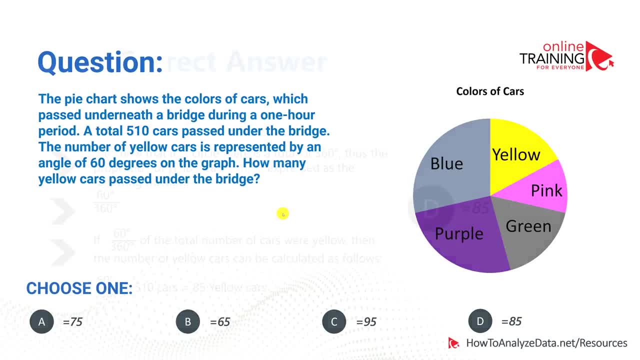 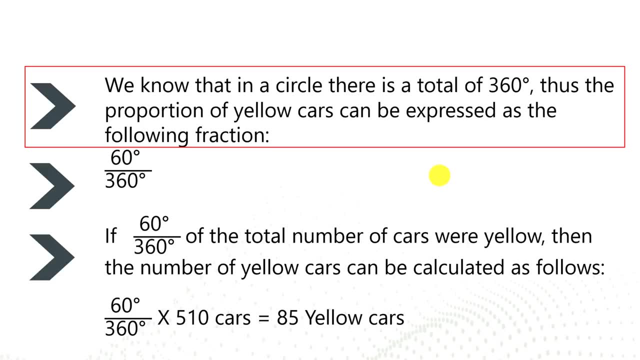 So the correct answer here is D, which is 85.. Let's recap: We know that in the circle is the total of 360 degrees and proportion of yellow cars can be expressed as one sixth of 360. When we divide 510 by six, we get 85.. 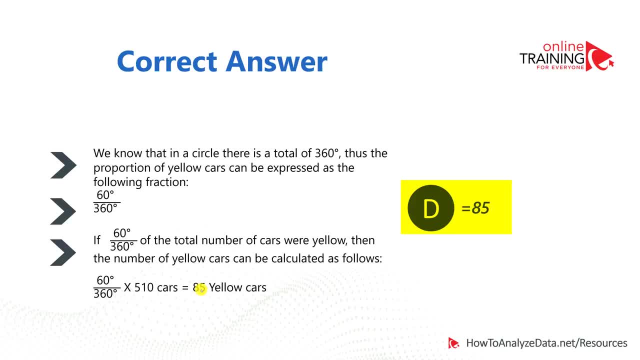 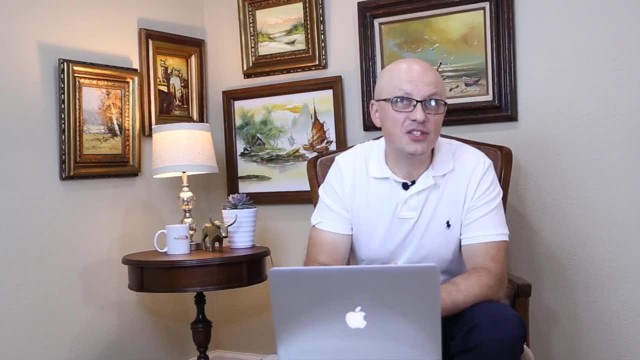 And 85 is the number of yellow cars passed under the bridge during one hour period. I'm pretty sure you've got this one correctly. Please make sure to check out the available downloads in the description section of this video. All links to the downloads are available. 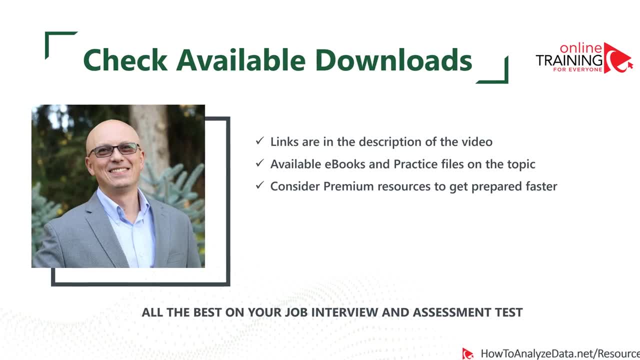 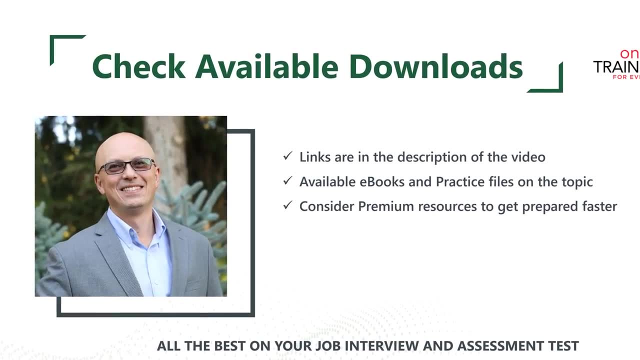 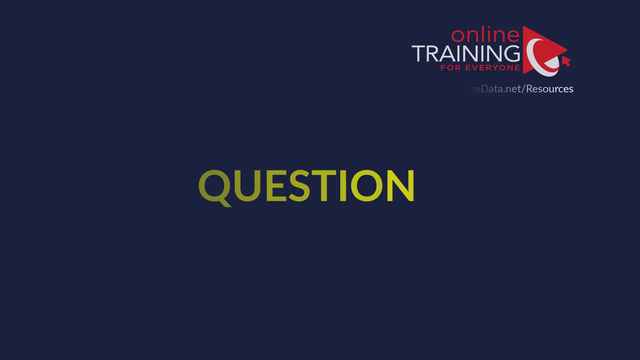 in the description of this video. Please make sure to consider eBooks and practice files, and also consider premium resources that helped other people to get prepared faster. Now let's continue and get you ready for the assessment test. Now let's review assessment test question. 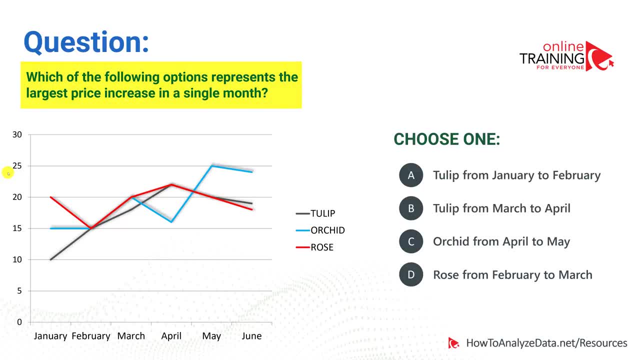 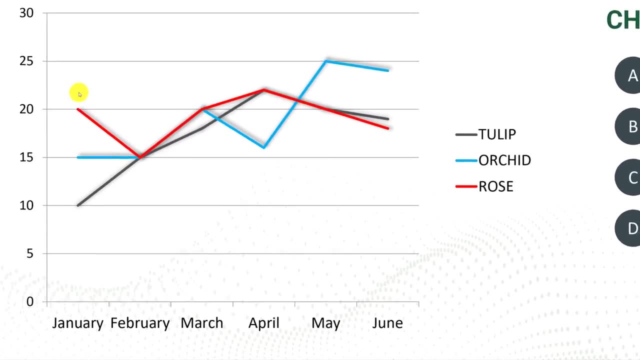 which tests your knowledge of charts and graphs. Which of the following options represent the largest price increase in a single month? You're presented with the graph, which contains three different lines, One for each of the three lines: One for tulips, another one for orchids. 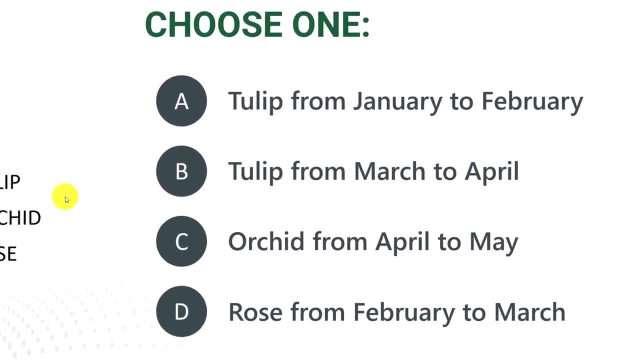 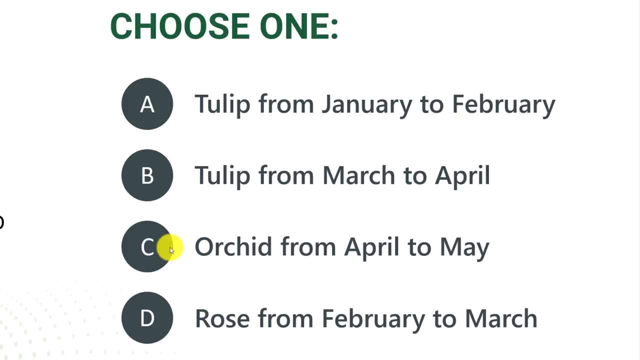 and the third one is for roses. You have four choices: Tulips from January to February, Choice B tulip from March to April, Choice C- orchid from April to May And choice D roses from February to March. Which one do you think is the correct answer? 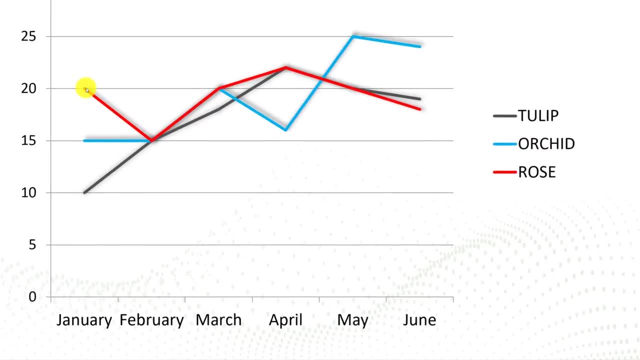 To answer this question correctly, you need to look at the segments of this graph. Segment that goes from months to months represents either price increase or price decrease. The largest segment that represents one single month's largest price increase would be on the blue line from April to May. 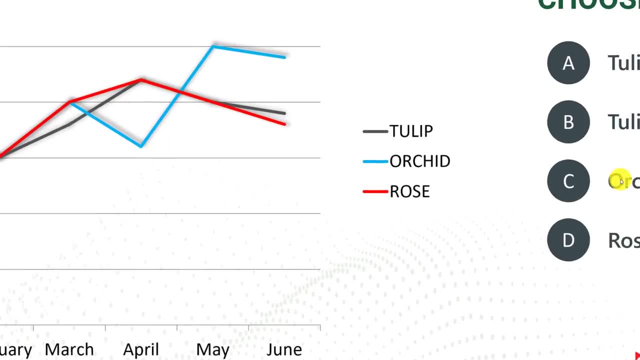 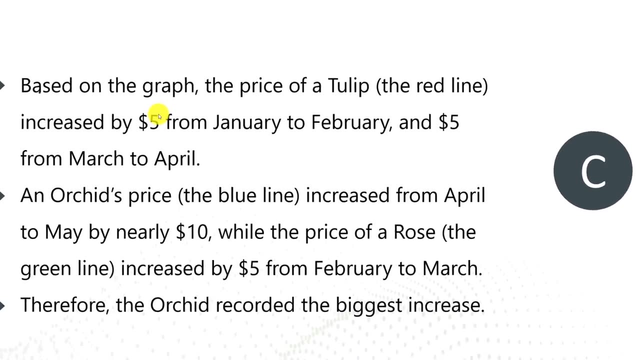 Blue line represents orchids And let's go to the choice. So the right answer here is choice C: orchids from April to May, Based on the graph shown, there are different price increases here. Price of the tulip, for example. 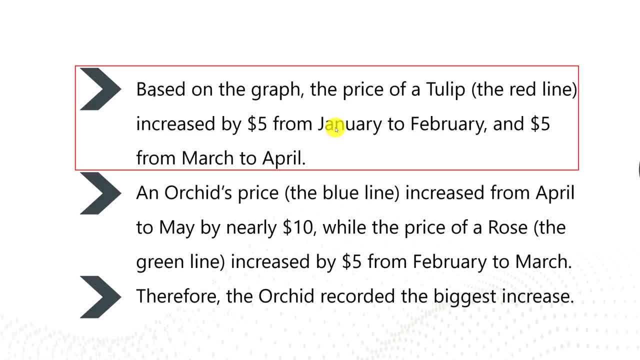 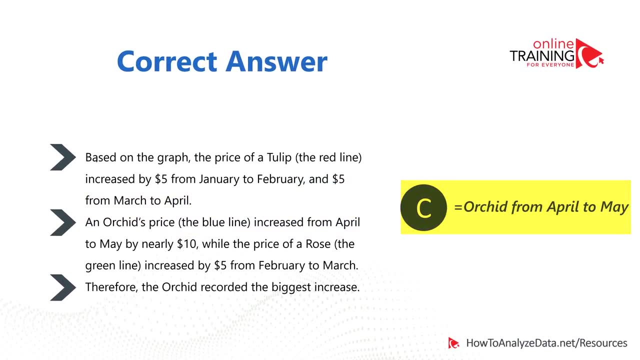 increased by about $5 from January to February and another $5 from March to April. But orchid's price, which represented by blue line, increased from April to May by nearly $10,, which represents the largest price increase. I'm pretty sure you nailed this question. 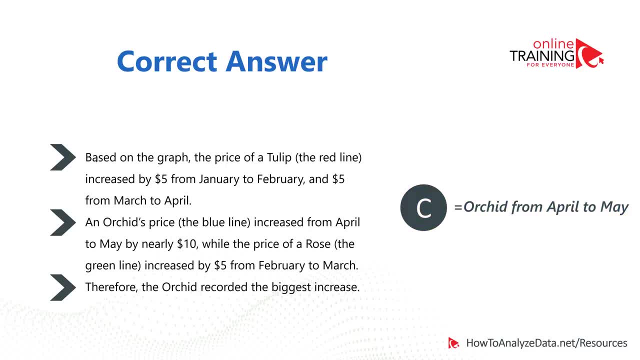 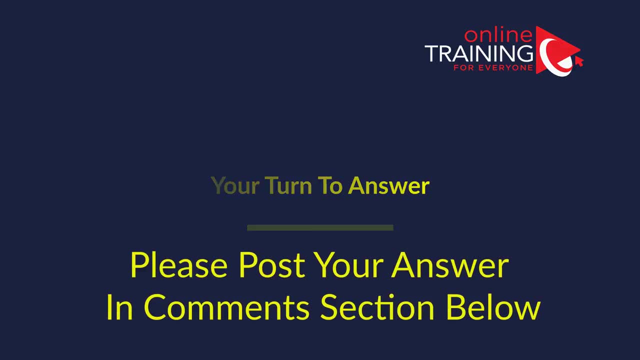 This was rather easy, but you see a lot of these types of questions in assessment tests, And now it's your turn. Please make sure to post your answer in the comment section below this video so I can give you the grade. Here is the question for you to answer. 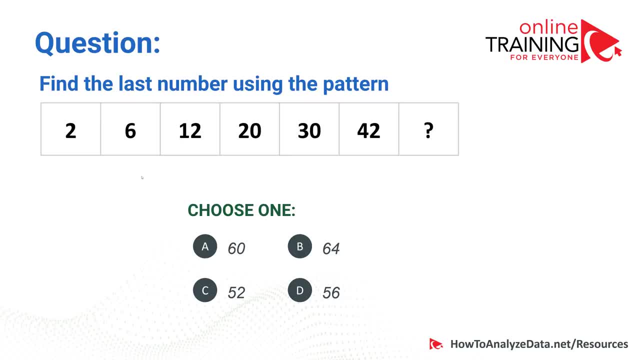 You need to find the last number using the pattern: 2, 6,, 12,, 20,, 30,, 42,, and then the missing number, And the choices are 60,, 64,, 52, or 56.. 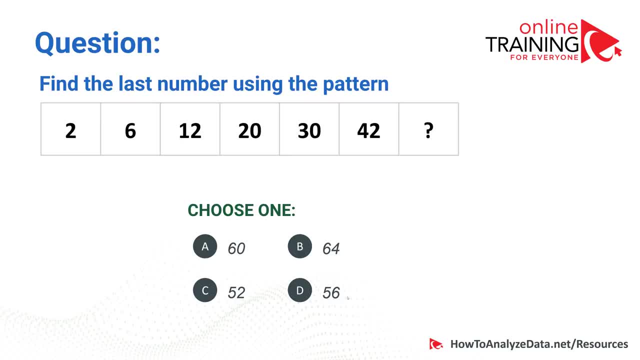 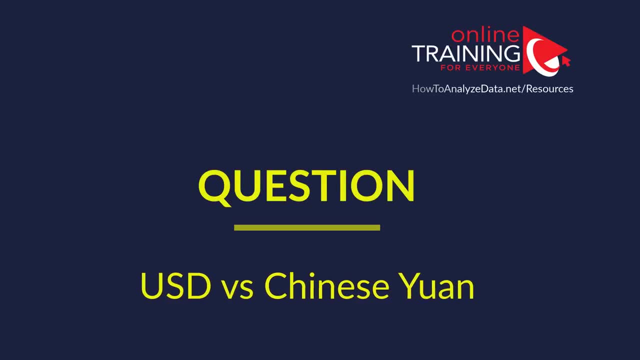 Which one do you think is the right answer here? Please make sure to post your answer in the comment section below this video, so I can give you the grade. And now let's look at the answer to the question, which is very frequently used as part of aptitude tests. 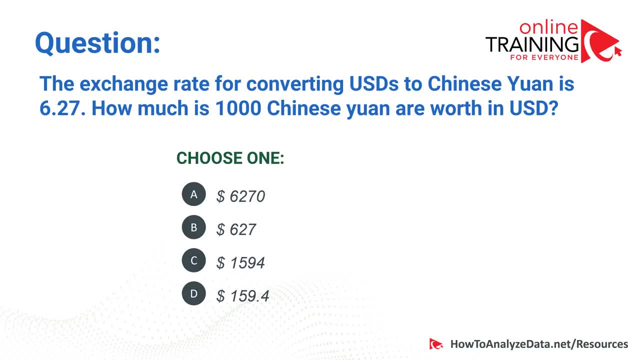 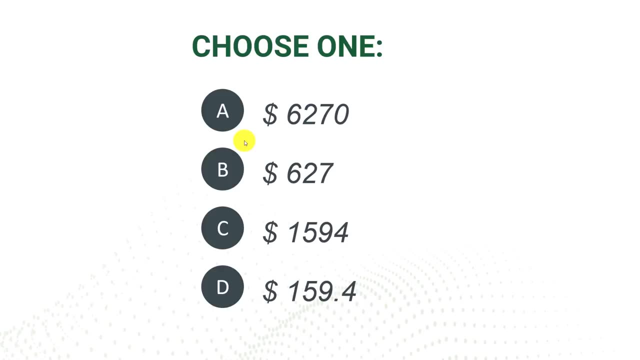 math reasoning, abstract reasoning and logical reasoning tests. The exchange rate for converting US dollars to Chinese yans is 6.27.. How much is 1,000 Chinese yans are worth in US dollars? And you have four choices: 6,270,, 627,, 1,594, or $159.40. 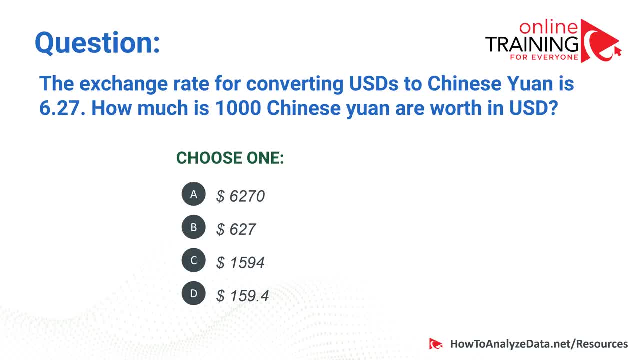 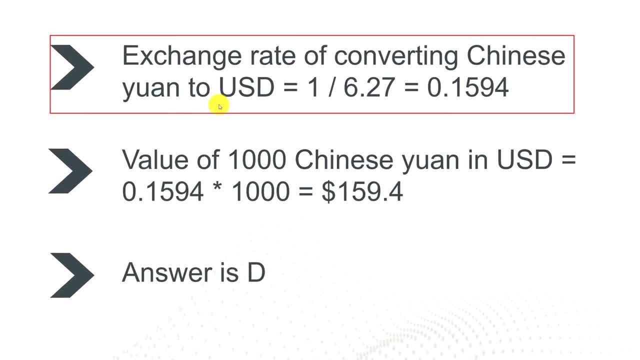 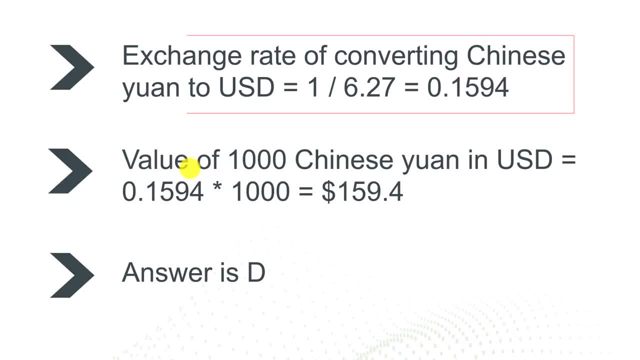 which is an equivalent of 0.1594,, which means that the value of 1,000 of Chinese yans in US dollars is an equivalent of 0.1594 multiplied by 1000, which is $159.40.. 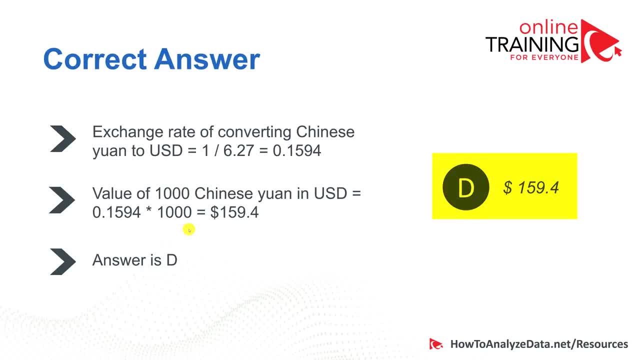 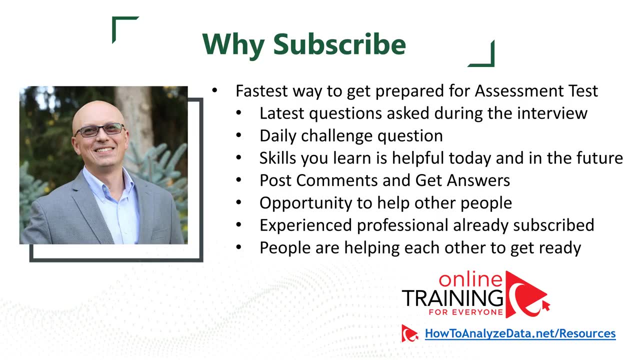 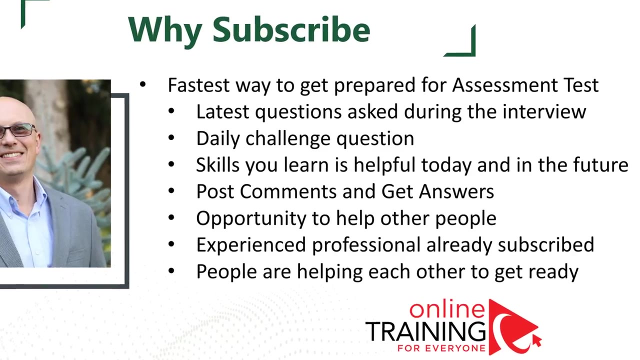 So the correct choice is D. Hopefully your selection for this answer was correct. Let me give you a couple reasons why you might consider subscribing to online training for everyone. Knowing latest assessment test questions and answers helps you to get ready for the interview and assessment test and improves your job mobility. We share with you latest questions. 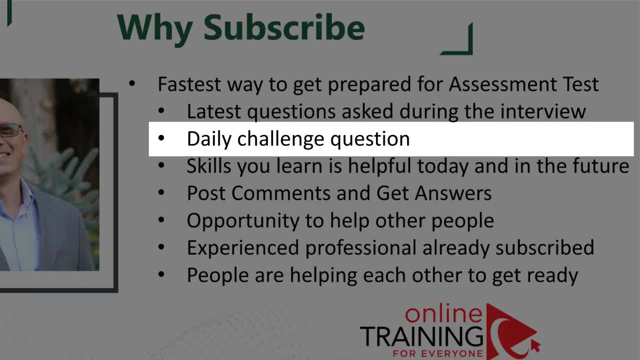 asked during the interview. You get access to the daily challenge question. You see questions and answers people posting in the comment section of this video and you get access to other people's experiences. You also have opportunity to help other people by answering their questions. We have 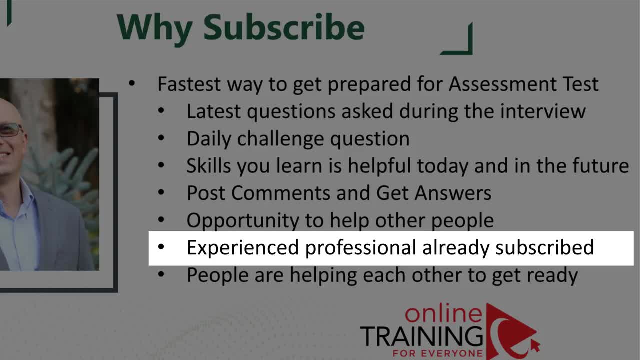 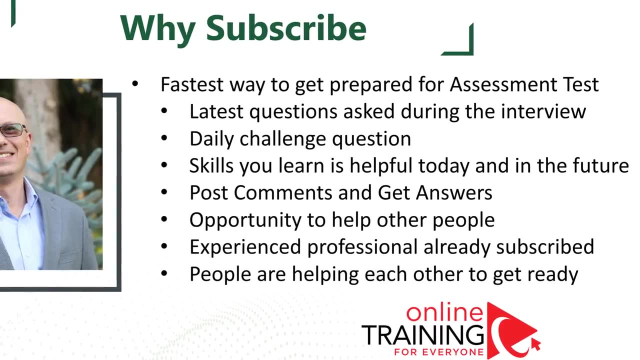 a community of great people already subscribed to this channel, and these people are here ready to help you with the challenges you are experiencing. Subscribing to online training for everyone is an exciting opportunity to get ahead in your career. Thank you for your time and consideration, and 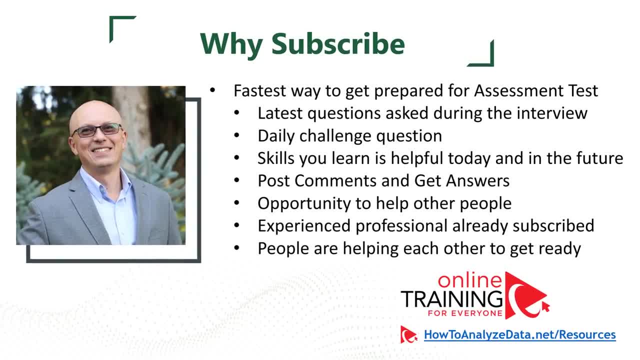 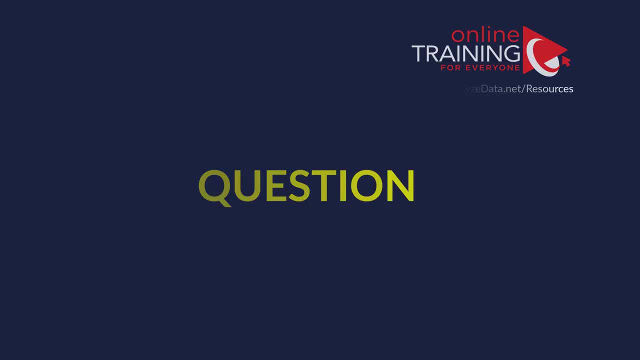 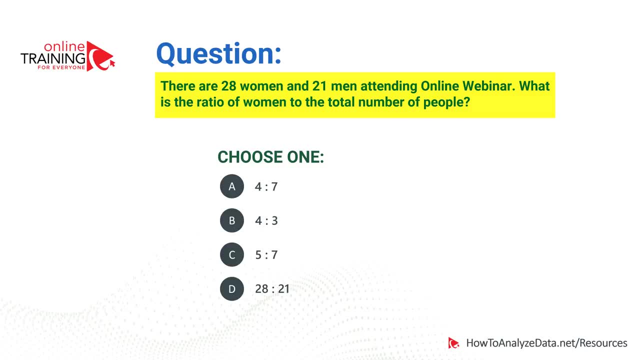 looking forward to have you as a member on this channel. Now let's continue and get you ready for the assessment test. Now let's look at the tricky question which is frequently used as part of math reasoning and abstract reasoning tests: There are 28 women and 21 men attending online webinar. What is the ratio? 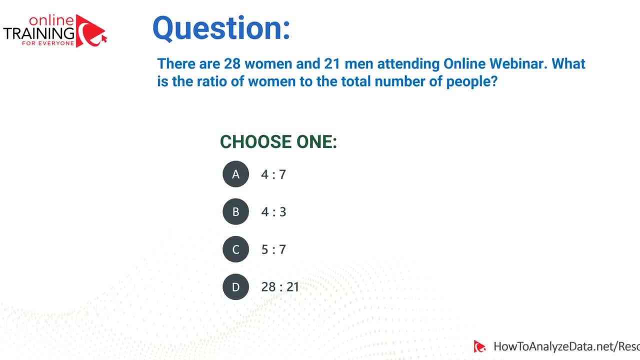 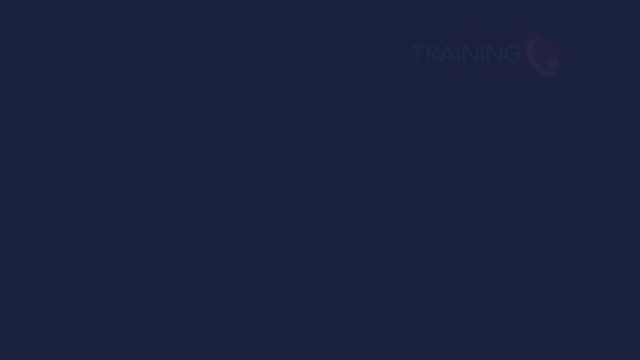 of women to the total number of people, And there are four choices: 4 to 7,, 4 to 3,, 5 to 7, and 28 to 21.. Which one do you think is the right answer? The tricky part about this question is that there 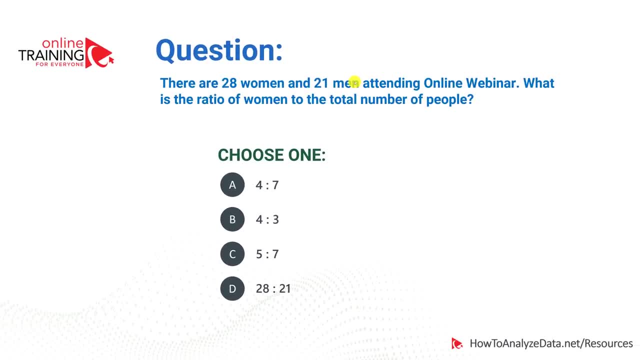 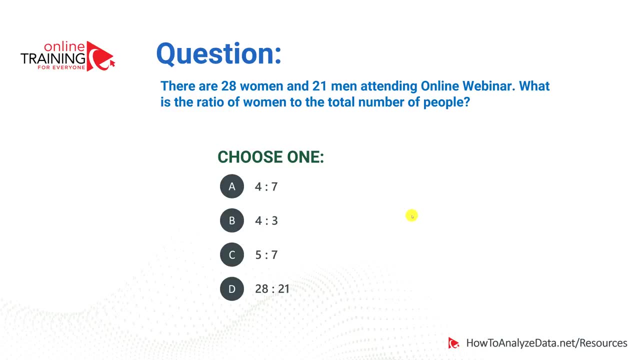 are choices B and D, which represent the ratio of women to men. But this is not what needs to be calculated here, because ratio of women to total number of people need to be captured. Let's look at the correct answer: Total ratio of women to men is 4 to 3. 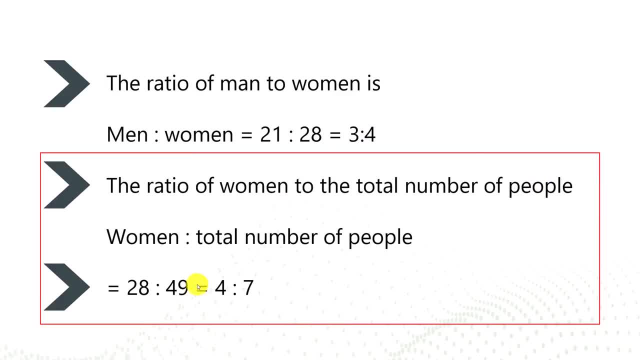 but the ratio of women to total number of people is 4 to 7, which represented by 28 to 49, and 49 is calculated as the sum of all people: 28 women and 21 men. So the correct answer is A 4 to 7.. I'm 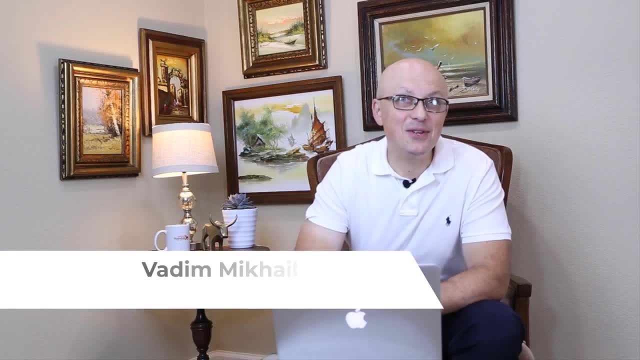 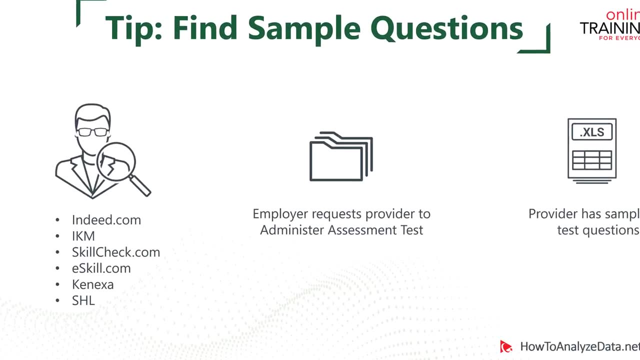 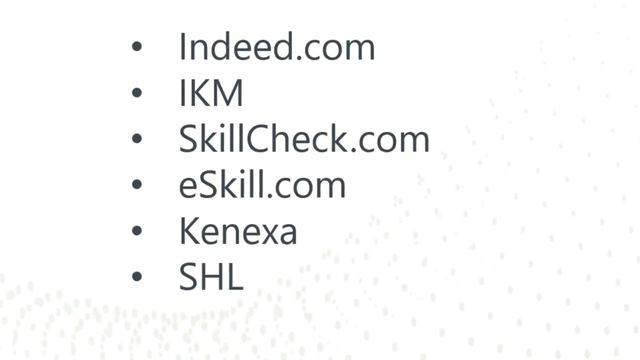 pretty sure you nailed this question. I would like to give you a tip. There are a lot of different providers that conduct employment assessment tests. Most common providers that do assessment tests today are Indeedcom, IKM, Skillcheck, eSkills, Connexa, SHL and a lot of others. Employer: 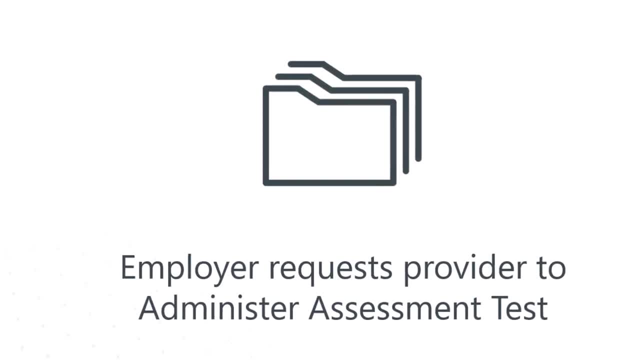 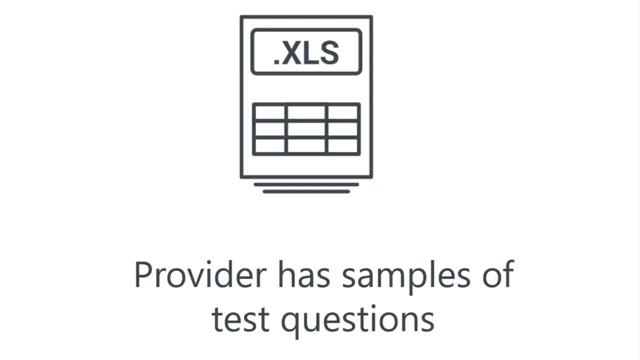 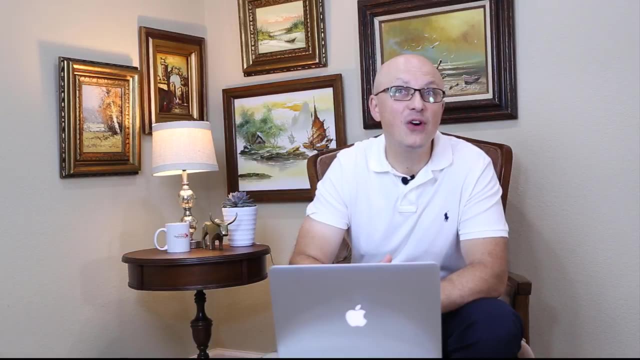 typically requests provider to administer assessment tests, and then provider contacts the candidates to conduct the test. A lot of times, provider has a sample test questions on their website. Once you know which provider will be assessing your skills, it's a good idea to visit their website to find sample questions. 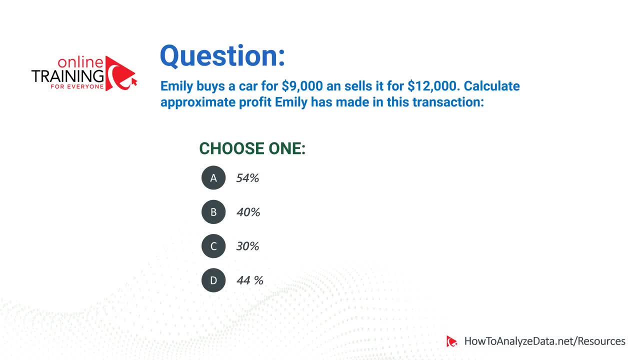 Let's look at assessment test question which is frequently used as part of abstract reasoning, numerical reasoning and logical reasoning tests. Emily buys a car for $9,000 and sells it for $12,000.. Calculate approximate profit Emily has made in this transaction. 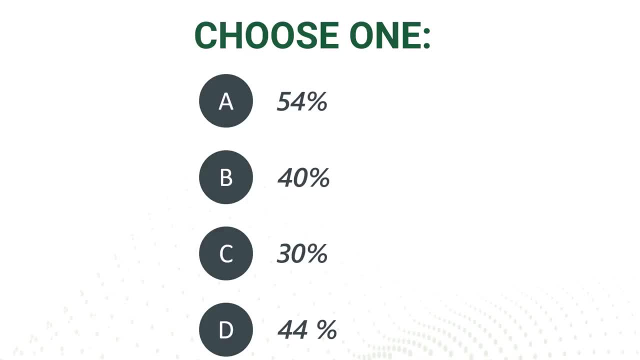 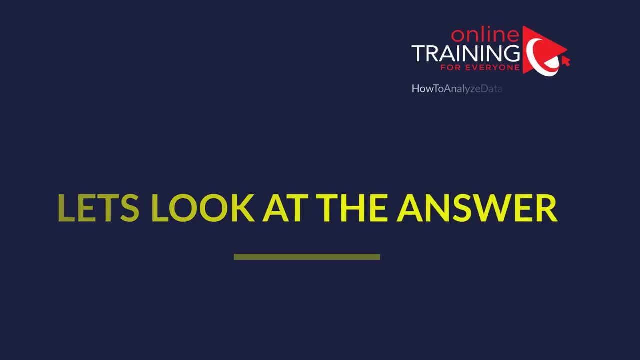 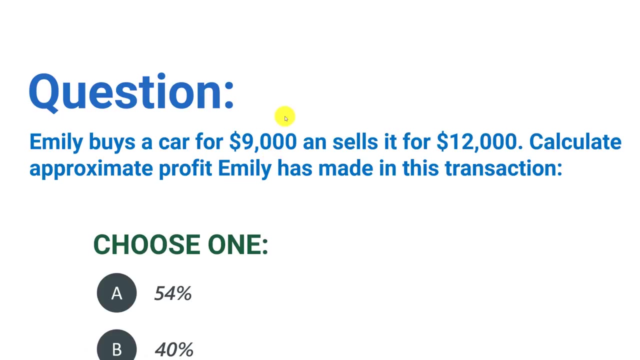 dans le choix: E 40 %, B, 30 %, D, 44 %. Which one do you think is the right answer? First, to answer the question here, you need to calculate the actual profit, And the profit is $12,000 minus $9,000, which is equal to $3,000.. Then you need to calculate the profit. 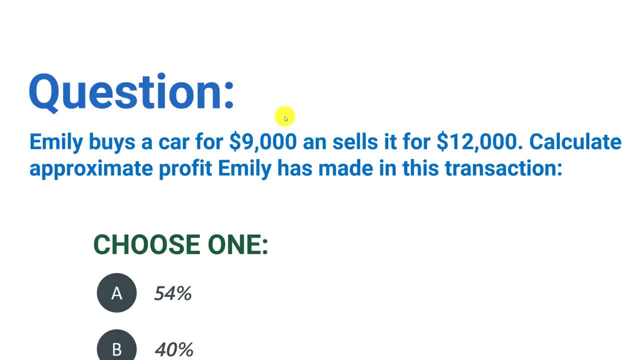 percentage which is calculated by $3,000 divided by $9,000, because $9,000 is the most recent profit in this transaction. If you calculate the total profit per percentage, well, it's $3,000, some people say it's $9,000.. If you calculate the profit per percentage, you should. 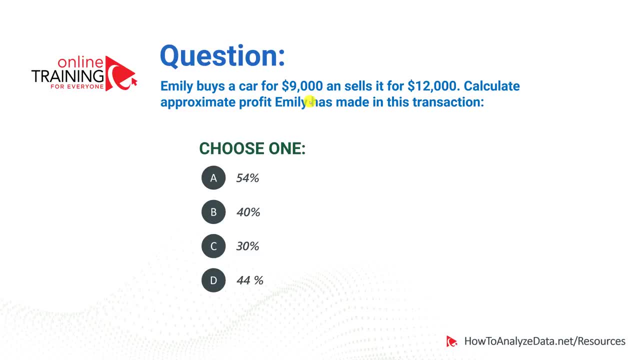 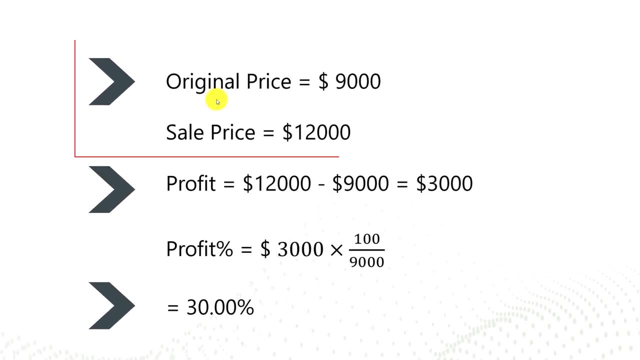 the original price and the value here that you will get would be 30 percent. so choice c is correct. let's recap: original price for the vehicle was nine thousand dollars, sale price was twelve thousand, profit is three thousand and is calculated as twelve thousand minus nine thousand. 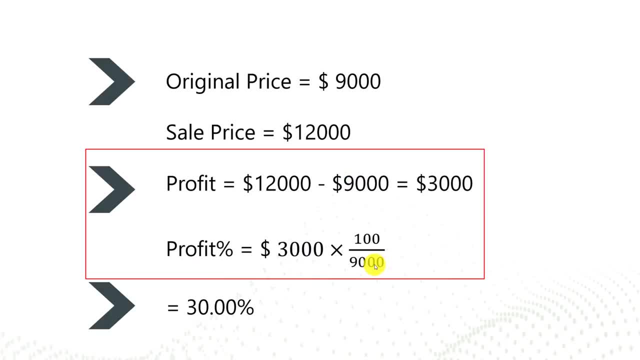 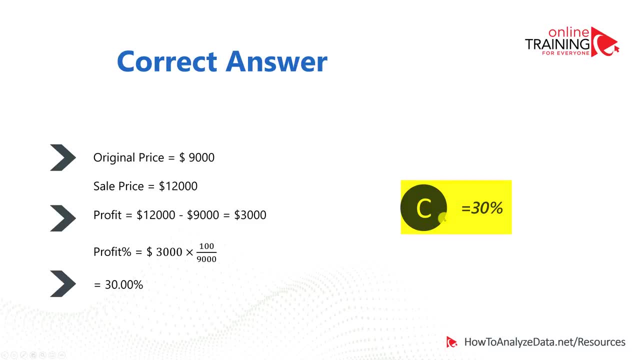 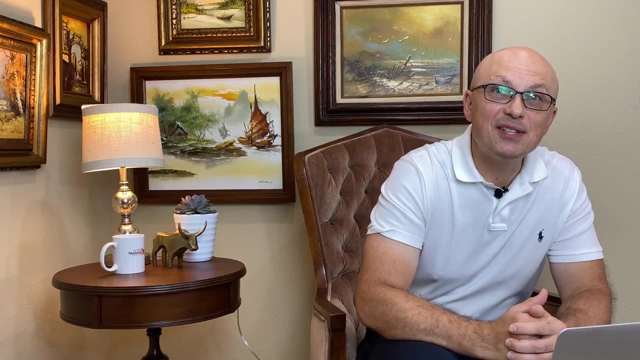 the profit is calculated as three thousand divided by nine thousand and multiplied by hundred and is equivalent of thirty percent. so choice c is correct. did you get this one right? please share in the description of this video. if you got this one correctly, let me share you smart ways to get prepared for the test. one of the smartest way: 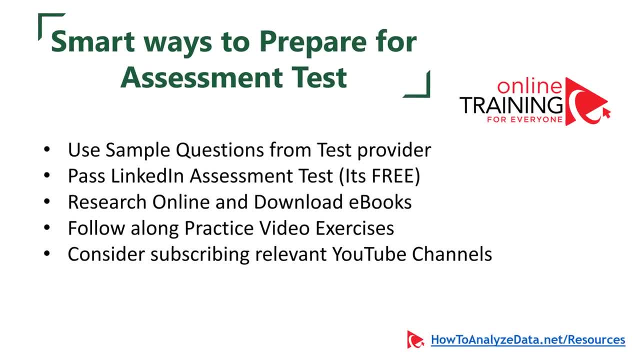 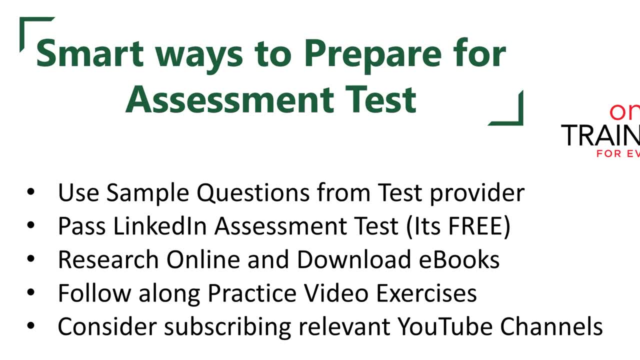 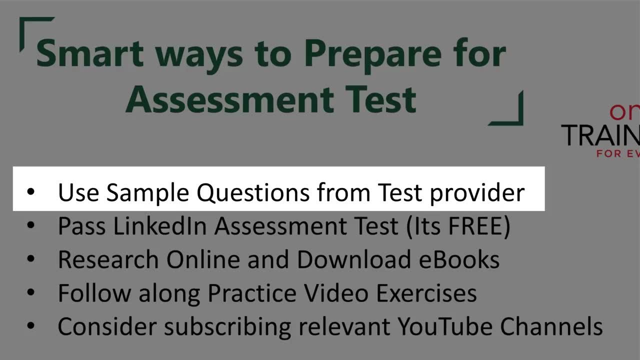 to prepare is to find out who your provider is. that will be conducting an assessment test and use outlines and sample questions from the provider. the providers might be indeedcom skill check, ikm, kinexa, shl and a lot of others. once you know who the provider is, you can go. 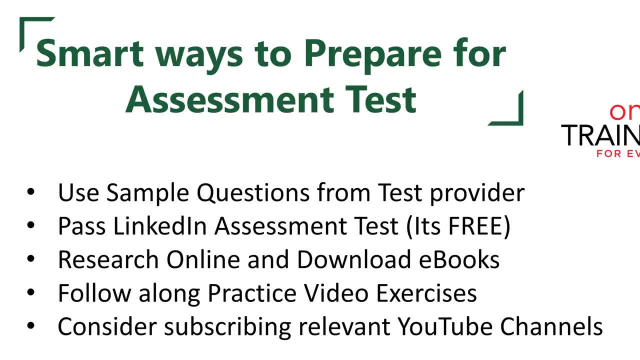 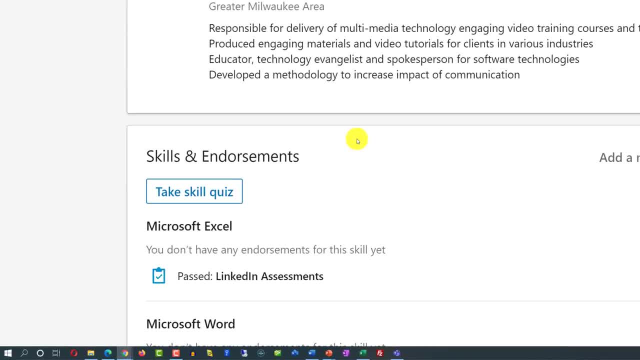 to their website and find out who is the provider. who is the provider for you? the provider will tell. find out sample questions and practice with sample questions. You can also practice LinkedIn assessment test questions on the topic that you will be assessed. LinkedIn test is free. It gives. 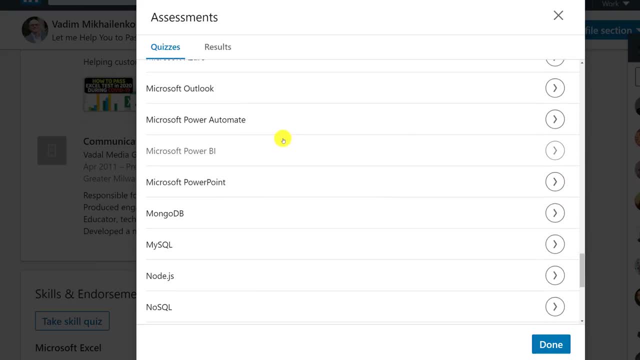 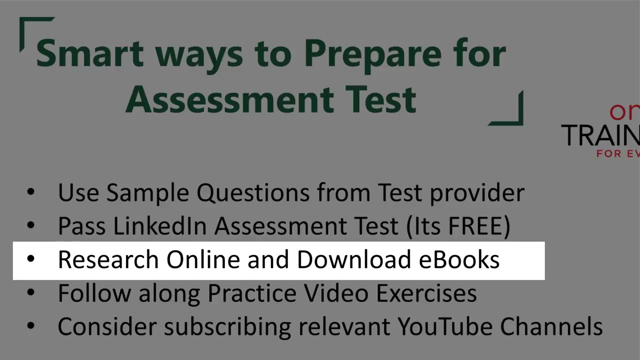 you exposure to the sample questions and also you can get a badge that will enhance your profile for potential employers. You can also research the topic you're trying to prepare for online and download ebooks to get ready for the test. Hands-on experience is very important. You can. 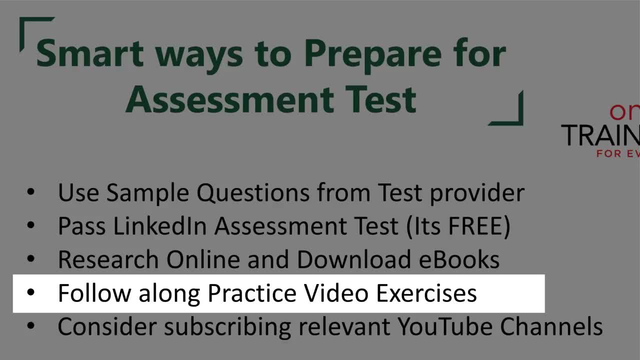 find relevant training and follow along to do hands-on exercises using practice videos on the training. If you have a question or ran into an obstacle during your practice exercises, try posting questions in the comment sections of the video Channel. owners or members of the channel. 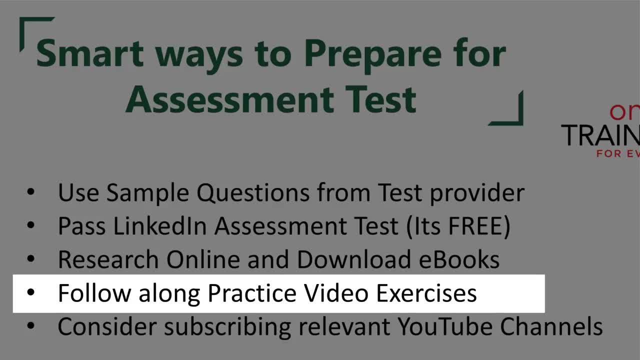 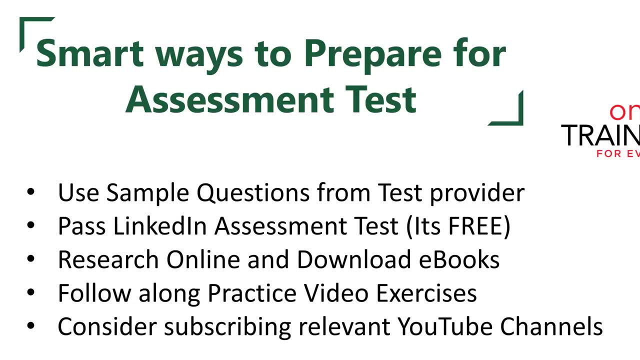 monitor the questions and respond to the inquiries And, last but not least, consider subscribing to the channel. Thank you to relevant YouTube channels. I encourage you to consider subscribing to online training for everyone. We have a great community of people helping each other to prepare and pass the test. 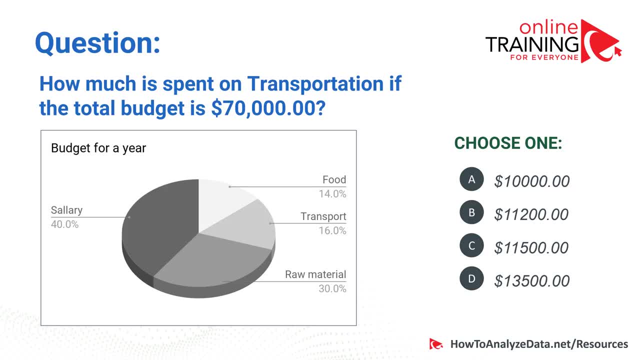 Let's look at the question which is frequently used to test your knowledge of charts and graph and frequently used as part of math reasoning, logical reasoning and also numerical reasoning tests: How much is spent on transportation if the total budget is $70,000?? You have four choices as: 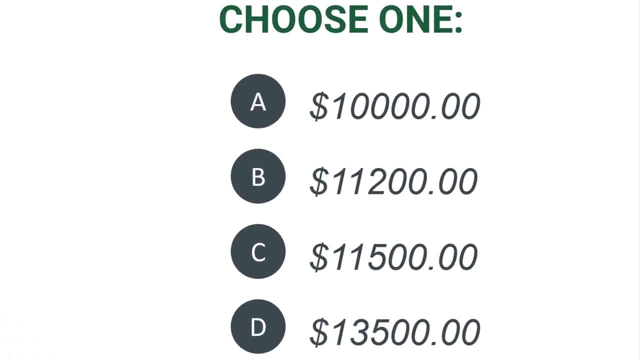 you go. How much is spent on transportation if the total budget is $70,000?? You have four choices as you go. How much is spent on transportation if the total budget is $70,000? You have four choices, as usual: $10,000,, $11,200,, $11,500, and $13,500.. You also present it with the graph on which: 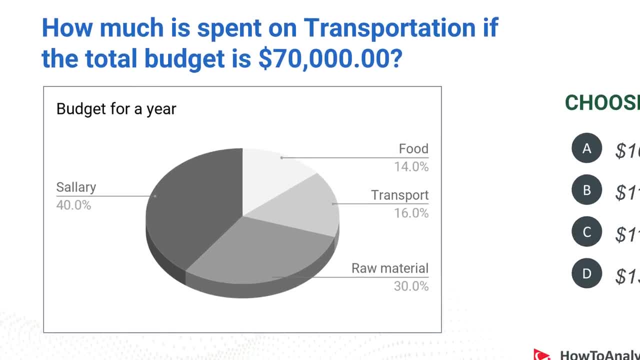 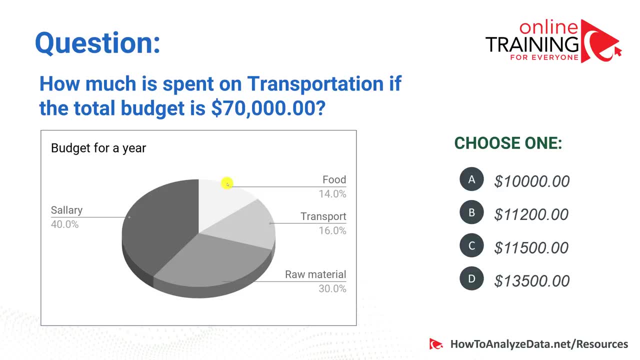 transportation is 16% of the entire budget. Which one do you think is the right choice here? To calculate the transportation budget, you need to get 16% off of $70,000.. Ultimately, you need to multiply $70,000 by 0.16.. So let's look at the answer, Because per 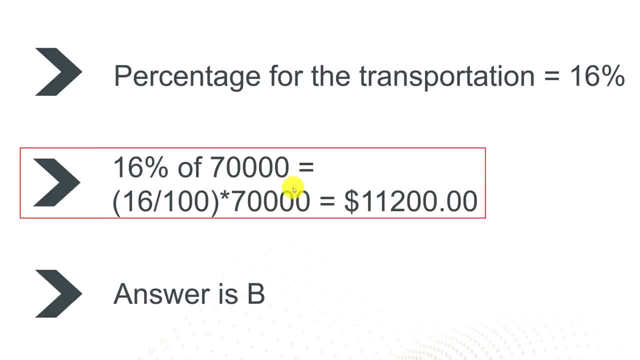 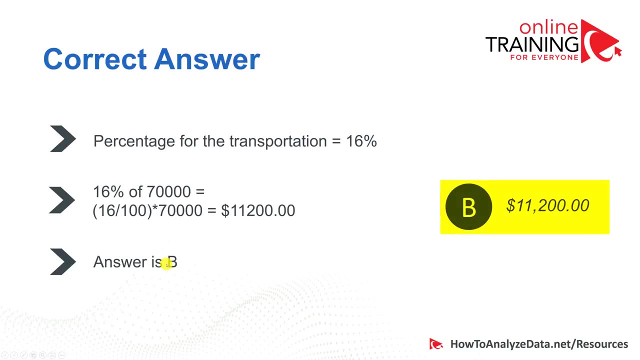 percentage of transportation is 16%, the correct answer is $11,200,, which is calculated as 16 divided by 100, which gets you 0.16 multiplied by $70,000.. So the correct choice is $11,200,, which is choice. 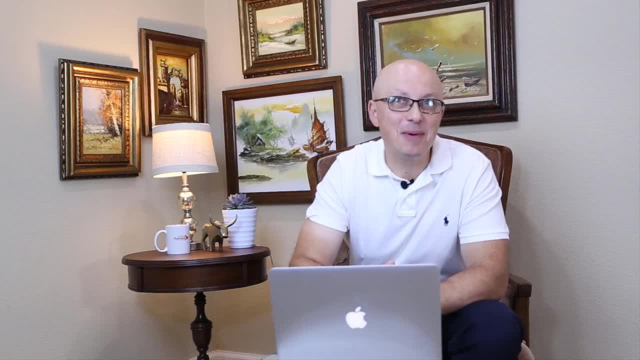 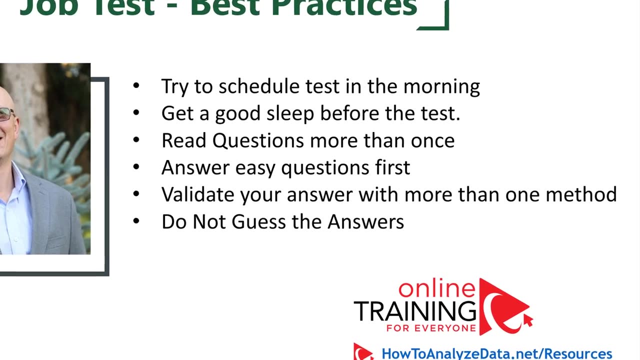 B. Hopefully you've got this one right. Let's talk about best practices on how to get ready for employment assessment test. If this option is available and you have a choice, try to schedule assessment test in the morning. If you have a choice, try to schedule assessment test in the 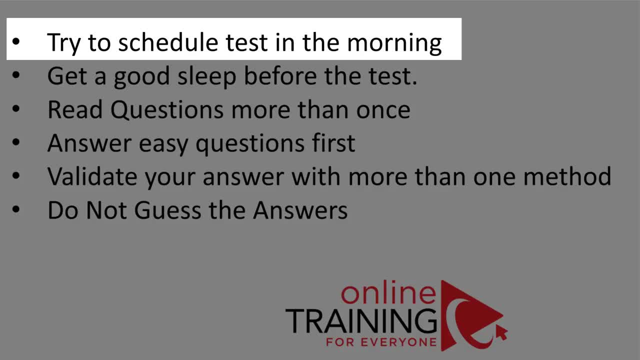 afternoon, when you have highest levels of energy. Get a good night's sleep before the test And please do not take the test if you're tired, since a lot of questions require your top mental energy performance During the test. read each question carefully, ideally more than once. Questions are: 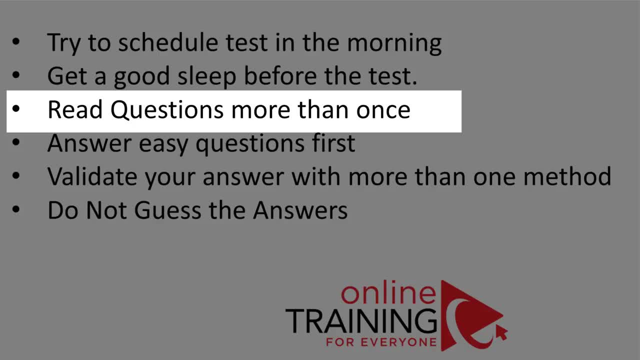 designed to be tricky and each and every detail in the question might be important. If you have a choice, try to answer easy questions first. This would allow you to leave harder questions for the end, but you will get easy answers anyway. If you have a choice, try to answer easy questions. 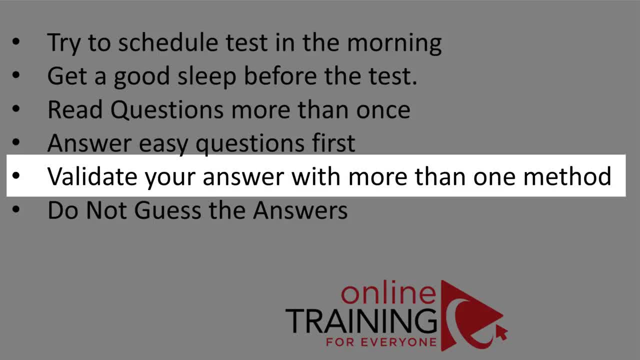 again and you will get the points for them. Try to validate your answers with more than one method. For example, if you are doing an Excel assessment test, you can do manual calculation. you can try to use formulas for calculations, use calculator or use pivot tables to validate your answers. 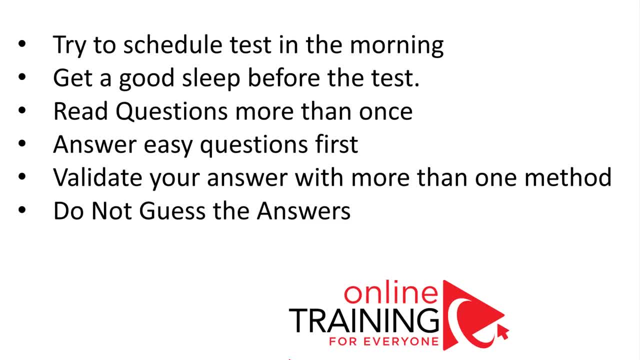 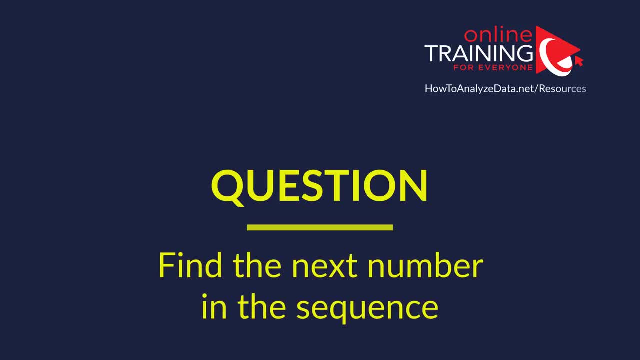 And, last but not least, try not to guess the answers, as some providers deduct points for incorrect selections. So here is the question: what is the best way to get ready for employment in the future, If you have a question which is frequently used as part of numerical reasoning? 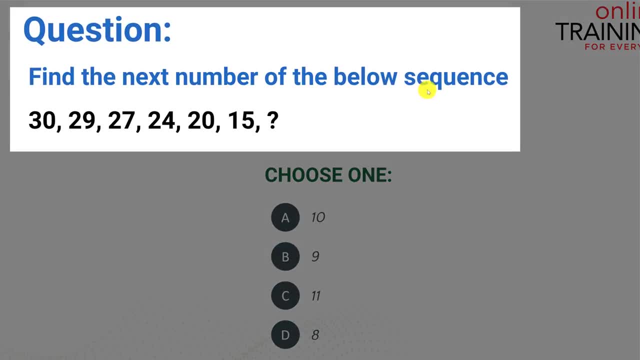 and logical reasoning tests, find the next number of the below sequence And you have a series of numbers- 30,, 29,, 27,, 24,, 20,, 15,- and you have a choices, four different choices: 10,, 9,, 11, and 8.. 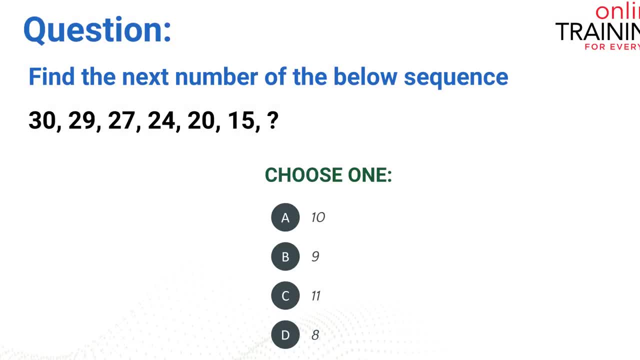 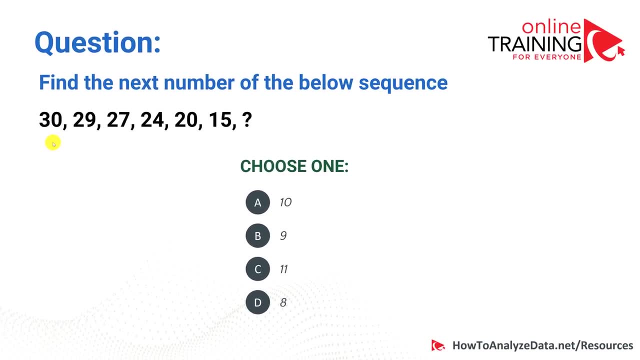 Which one do you think is right, And how would you even approach answering something like this? The key to answer something like this, in these types of questions in general, is to detect the pattern. So you see, the pattern here is you encourage the answer to the question and you 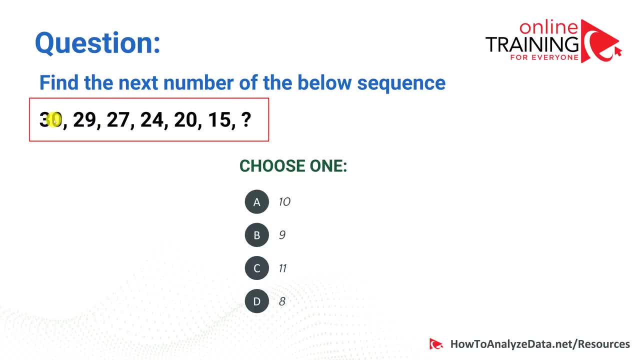 increase the number every time you go from one number to the next. 30 is one more than 29, and 27 is two more than 29.. 24 is three more than 27,, 20 is four more than 24, and 15 is five more. 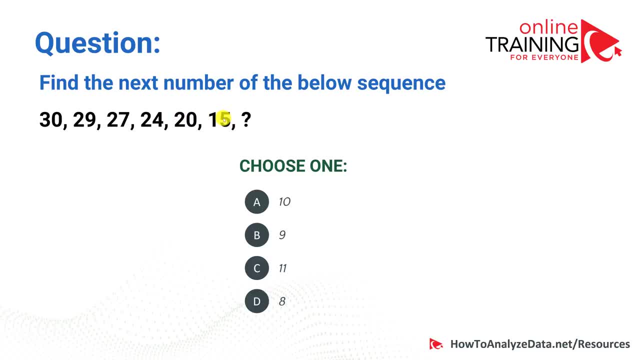 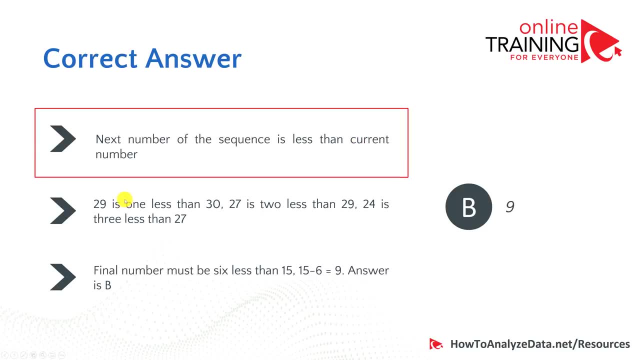 than 20.. So the next difference would be six, and 15 minus six would be nine. Let's recap: So next number in the sequence is less than the current number, 29 is less than 30, 27 is two less. 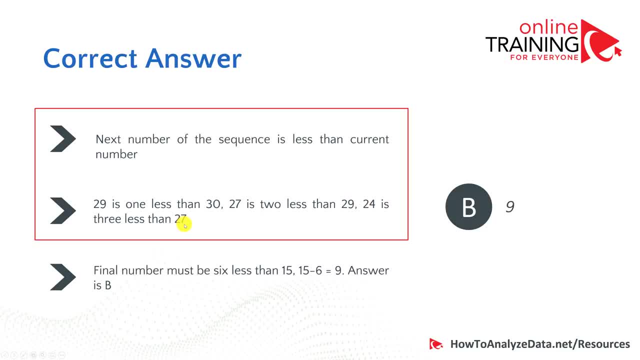 than 20, and 15 minus six would be nine. Let's recap: So next number in the sequence is less than 29, and 24 is three less than 27.. And you can continue the sequence once you detect it. And 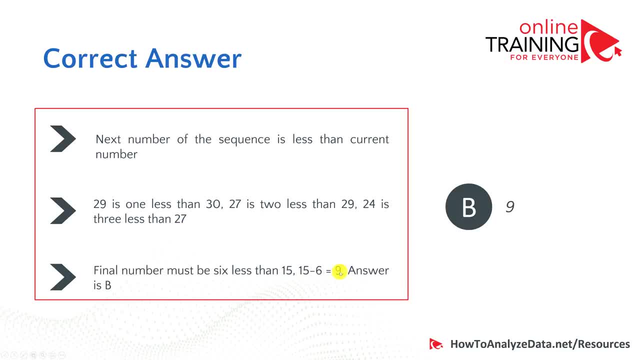 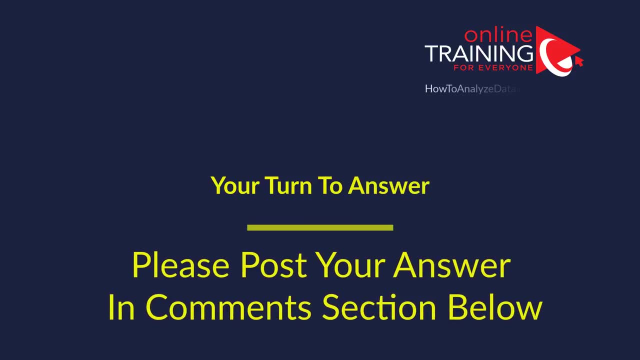 final number must be six less than 15, which is nine. So the correct answer is B, which is nine. Hopefully you've got this one right And now it's your turn. Please make sure to post your answer in the comment section below this video so I can give you the grade. Here's the question for you. 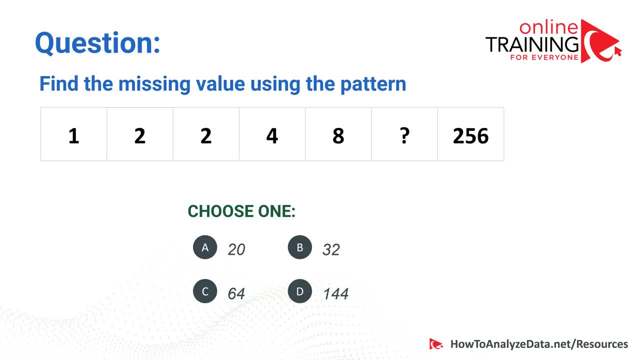 to answer: Find the missing value using the pattern, And you have pattern of numbers one, two, two, four, eight, a value that's missing and then 256. You need to choose one from the list And the choices are 20,, 32,, 64, and 144.. What do you think is the right answer here? Please make. 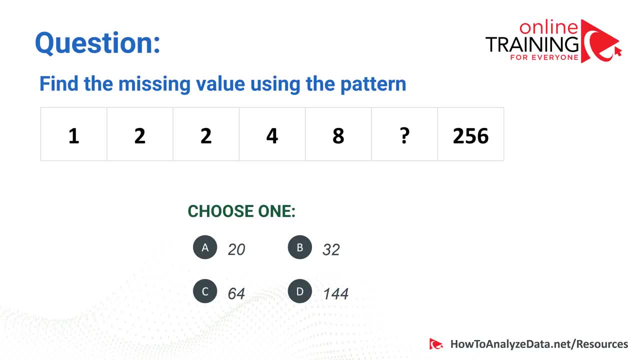 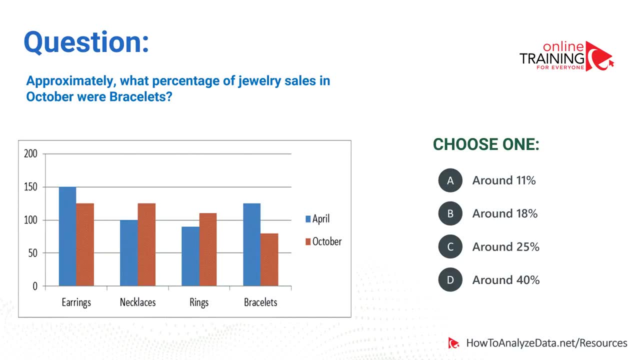 sure to post your answer in the comment section below this video so I can give you the grade. Now let's look at the question which tests your knowledge of charts and graphs, math reasoning and logical reasoning. Approximately What percentage of jewelry sales in October were bracelets? 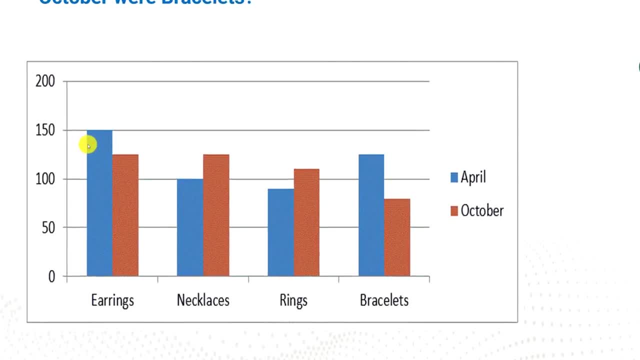 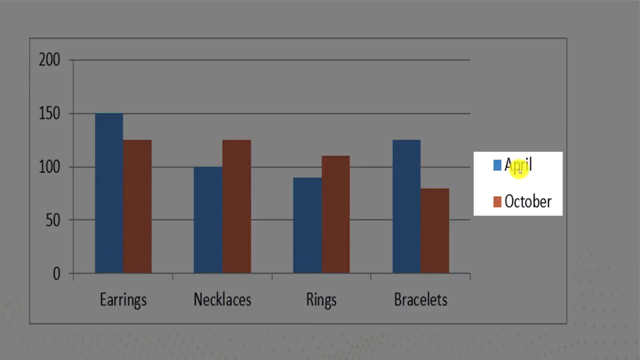 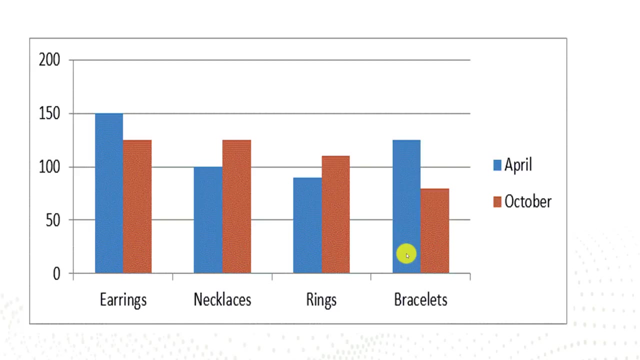 And you present it with the graph, which has four sections. Each section has two bars. Each bar represents monthly sales, Blue bar represents April sales for different types of jewelry And orange bar represents October sales for the same jewelry, For example for bracelets. 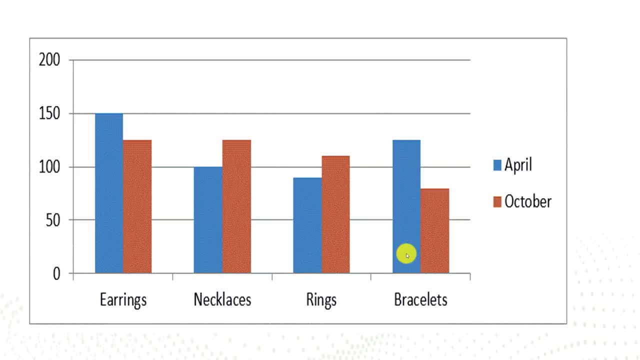 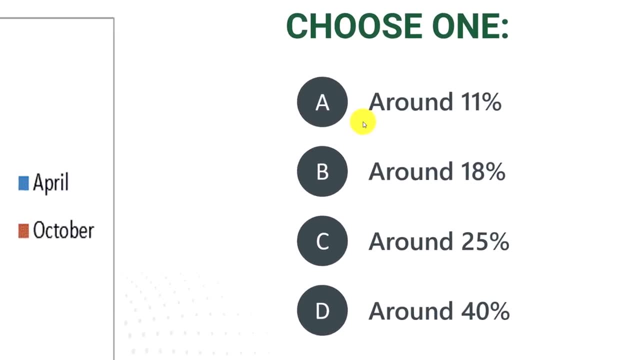 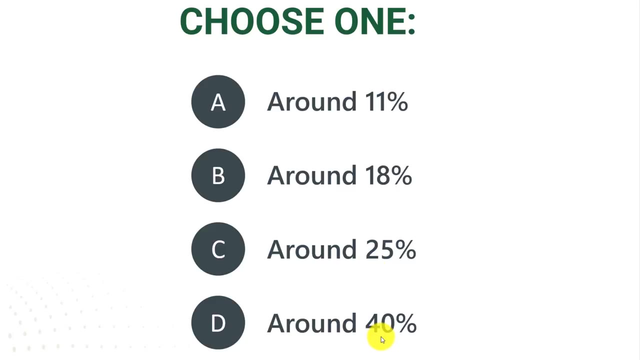 April sales are approximately 125 items, versus October sales are approximately 80 items. You have four choices to answer this question: Around 11%. choice B: around 18%, around 25% or around 40%. So how would you approach this question? Which one do you think is the right answer? 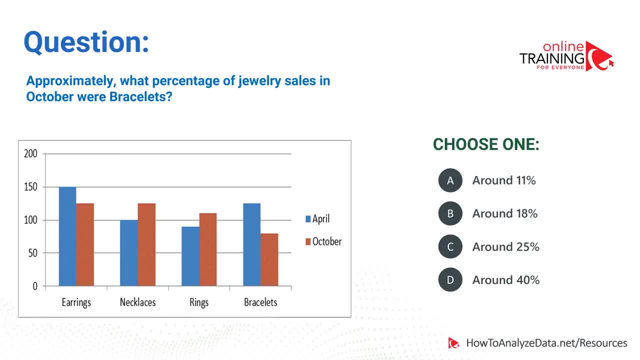 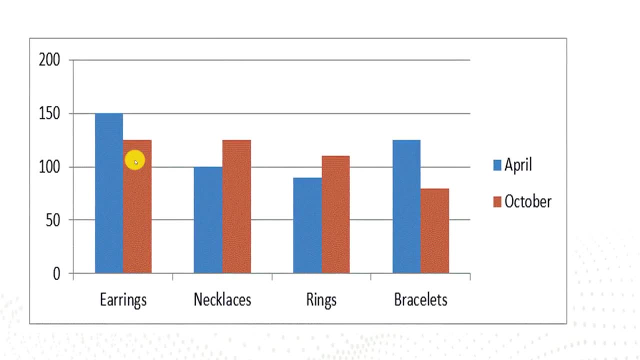 To answer this question, you need to add up all jewelry sales for October and then understand what percentage of those were bracelets, For example, for earrings, the value is about 125.. Same thing for bracelets For rings: it's about 110.. And for bracelets: it's about 80.. Let's add up all. 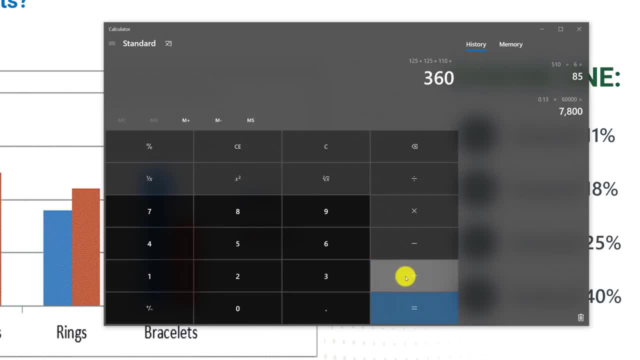 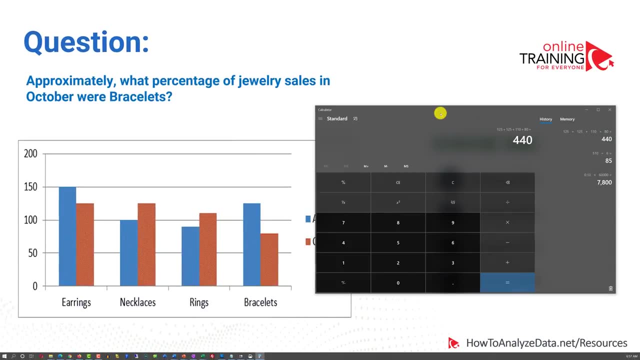 these values in the calculator. The total number for October sales of jewelry is 440 items. Now we need to divide 80, which are the bracelet sales, by 440 and multiply by 100.. What percentage of jewelry sales in October were bracelets? 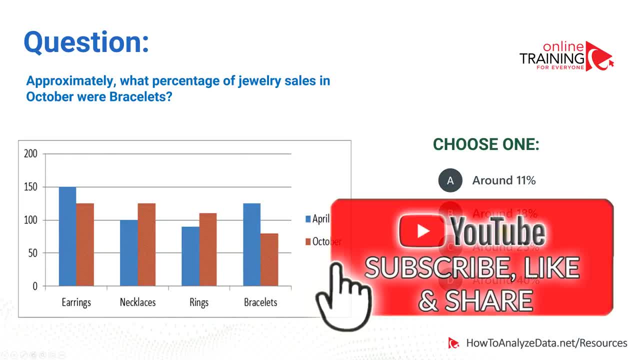 The answer is about 80.. For rings it's about 110.. And for bracelets it's about 80.. Let's add up all these values in the calculator 18,, which means that sales of bracelets are about 18% for October. 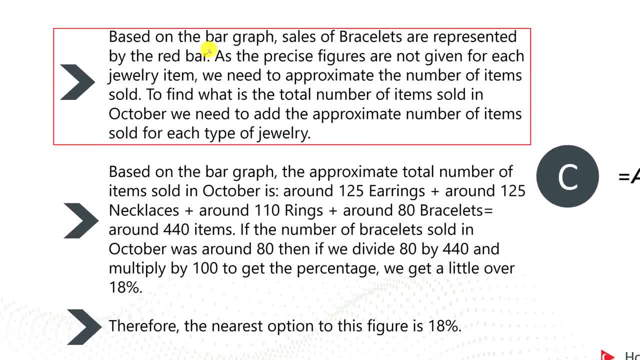 Let's recap. Based on the bar graph, sales of bracelets are represented by the red bar. We do not have precise figures for the sales, so we need to approximate the numbers Based on the graph. the approximate number of items sold in October are about 125 earrings. 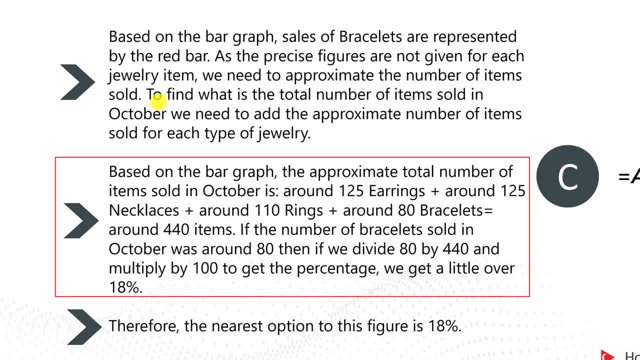 about 125 necklaces and about 110 rings, plus about 80 bracelets. To calculate the percentage of bracelets sold, we need to divide 80 by 440 and multiply by 100.. The number of bracelets sold in October is represented by about 18%. 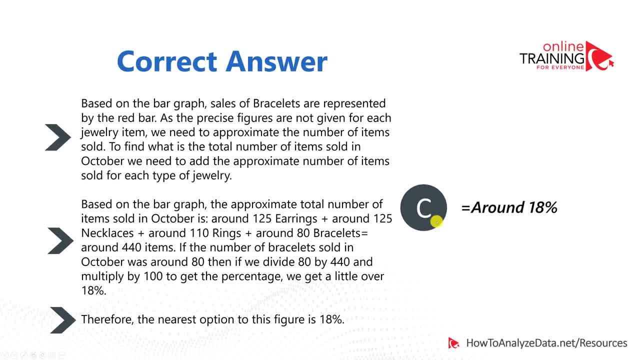 To calculate the percentage of bracelets sold, we need to divide 80 by 440 and multiply by 100.. The number of bracelets sold in October represented by about 18%. Hopefully you've got this one correctly, as this question involved a lot of calculations. 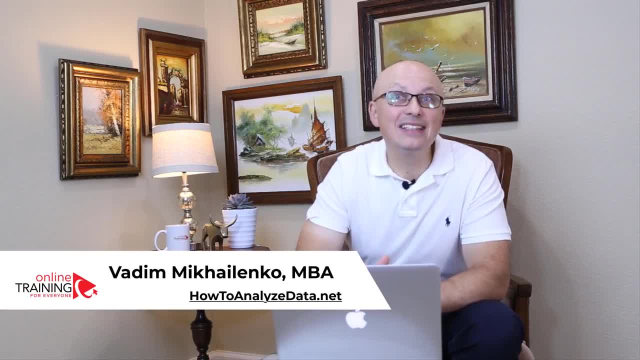 A lot of students ask me: how can I learn quickly? Let's look at all different options based on recent scientific research. Let's look at all different options based on recent scientific research. One of the most effective ways to learn quickly is to use the calculator. 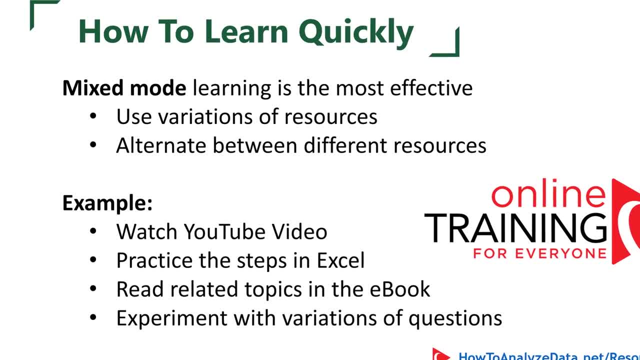 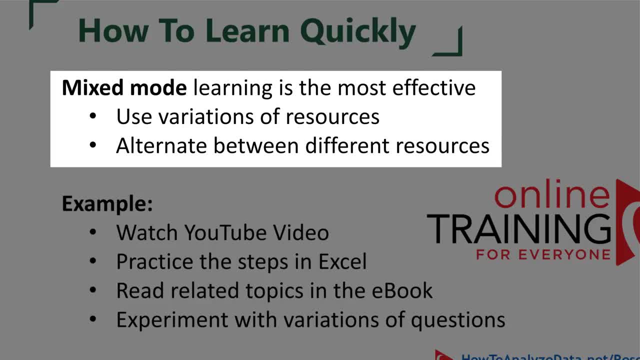 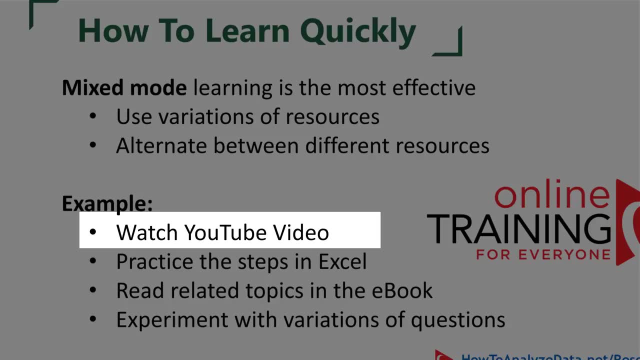 ways to learn we recommend to our students is a mixed-mode learning. you use variety of different resources during mixed-mode learning and alternate between them to ensure better comprehension of the material. for example, if you're trying to get ready for Excel assessment test, you can start by watching YouTube videos, then practice the steps in Microsoft Excel read. 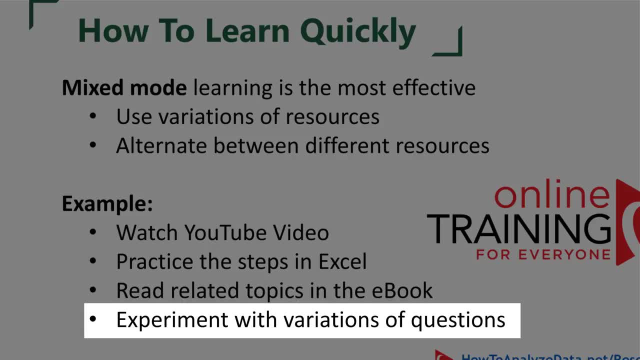 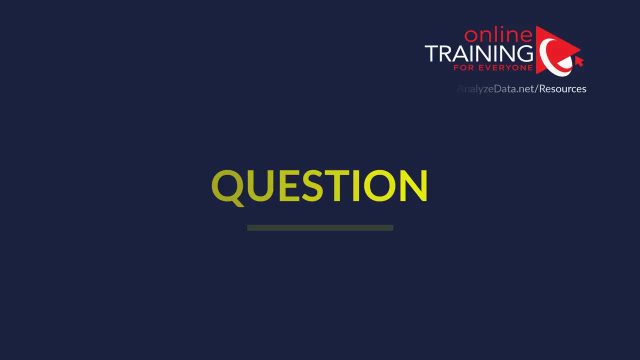 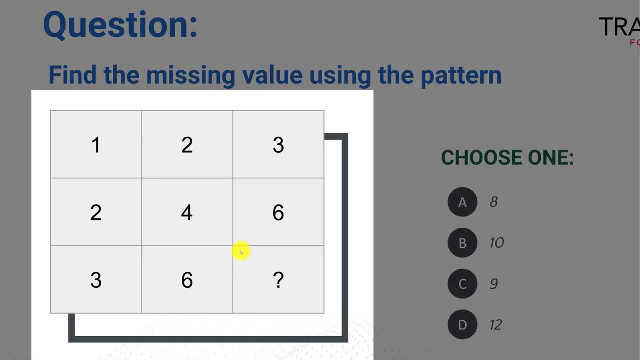 related topics in the e-book and then experiment with variety of questions during practice test. you now- let's look at the question- find the missing value using the pattern. you see the three by three box and one of the values in this box is missing. so what is? 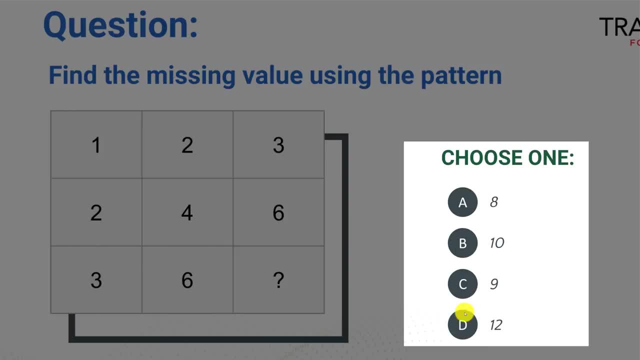 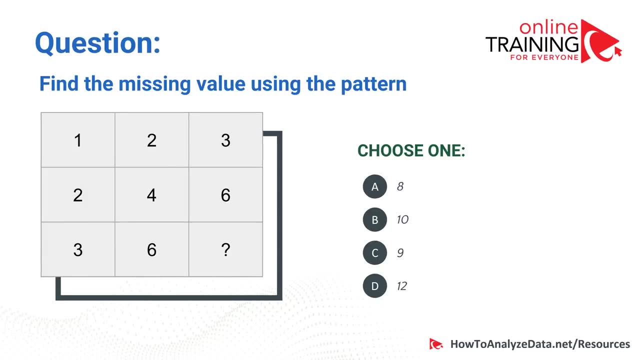 the pattern and there are four choices. we have a, B, C and D right, and obviously you would have to find the pattern and calculate the value. so what do you guys think is the right answer here? before I reveal the right answer, let me try to discuss with you the pattern. 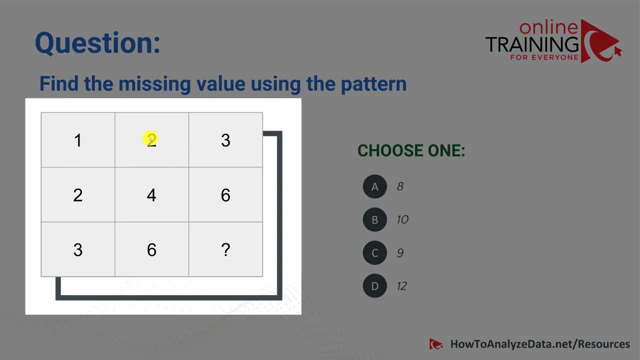 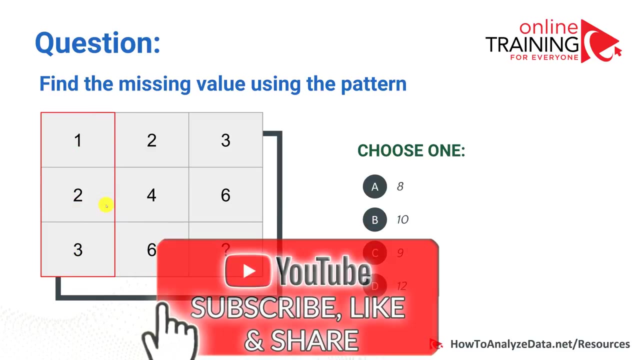 so you see one, two and three right, but then this one, two, four and six, so it's not sequential. so it's not like you go: one plus one equals two plus one equals three. there is a different type of pattern here, and the right pattern here is that one plus two equals three right, and then two plus four equals six and 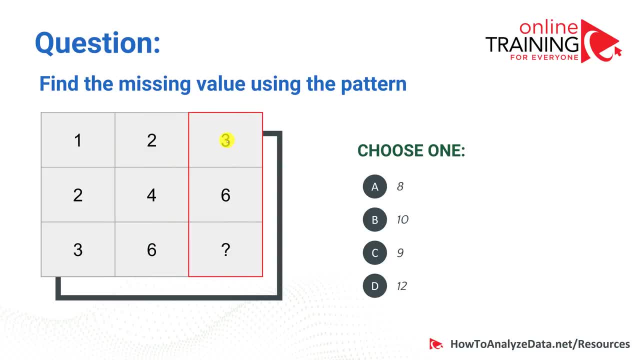 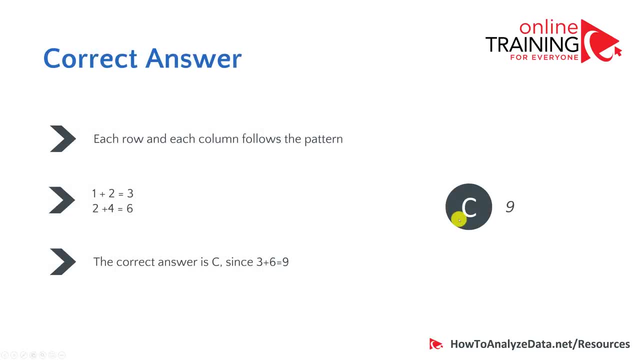 once you know the pattern, you can easily calculate that three plus six equals nine. so the right answer here's choice C. let's validate, and you're absolutely right: the right choice is choice c and this is exactly the logic that i just presented to you. hopefully you've got this one right. people contact me and ask what's changed. 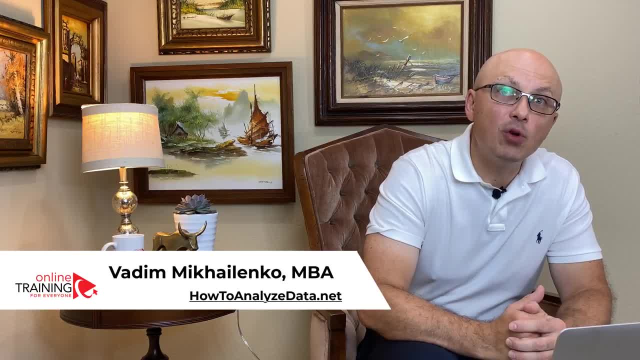 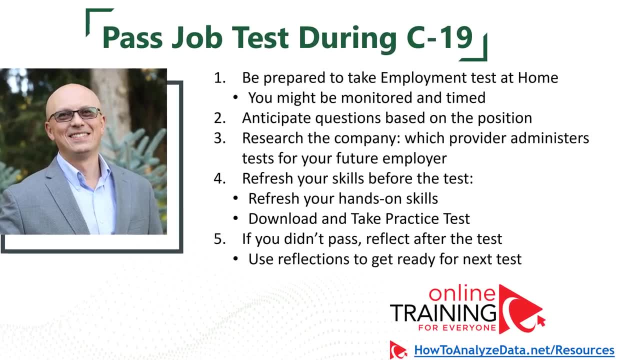 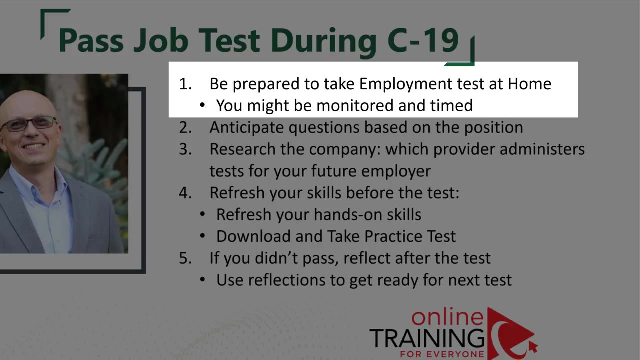 during carpet 19.. let's look at the changes in employment assessment test process that have happened recently. one of the biggest changes is the fact that a lot of people work remotely, which means a lot of hiring also happening remotely. provider might ask you to install special software to monitor your desktop activities. they might also ask you to enable 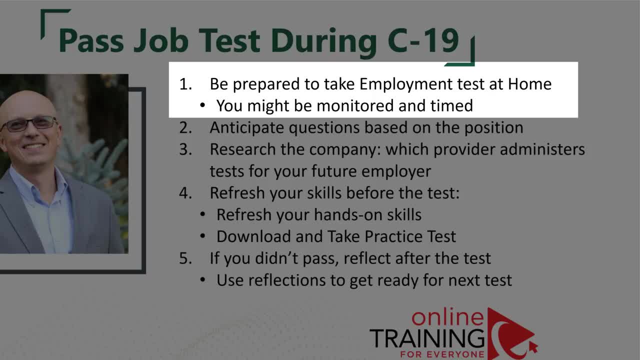 your camera to see what you're doing during the test. another big shift we see is that the questions become more relevant to the position. for example, if you're applying for accountant or bookkeeper job, make sure you know how to import the data. do profit and loss reports? 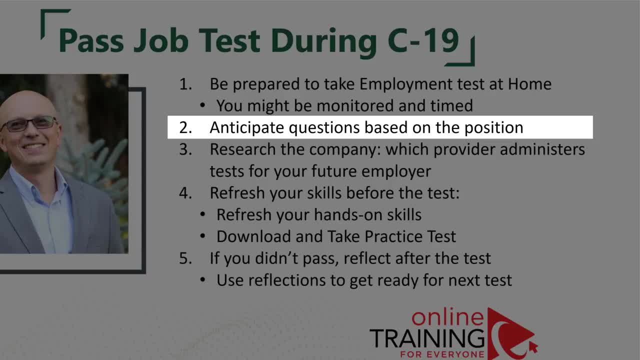 calculate the expenses and calculate the annual statements. these are the types of questions that you might see for that specific position. researching the company and researching the test provider always works for our students. once you know who the provider is, you can try to go to their website to see the sample questions to get an idea what kind of 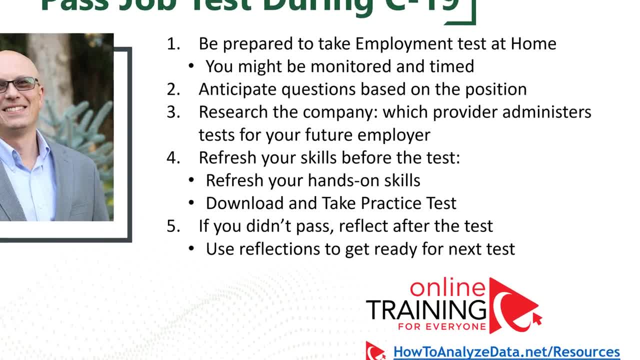 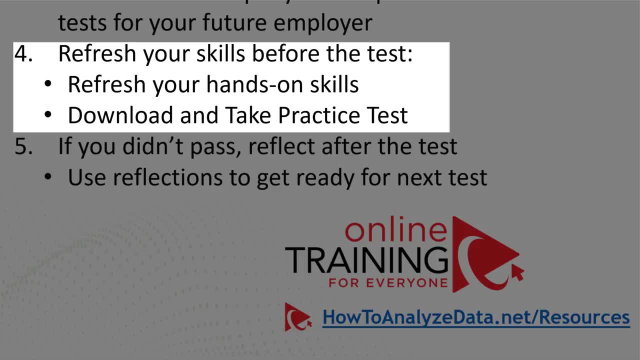 questions you're going to get on the test. it is always a good idea to refresh your hands-on skills and practice before the test. this gives you necessary boost of confidence and allows to pass the test with the higher grade. if you didn't pass the test, make sure to reflect after it. 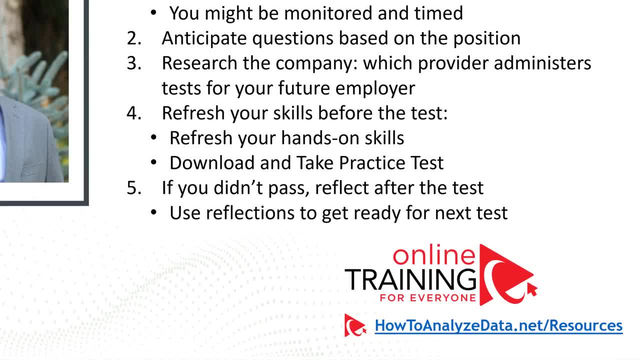 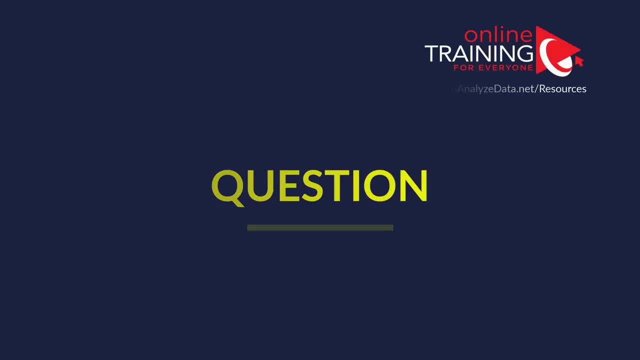 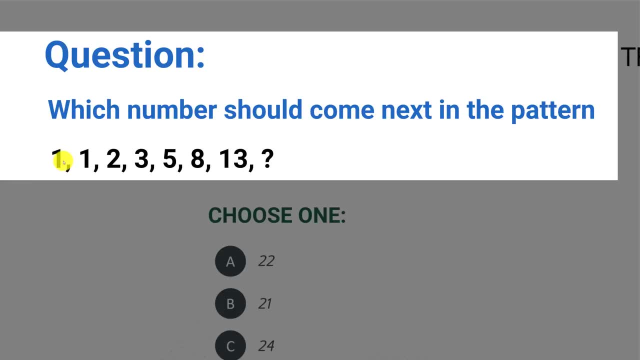 take notes and develop an action plan to see what the next steps might be to get you the job. now let's look at another pattern type question: which number should come next in the pattern? and then you have pattern of numbers one, one, two, three, five, eight, thirteen. so let's first determine what's. 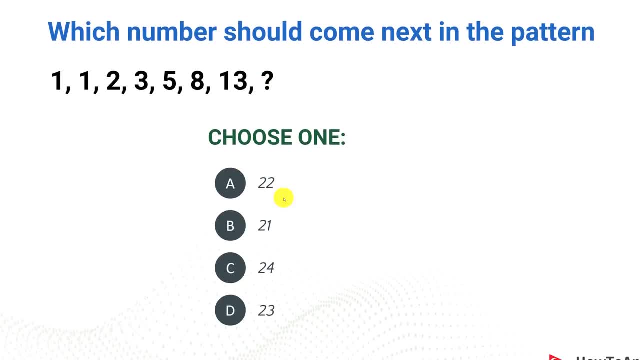 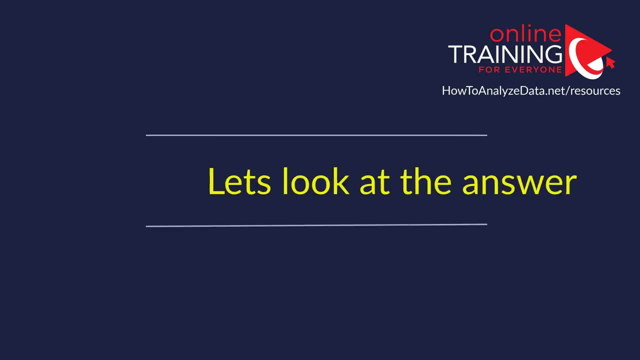 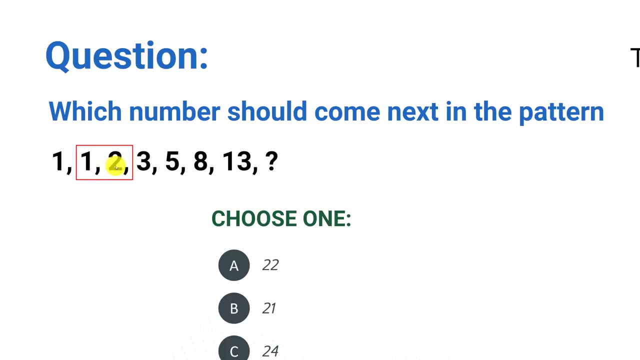 the pattern here. obviously there are four choices, but the result here is calculated based on the pattern that we would need to determine which one do you guys think is the right one here. well, let's look. so we have one one, and then one plus one equals two. then one plus two equals. 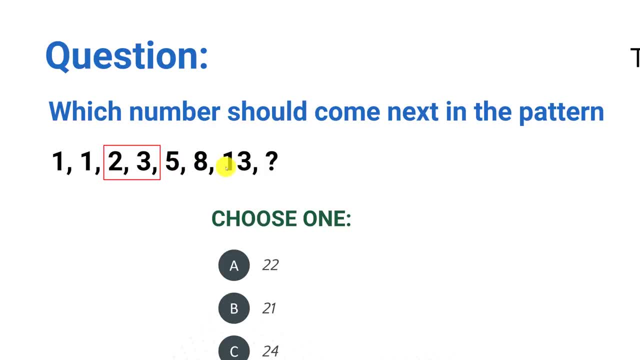 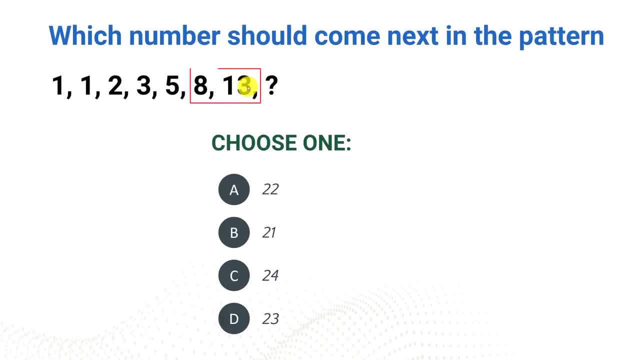 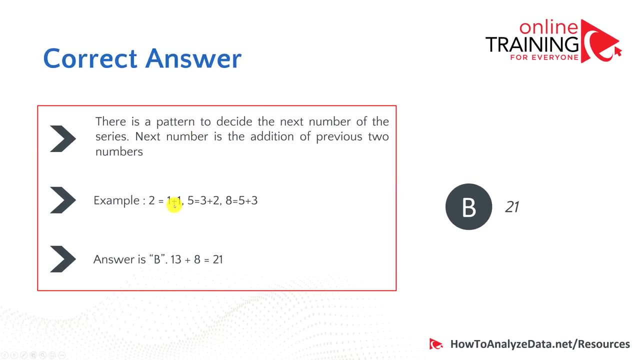 three. then we have two plus three equals five, and then you can kind of keep going. so to calculate the next number, it's basically the sum of the previous two numbers. so 8 plus 13 is 21. so the right choice here is choice b, which is 21.. and this is the explanation that the pattern here is. 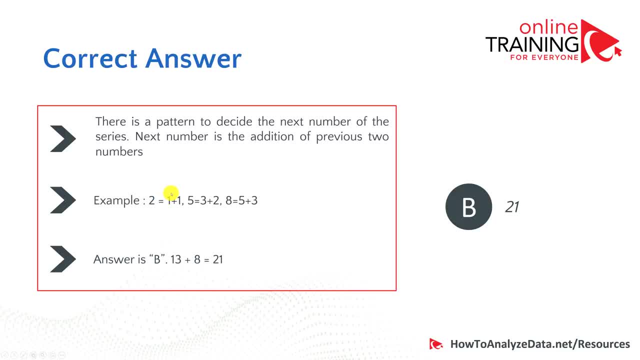 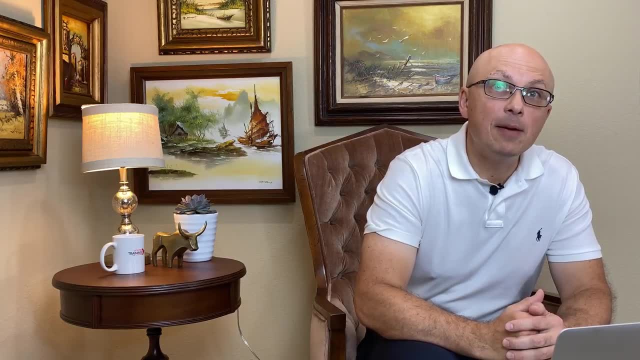 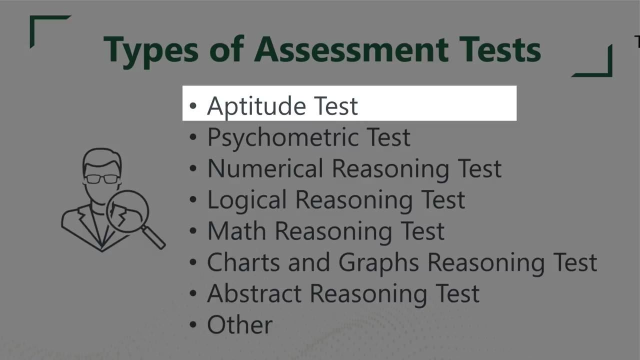 really the sum of previous two numbers. let's look at the most common options that you might encounter. most common tests that you see as part of the hiring process are: aptitude test, psychometric test, numerical reasoning test, logical reasoning test, math reasoning tests, charts and graphs reasoning test- abstract. 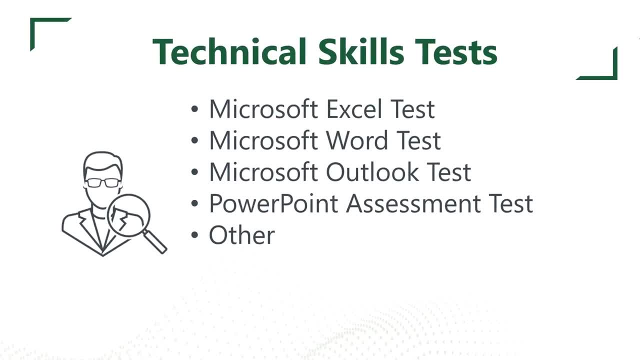 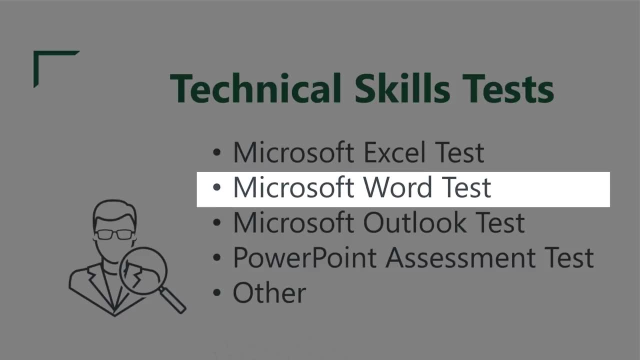 reasoning tests and a lot of others. sometimes, companies also would like to test your technical knowledge based on the fact that you're in the hiring process and you have a good reputation for on the job that you're applying for. You might encounter Microsoft Excel test, Microsoft Word, 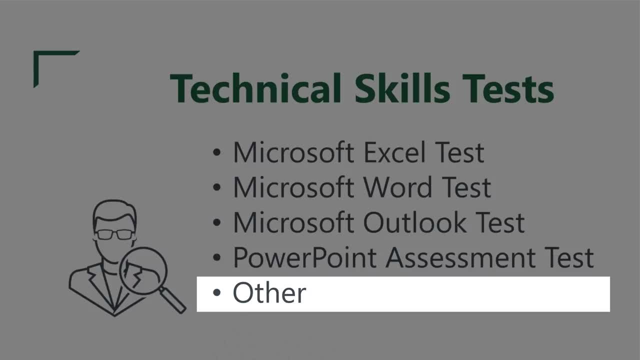 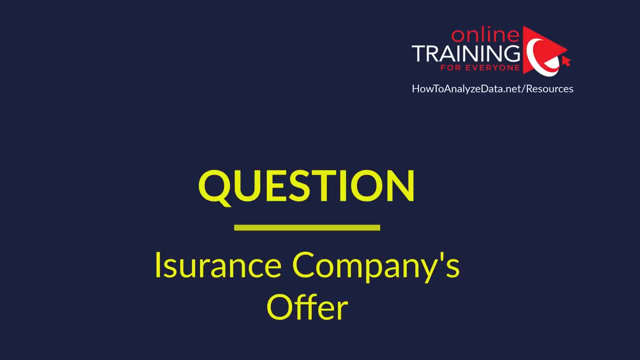 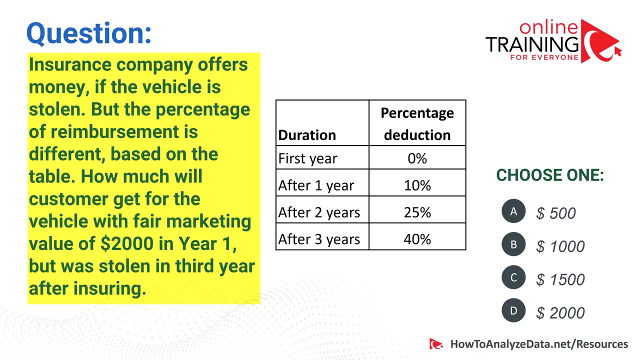 test Outlook, PowerPoint and a lot of other different tests that might be required for you to succeed on your job. Let's look at the question which is frequently used when you're applying for the jobs with financial companies: Insurance company offers money if the vehicle is stolen. 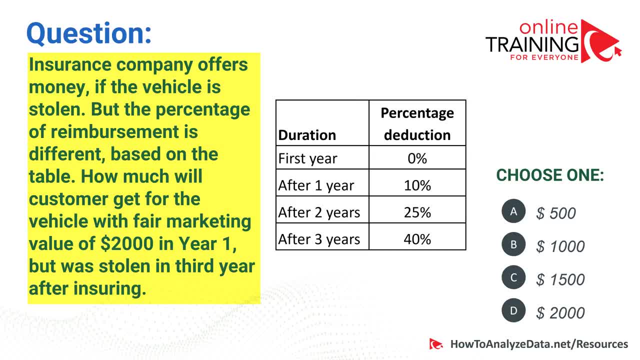 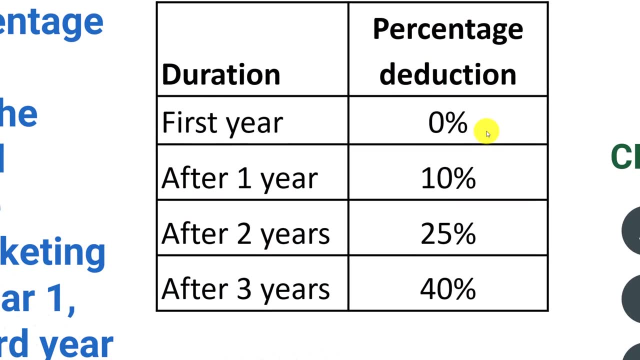 but the percentage of reimbursement is different based on the table. How much will customer get for the vehicle with fair market value of $2,000 in year one but was stolen in the third year after insuring? You have a table and it shows that percentage deduction in first year there. 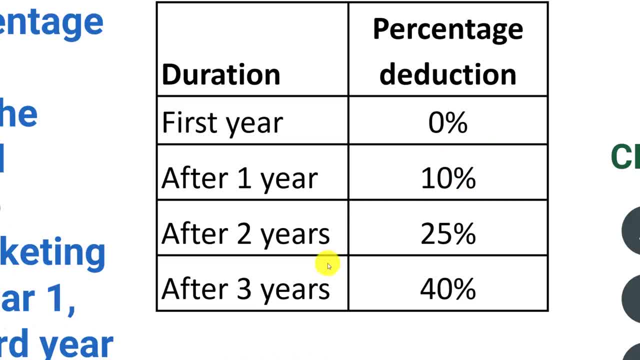 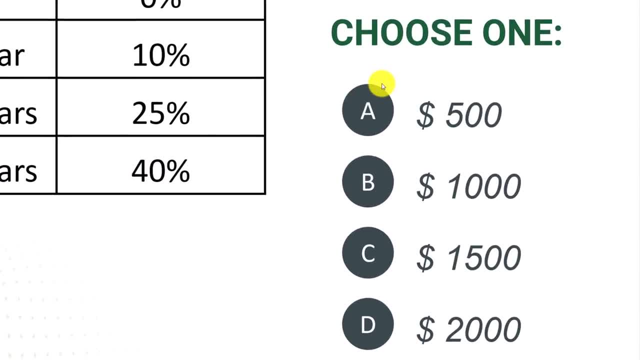 is no deduction After one year. there is a 10% deduction, After two years, 25.. And after three years, 40%. And you have four choices: $500,, $1,000,, $1,500, and $2,000.. Which one do you? 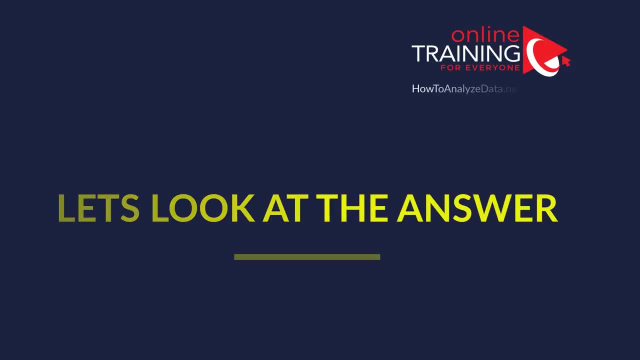 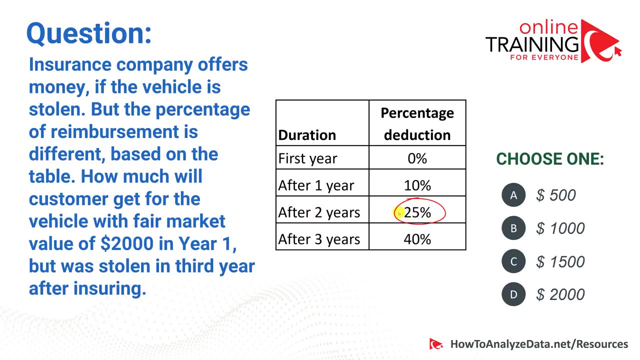 think is right choice here. Let's look at the question which is frequently used when you're applying for the job with. Let's look at how you would approach answering this question. After two years you would have to deduct 25% of the original cost of the vehicle. 25% of $2,000 is $500.. So $2,000 minus $500 that. 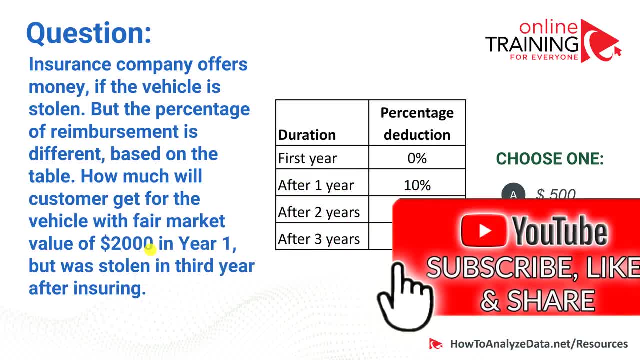 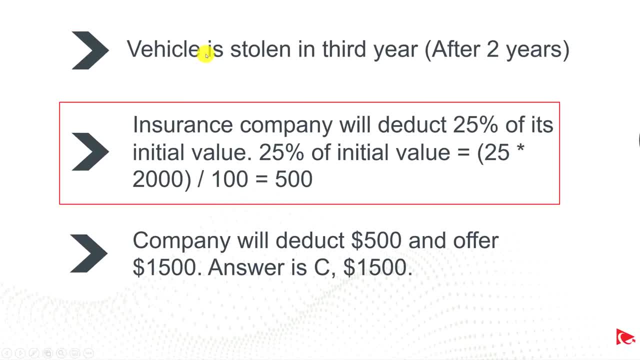 you would have to deduct would be $1,500 reimbursement that you can get from insurance company. Let's recap: Vehicle is stolen in the third year after two years. Insurance company will deduct 25% of initial value, and 25% of initial value is $500.. 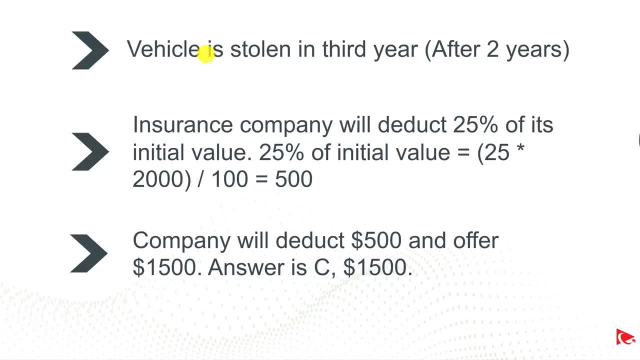 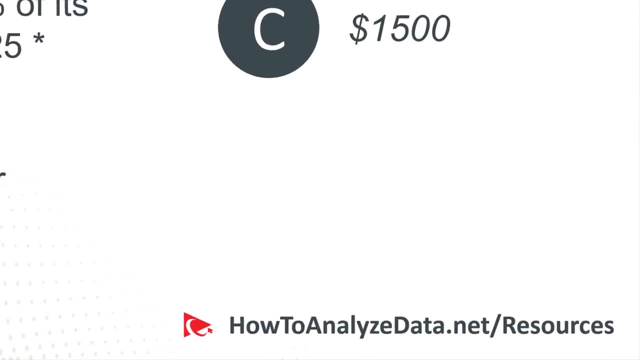 Company will deduct $500 and offer you $1,500. So the correct choice is answer C. Hopefully you've got this one right, But in case you need to practice more with similar questions, make sure to download my ebook with more practice questions using link in the description of this. 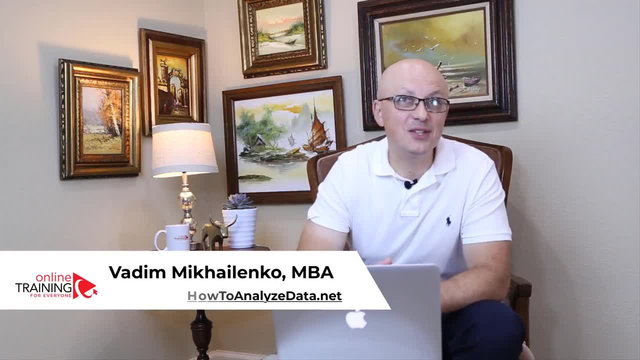 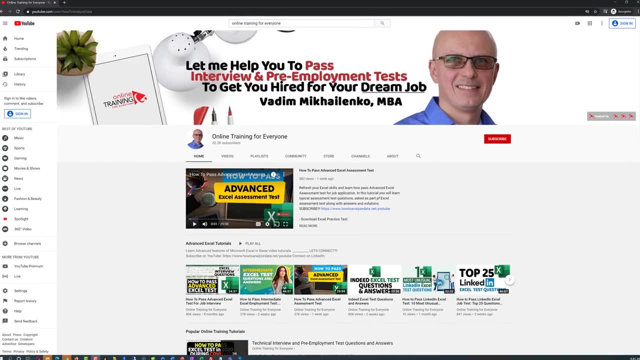 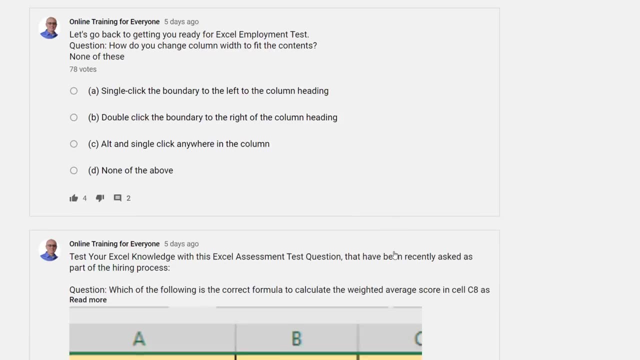 video. One of the best ways to learn is try to test your knowledge periodically. I encourage you to participate in our daily question challenge. Every day, we post a new question in the community section of the channel. You have an opportunity to test your knowledge and validate your skills on the different topics. 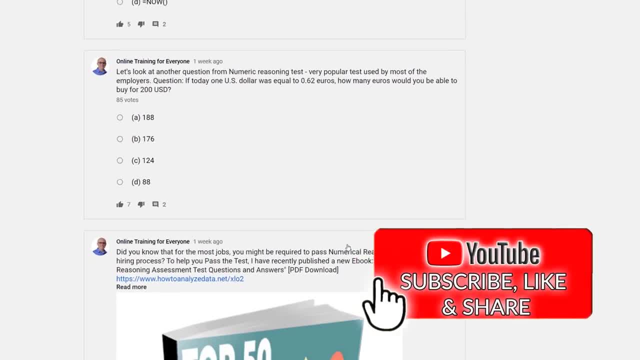 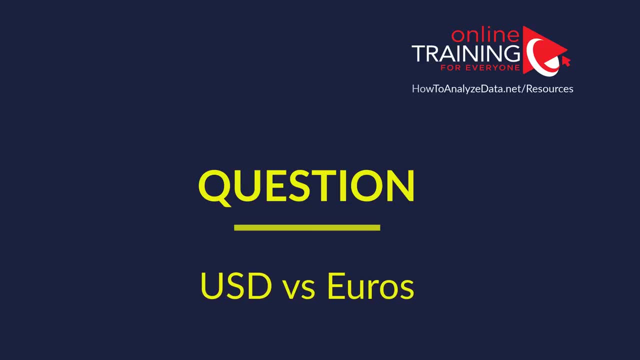 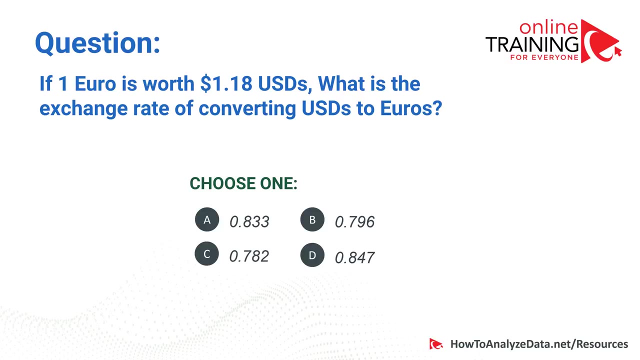 This is one additional reason to subscribe to the channel, because this way, all the questions will be delivered to you automatically. Now let's look at the question which is very frequently used as part of aptitude tests when you're applying for the position in financial industry, especially in the banking and insurance. 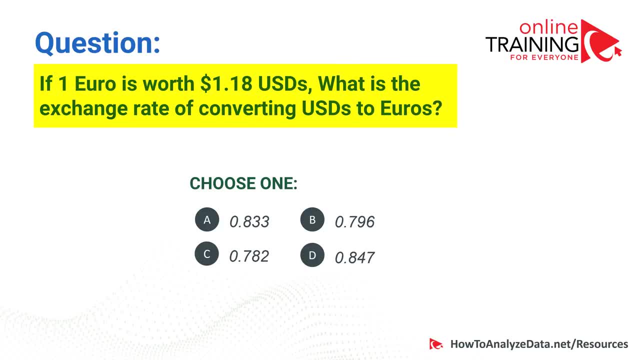 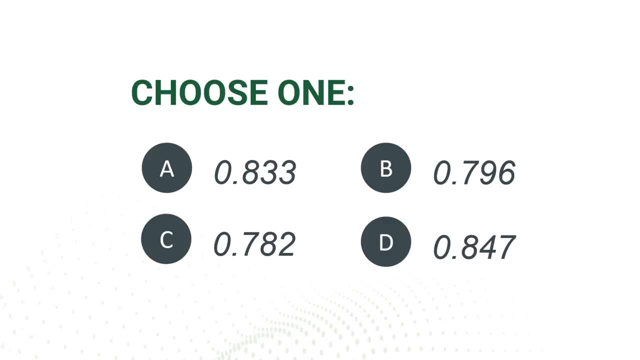 industries. If one euro is worth 1.18 US dollars, what is the exchange rate for the other euro? You have four choices here: 0.83,, 0.79,, 0.78, and 0.84.. How would you calculate this? 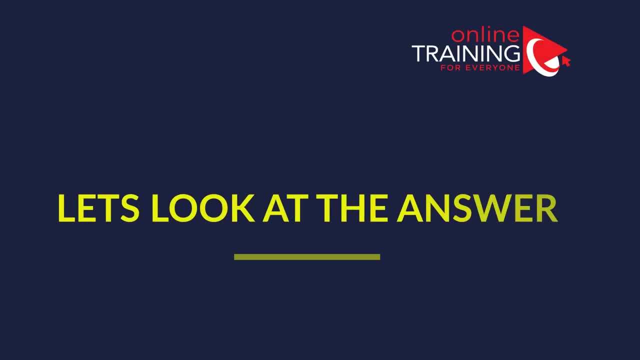 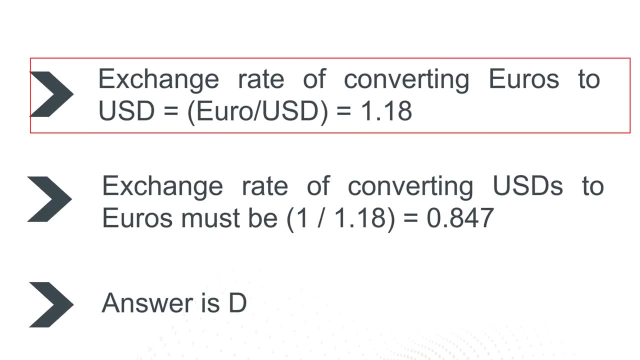 Let's see if you can nail this question. To get to the correct answer, we need to reverse the exchange rate. If exchange rate for converting euros to dollars is 1.18,, then exchange rate of converting dollars to euros must be 1 divided by. 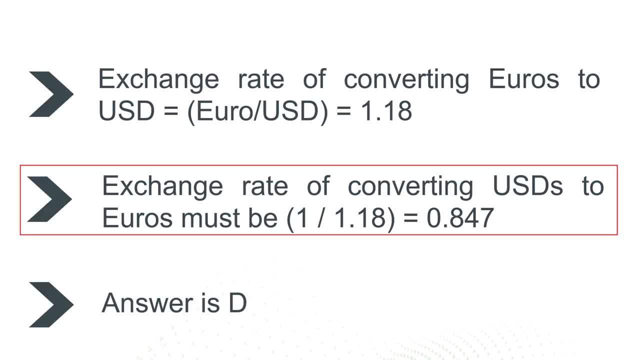 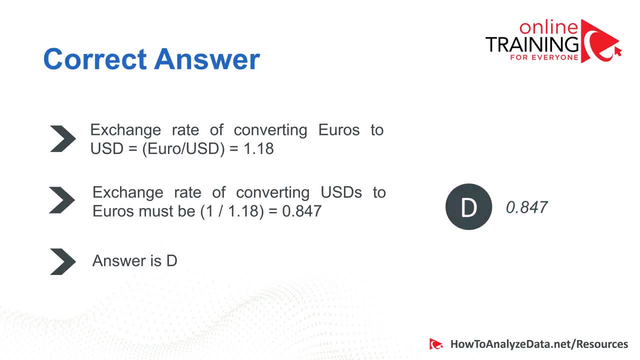 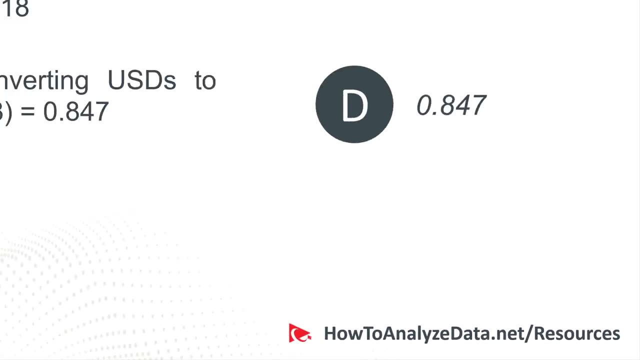 1.8.. So the correct answer here is D. I would imagine that you've answered this question correctly, but in case you need to practice more with similar questions, make sure to download my ebook with more practice questions using the link in the description of this video. 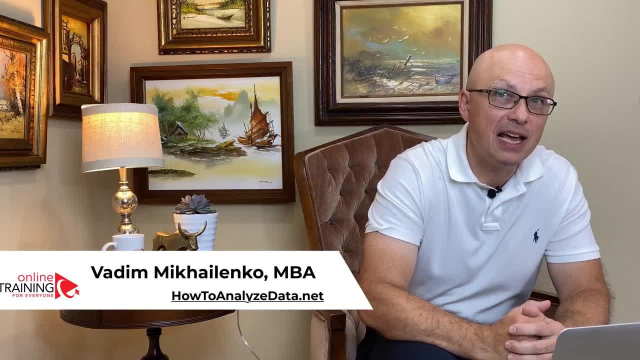 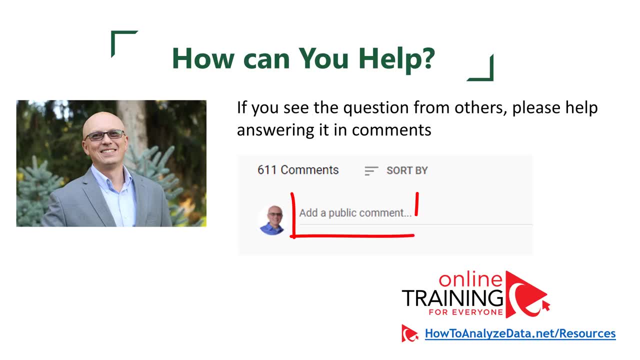 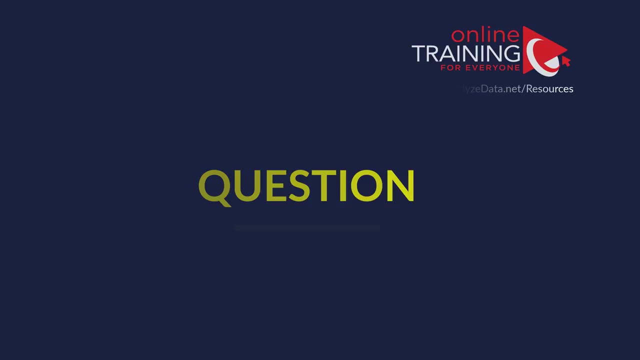 If you see questions on this channel that you know the answer to, please make sure to comment below. This way, you will help another person to get hired. Now let's continue and get you ready for the assessment test. Let's look at the question which tests your knowledge of logical reasoning. 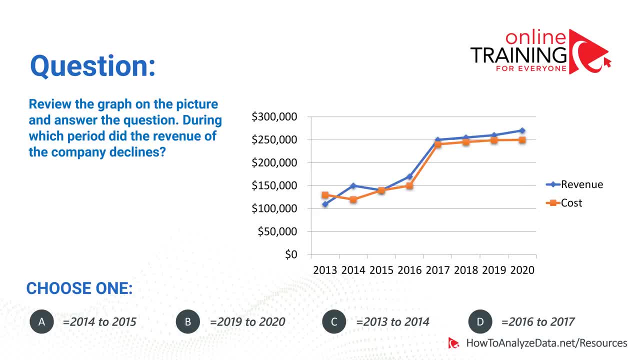 and how well you can apply this knowledge to charts and graphs. Review the graph in the picture and answer the question: During which period did the revenue of the company declines? There is a picture represented here with two lines: One blue line that shows revenue. 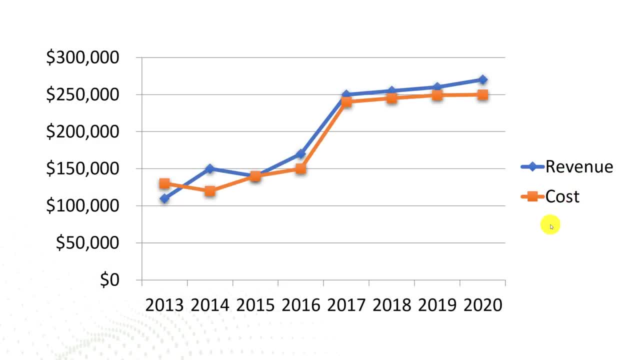 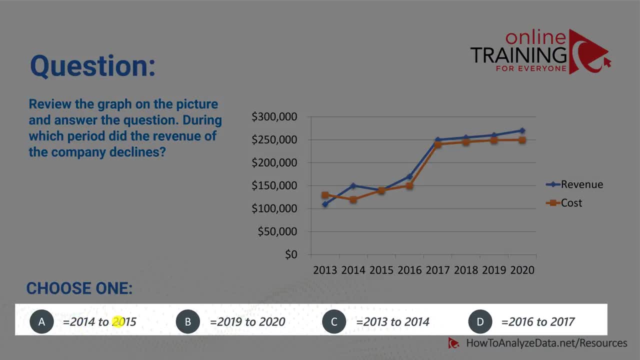 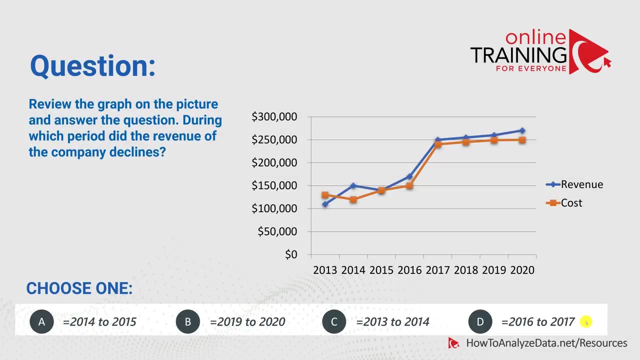 And then the orange line which shows the cost. The period is from 2013 to 2020.. And you have four choices to select: from 2014 to 2015,, 2019 to 2020,, 2013 to 2014, and 2016 to 2017.. 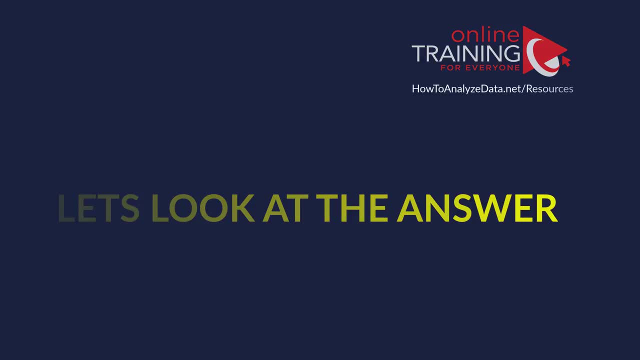 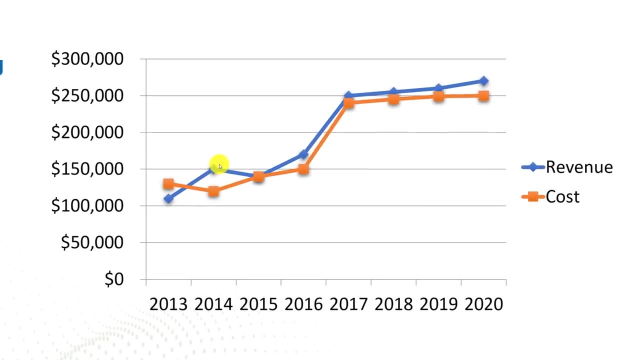 Which one do you think is right? To answer this question correctly, you need to differentiate between revenue and the cost, because revenue is represented by blue line. You have to follow the blue line To answer the question: in which period the revenue declines. 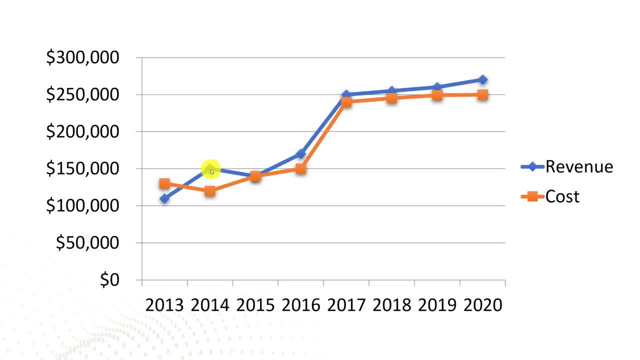 If you follow the line, you see that for all the years, with the exception of period of 2014 to 2015,. right here the line goes up, And only for the period 2014 to 2015,. revenue declines. 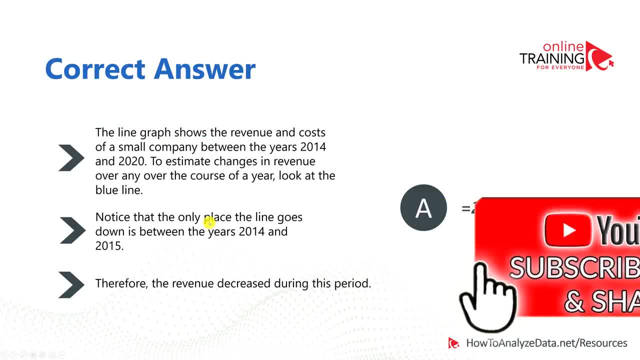 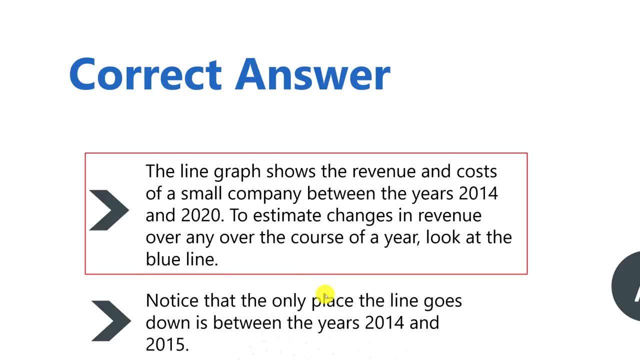 So that is the correct choice And that is the correct answer. Now let's recap. The line graph shows the revenue and costs of a small company between the periods of 2014 and 2015.. To estimate the changes, you need to find the spot on the line which goes down. 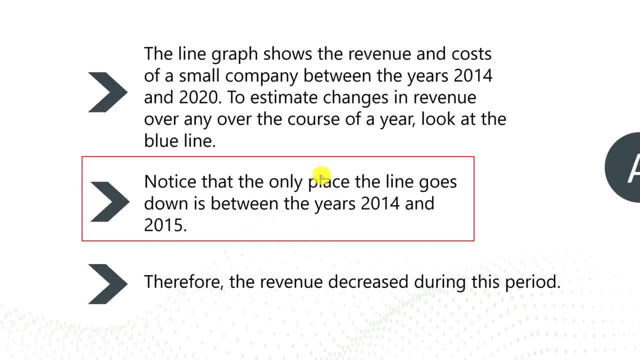 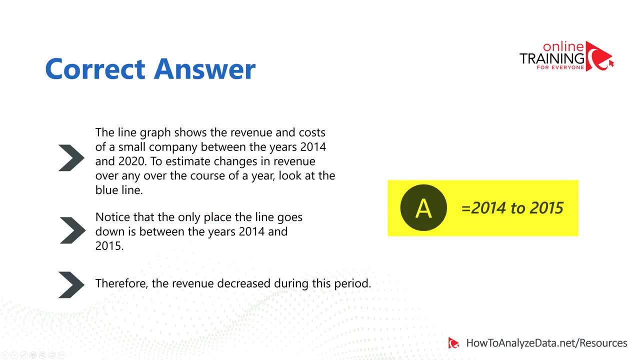 Only place when line goes down is between the years of 2014 and 2015.. Therefore, choice A, which shows 2014 to 2015,, is the right answer for this question. Hopefully you've got this one right. 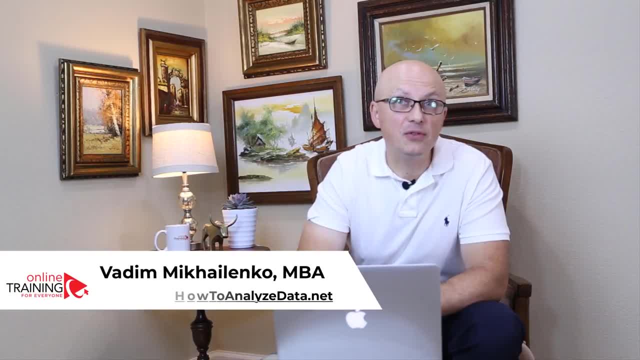 Can I ask you to do me a favor? If you know someone who will benefit from this material and looking for the job, please share this content with them. I really appreciate it. This will help them find the job, Thank you. Thank you very much. 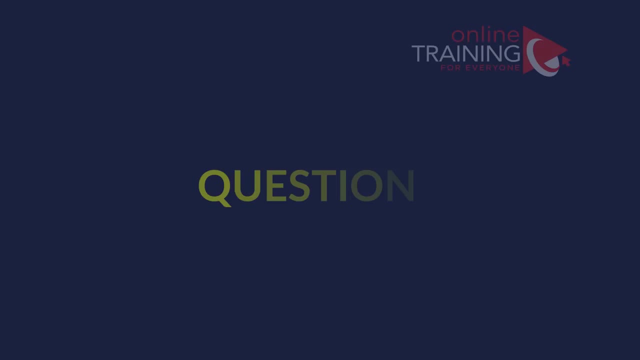 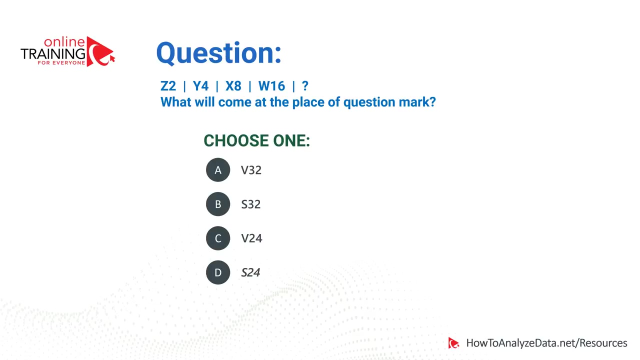 Now let's continue and get you ready for the assessment test. Let's look at the question, which is frequently used as part of verbal reasoning, logical reasoning, abstract reasoning and used as part of various aptitude tests. What will come at the place of question mark? 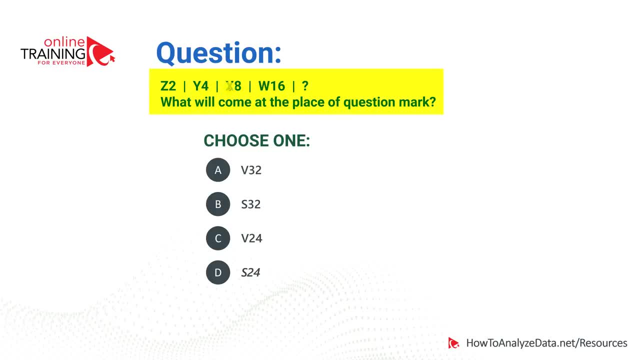 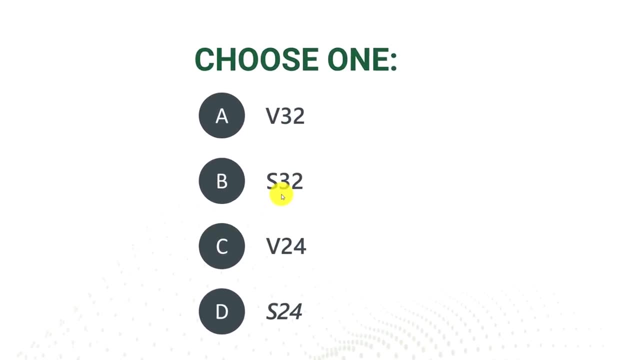 And you're presented with the series Z2, Y4,, X8,, W16, and in question mark, And you have four choices: V32,, S32,, V24, and an S24.. Which one do you think is right? 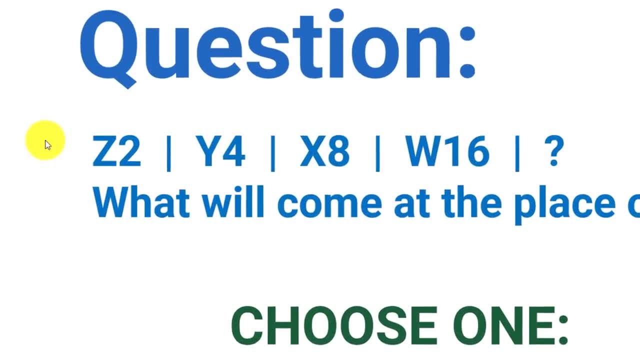 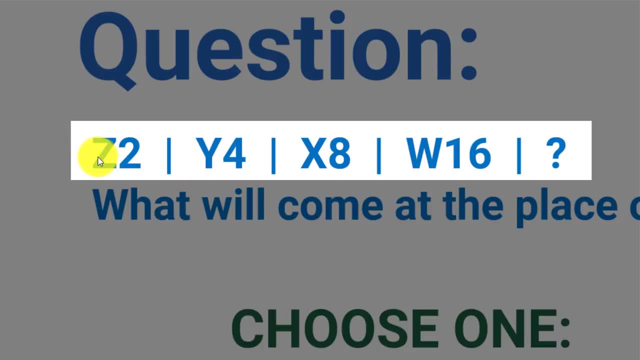 To answer this question you need to try to detect the pattern, And there are two patterns here presented in this question. First pattern is the pattern of the alphabet in reverse order. So you have letters Z Y X and W X Y Z, W X, Y Z. those are the last letters of the English alphabet. 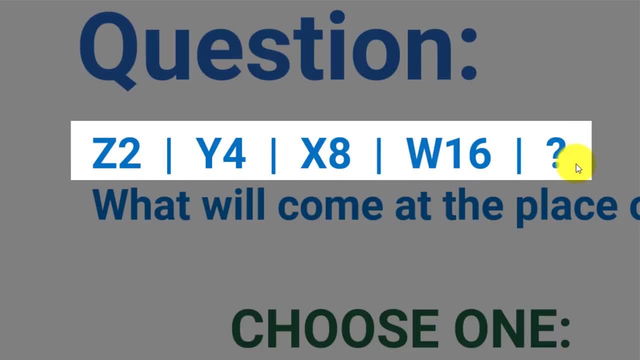 So the letter before Y Would be the letter that you need to put as the first character in the question mark. That's the first pattern. Then the second pattern is the pattern of numbers increasing. You have numbers increasing in the power of 2.. 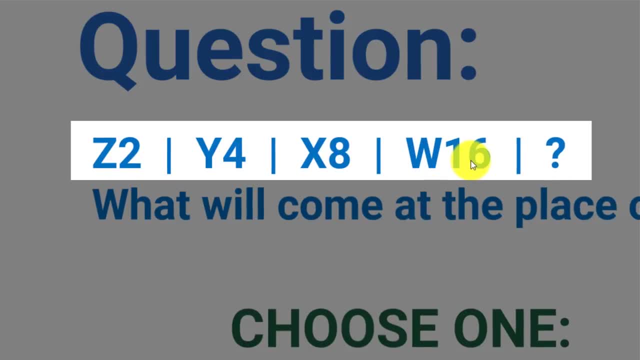 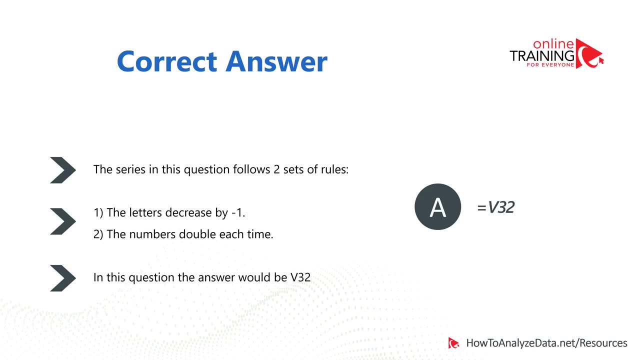 2, 4,, 8,, 16.. So the next one here would be 32.. So the correct answer here is V32.. Let's recap. To answer this question you need to follow two patterns. One pattern for the letters. 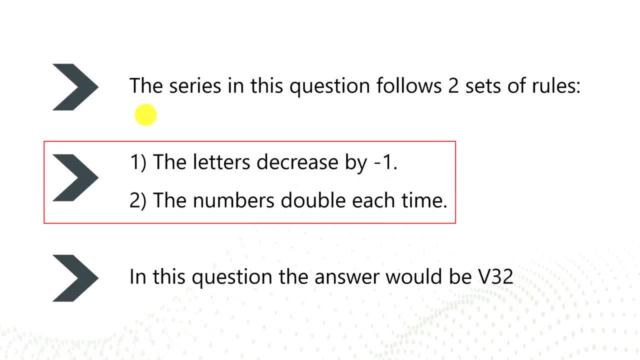 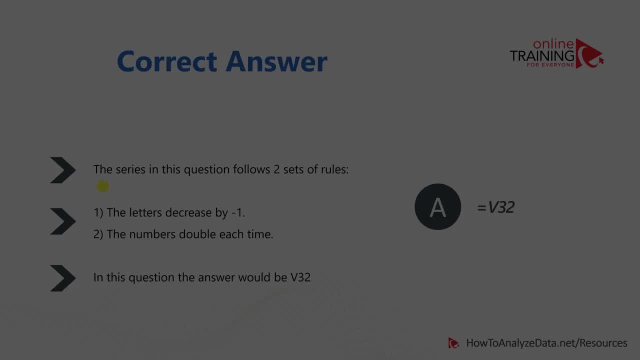 And second pattern for the numbers. The letters decrease by one And the numbers double each time, So the correct answer here is V32.. Hopefully you've got this one right. If you like the content, please give this video a big thumbs up. 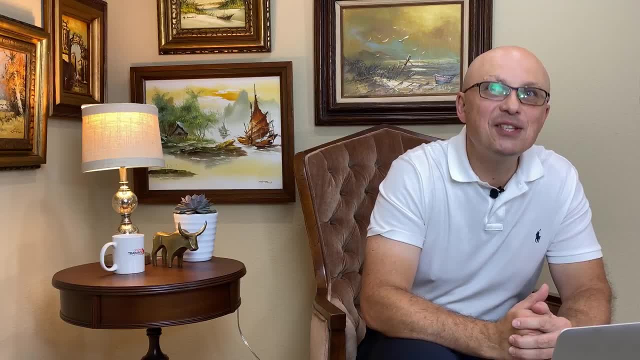 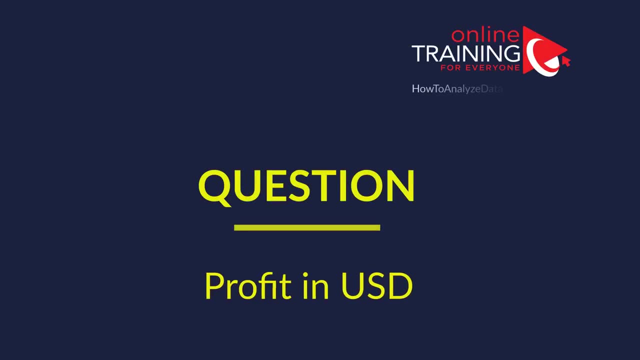 This tells us that you need more content like this, And we'll make sure that you get it in the future. Now let's continue and get you ready for the assessment test. Let's look at the question which you might get when applying for banking positions. 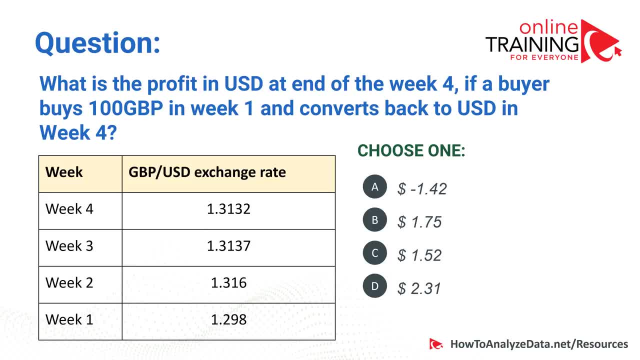 insurance companies or any other position within the financial industry. What is the profit in US dollars at the end of week 4 if a buyer buys 100 pounds in week 1 and converts back to US dollars in week 4?? 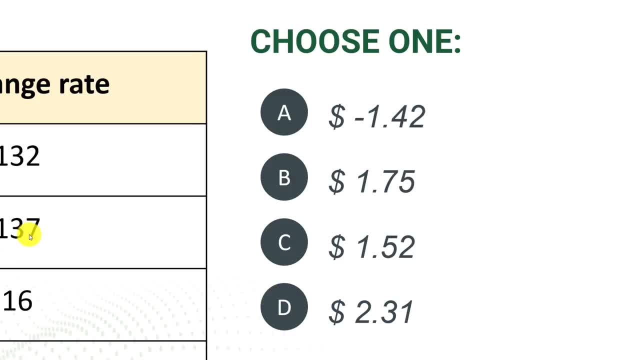 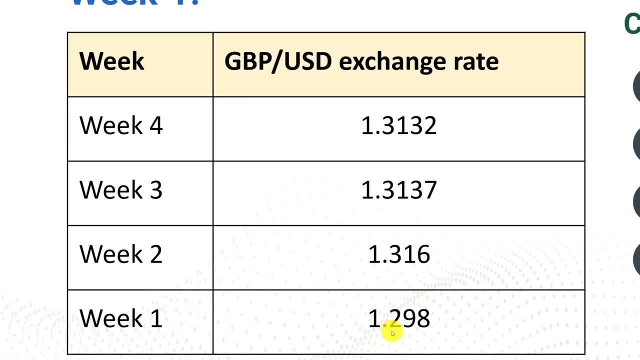 You have four different choices presented- A, B, C and D- And then you have a table Conversion rate between pounds and dollars for four weeks. In week 1, the conversion rate is 129.. And in week 4, the conversion rate is 1.5. 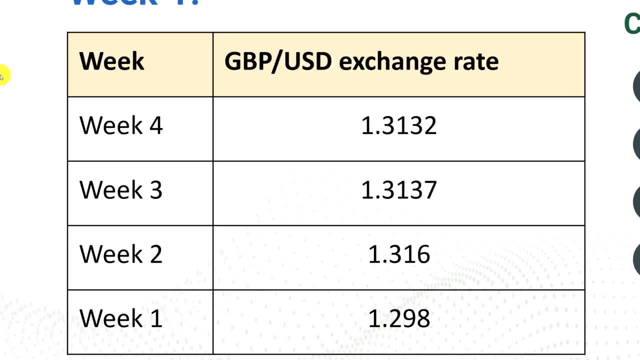 And in week 5, the conversion rate is 131.. Which one do you think is the right answer here? To get to the right answer, you need to calculate the values: the total sum of US dollars in week 1,. 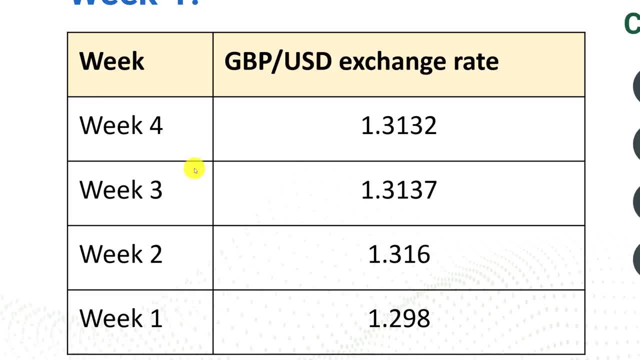 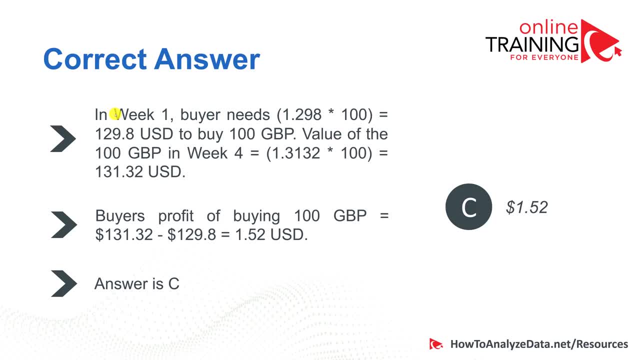 and then you need to convert it back to US dollars in week 4.. Ultimately, week 2 and week 3 values are irrelevant here, because you're holding through weeks 2 and week 3.. And this is how you do the calculation. 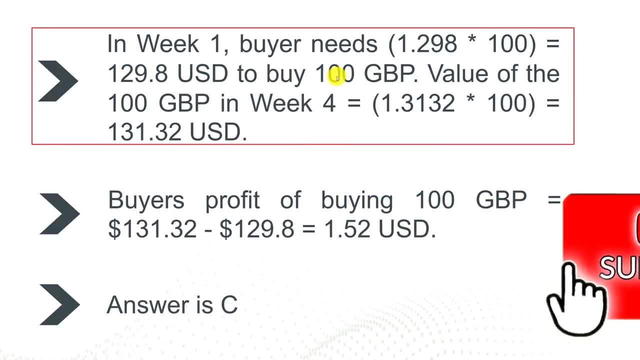 In week 1, you need 129 US dollars to buy 100 pounds. And this is how you do the calculation: In week 1, you need 129 US dollars to buy 100 pounds, While the total value of 100 pounds in week 4 is 131.32 dollars. 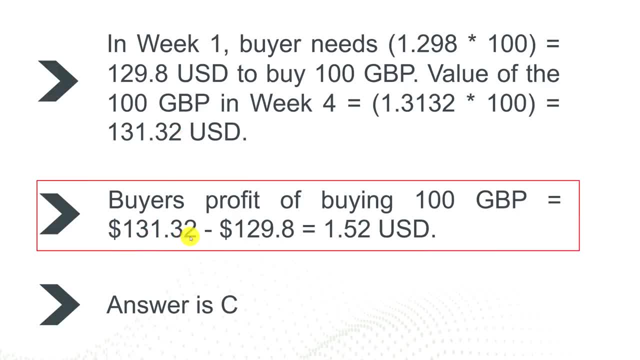 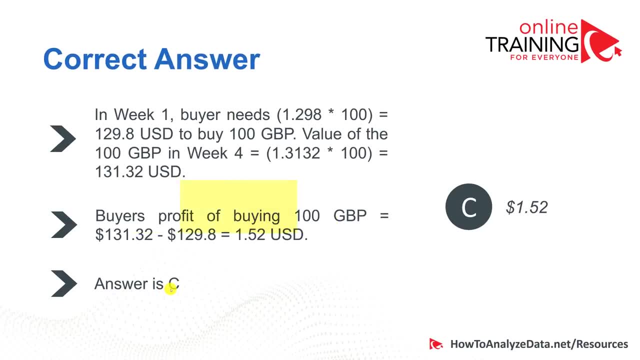 so the profit will be calculated as the difference between 131.32 and 129.8, and would be equivalent of $1.52.. So the correct answer is C here. I hope you've got this one right, But in case you need to practice more, 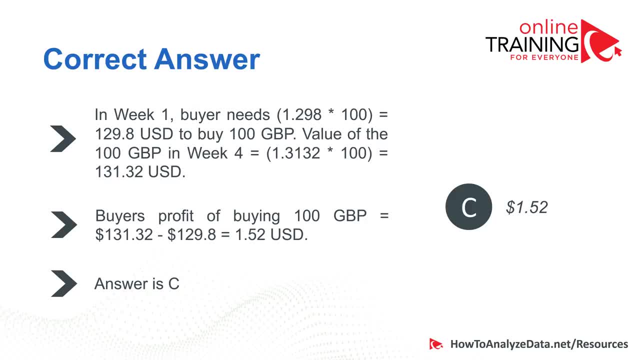 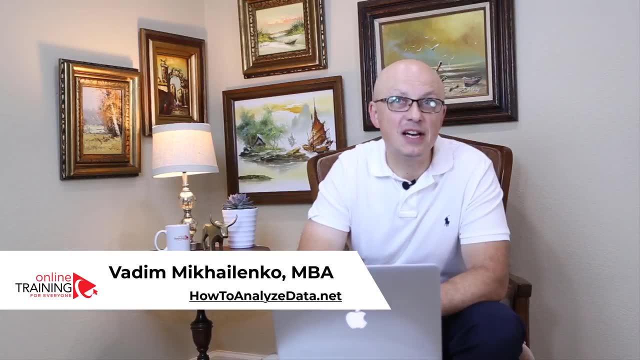 make sure to download my eBook with more practice questions using the link in the description of this video. Can I ask you to do me a favor? passed Employment Assessment Test. please share the questions that are being asked during the test. This will help all of us learn and better prepare for the upcoming test. 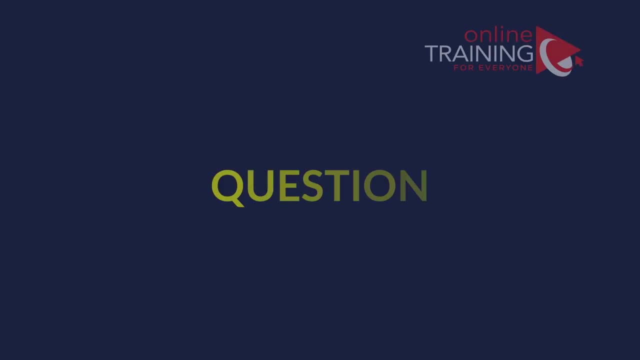 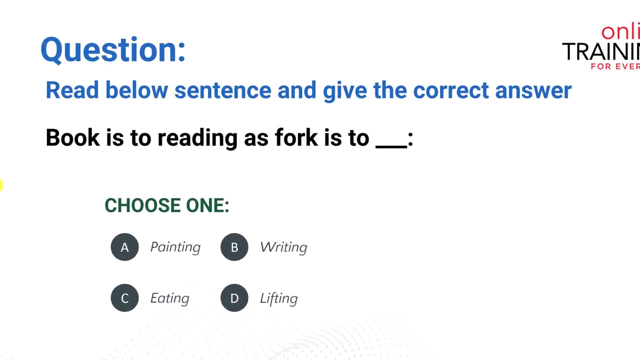 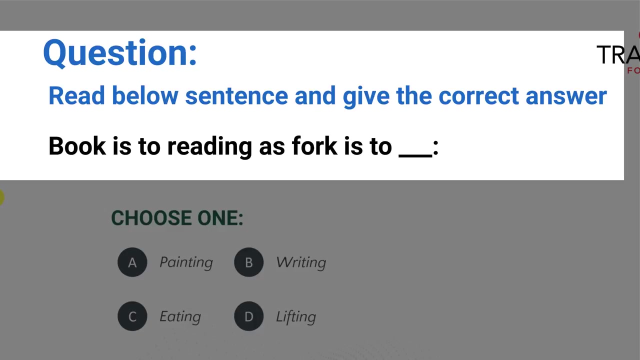 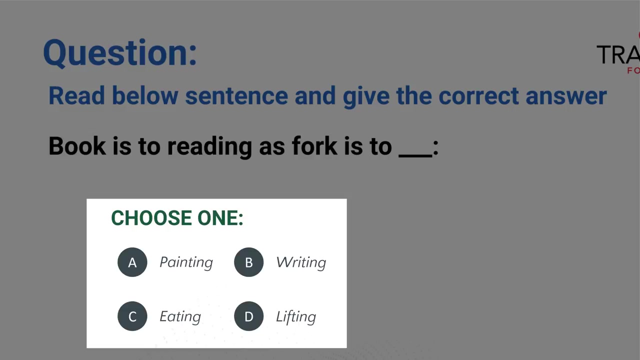 Now let's continue and get you ready for the assessment test. Now let's look at the reasoning question, where you need to complete the sentence Read below sentence and give the correct answer- Book is two, reading as fork is two- and then you need to pick one of the four choices: Painting, writing, eating and lifting. So what do you think? 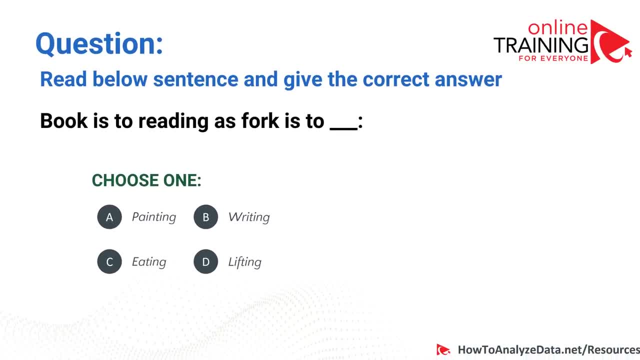 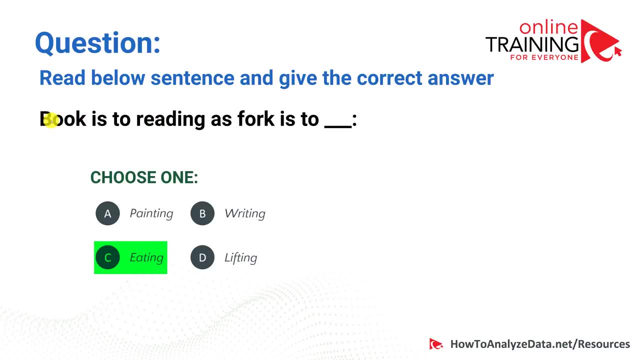 is the right choice. I think it's pretty obvious here, but let's look at the right answer. So the correct answer is obviously eating right, Because book is two reading. This is an activity associated with reading, as fork is two eating. You use fork during the meal consumption, So the 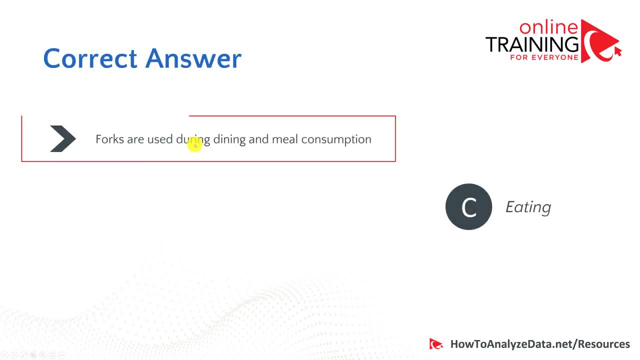 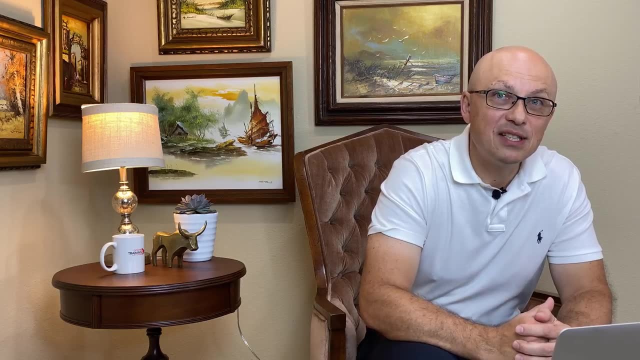 correct choice is C, and that's because forks are used during dining and meal consumption. Hopefully you've got this one right. Let me give you a tip on how to plan your time during the test. As you're probably well aware, most of the assessment tests are timed. One thing you can: 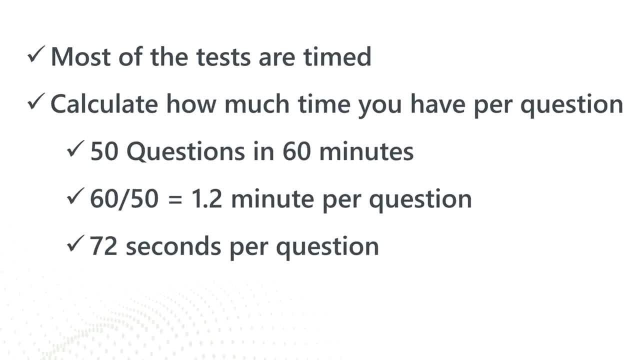 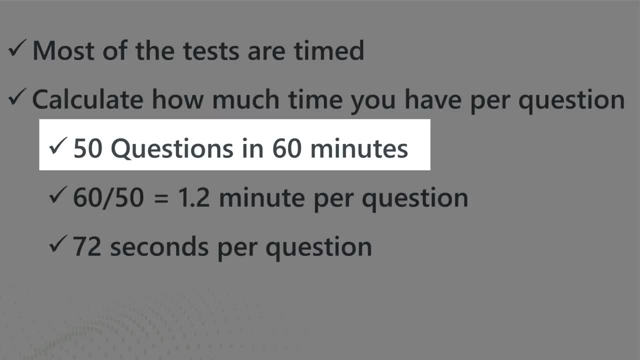 do to increase your chances of passing the test is to calculate how much time would you have per question. For example, if you have 50 questions that you need to complete in 60 minutes, you can do a quick math in your head By dividing 60 by 50, it will give you the answers that you need about. 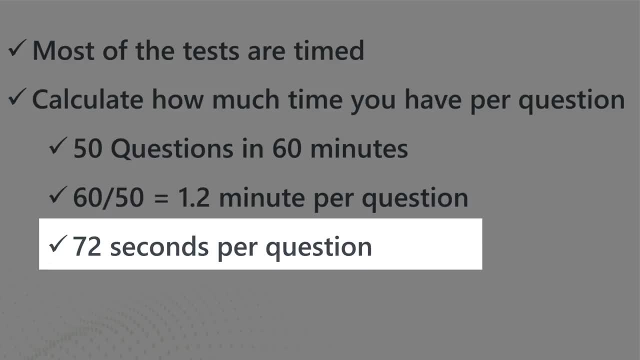 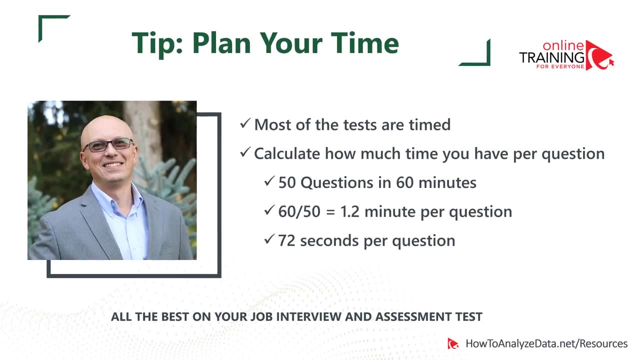 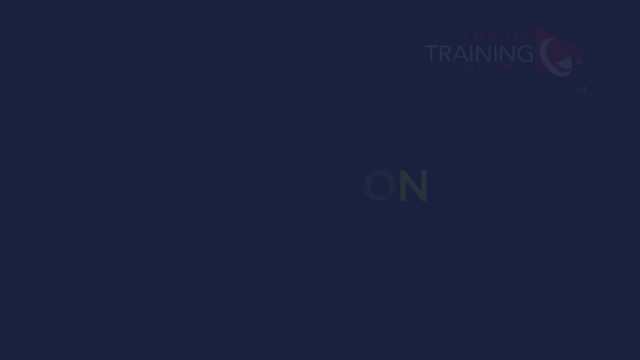 60 seconds per question, which is an equivalent of 72 seconds per question. Having this information handy will tell you how much time you need to allocate per each question. Now let's continue and get you ready for the assessment test. Now let's look at the question where you tested, not just how well you know English. 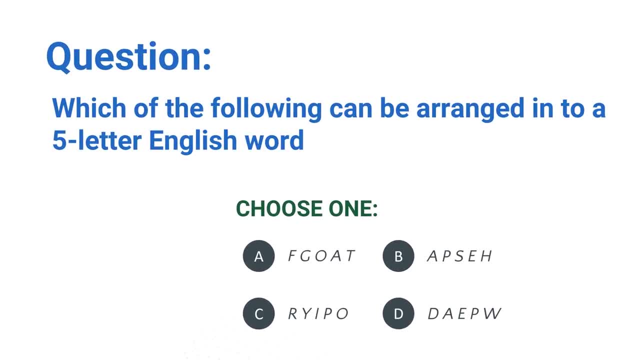 but also how well can you operate with the letters and take guesses based on the questions asked. A lot of times these types of questions used in the verbal reasoning test and in a lot of other tests as well, For example, psychometric tests or logic reasoning tests. 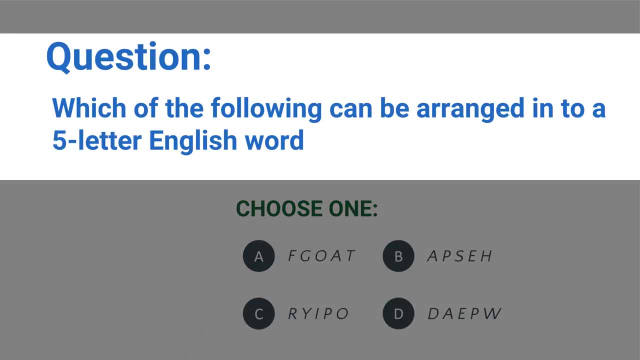 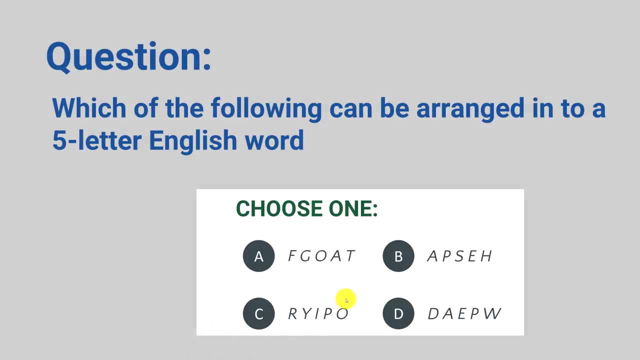 these types of questions we see all the time. So the question: which of the following can be arranged to a five-letter English word? And there are four choices with five letters of the words and you kind of would need to look at each choice and you would need to take a guess. 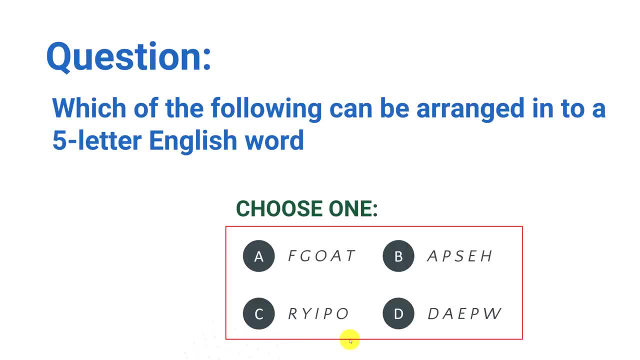 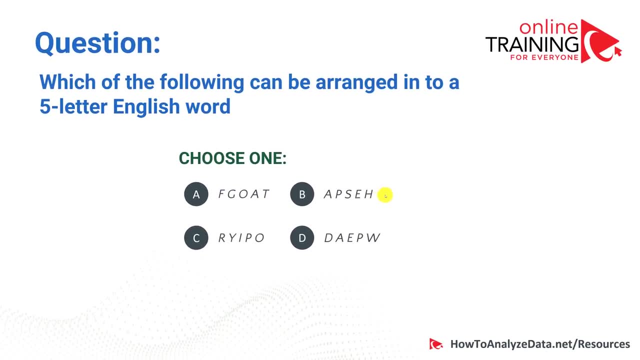 which one would be the one which leads to a specific English word, And obviously nobody gives you the English word, so you would have to take a guess on the word and combine these letters So they will be represented by the specific English word. So which one do you? 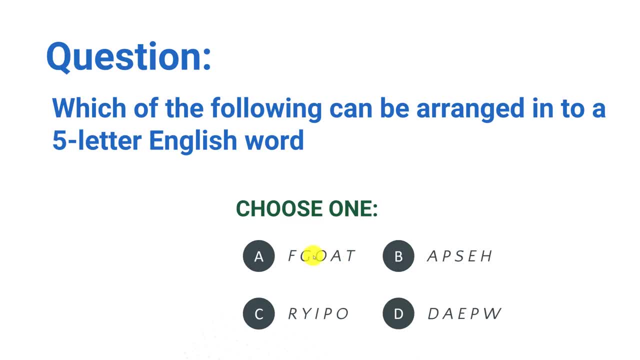 think is the right choice. A couple suggestions here. You see, choice A has inside of these letters English word goat. So typically it's the wrong choice because typically you wouldn't be able to easily rearrange this word into something else. Typically- and again it's only typically- 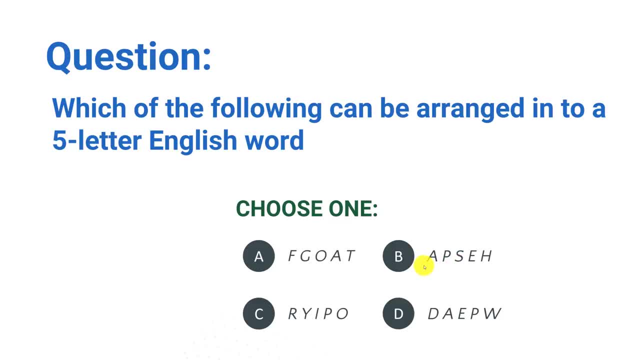 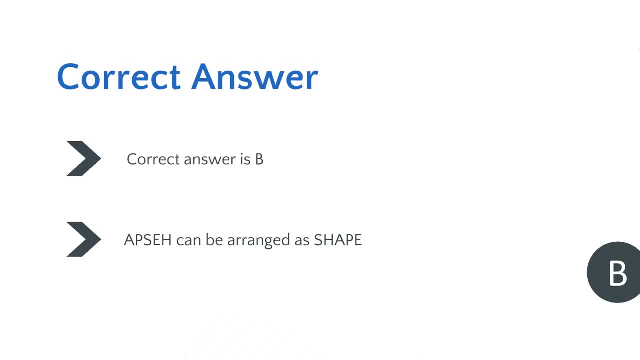 but you would want to start with the letter somewhere in the middle, and the right choice here is choice B, and it's the word shape. That's really the word that, the end result of it. You don't have a way of knowing right because you don't know what the end word. 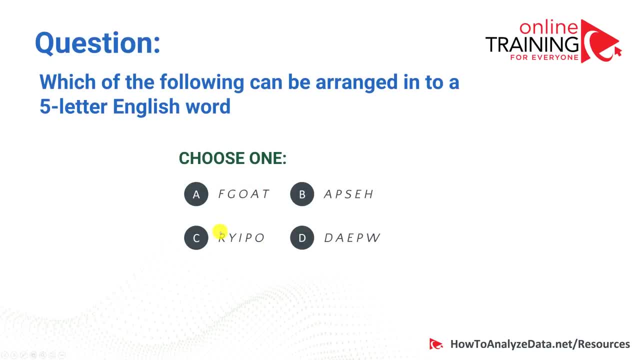 is So you would have to look realistically at all the different choices and see if you can combine them. But I would start with the middle letter, because typically they try to trick you and first letter is typically not the one that starts this new word. So find more exercises like this. This: 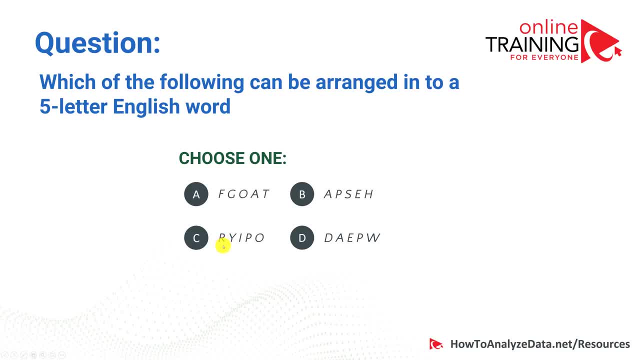 one was difficult. Very few people guess it right, but it takes practice to get these types of questions correctly. So make sure Google or find on the internet these types of verbal reasoning questions and see if you can get better at this. Let me share with you some information that you 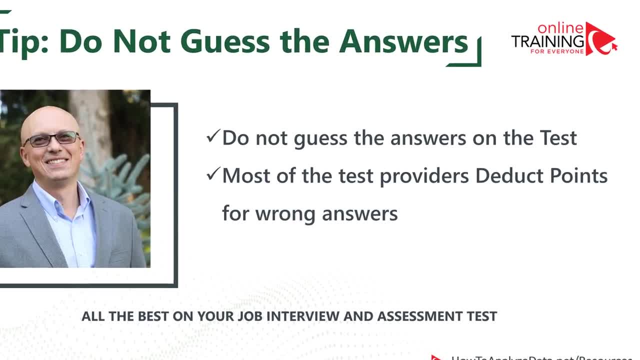 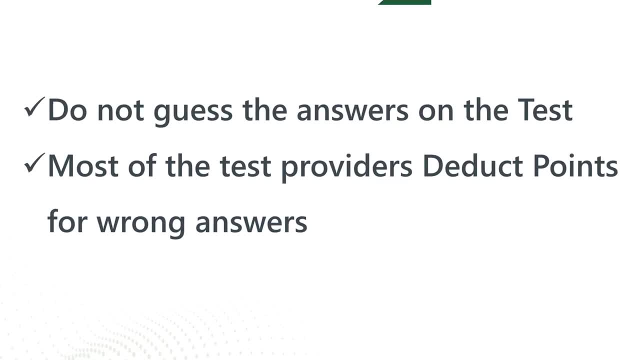 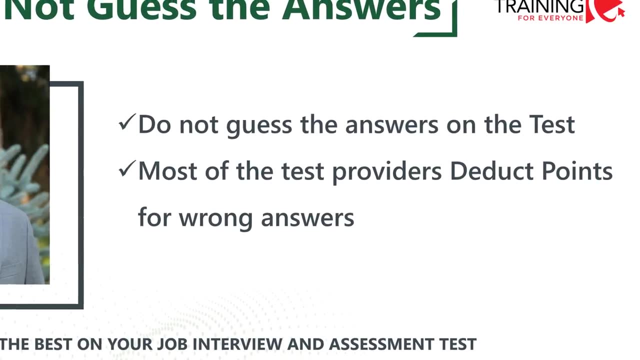 probably don't know. Based on our recent research, most assessment test providers deduct points for incorrect answers, so it is not a good idea to guess answers during the test. You can ask the assessment test to see how they handle incorrect answers If they deduct points for incorrect. 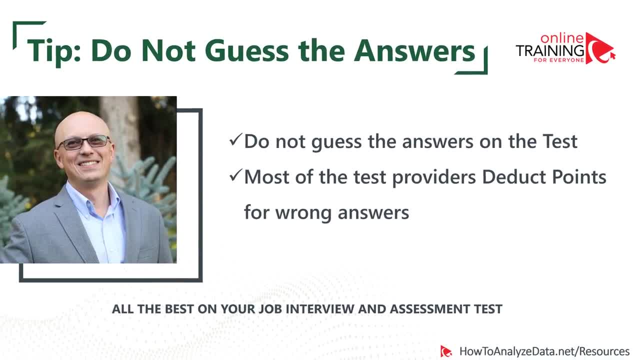 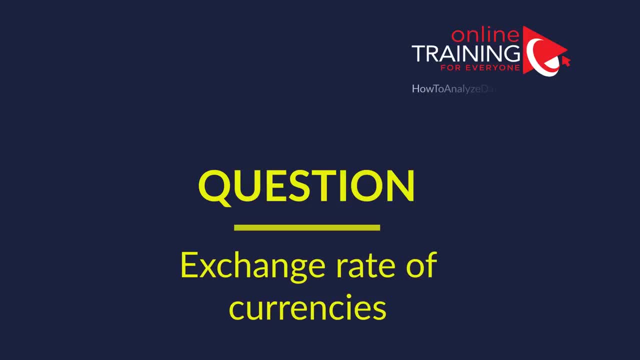 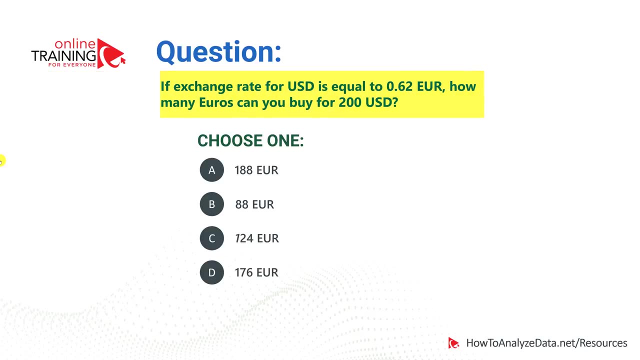 answers. you might consider skipping the questions where you do not know the answers to. Now let's continue and get you ready for the assessment test. Let's look at the question you might get as part of the interviewing with financial organizations: If exchange rate for US dollars, 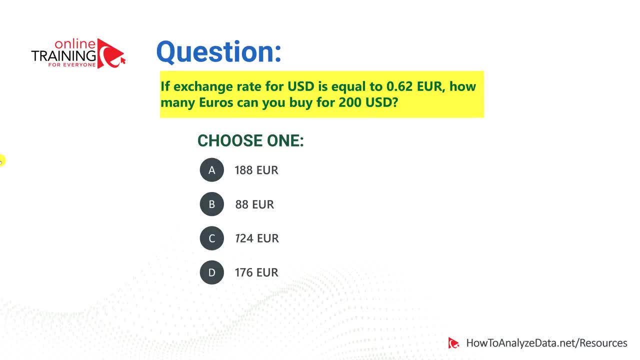 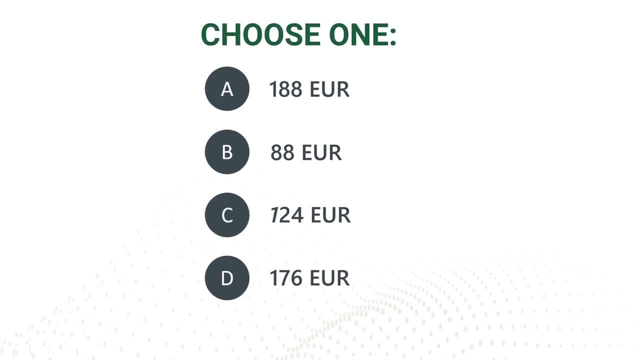 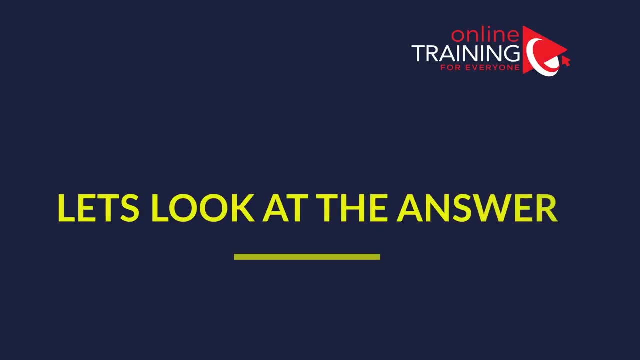 is an equivalent of 0.62 euros. how many euros can you buy for $200?? And there are four choices: $188,, $88,, $124, and $176.. Which one do you think is right? A lot of times when answering this, 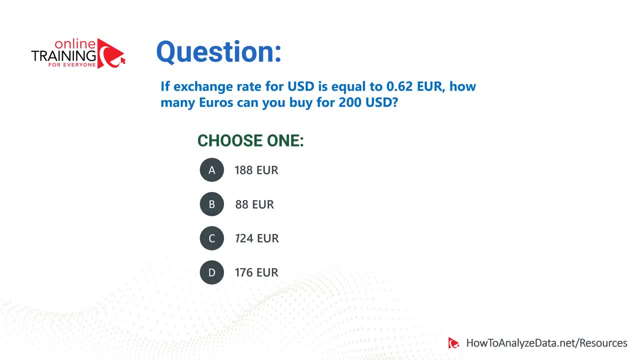 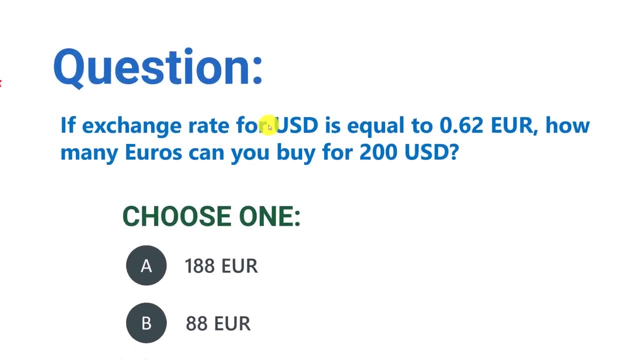 question. you may not have access to the calculator, so you may need to do the math in your head. To do the math in your head, the easiest way is to do it for $100.. For $100, you'll be able to. 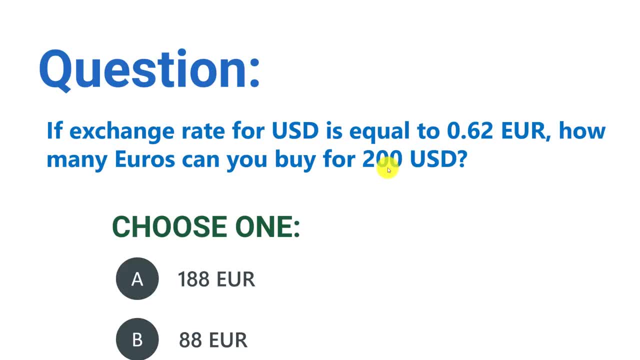 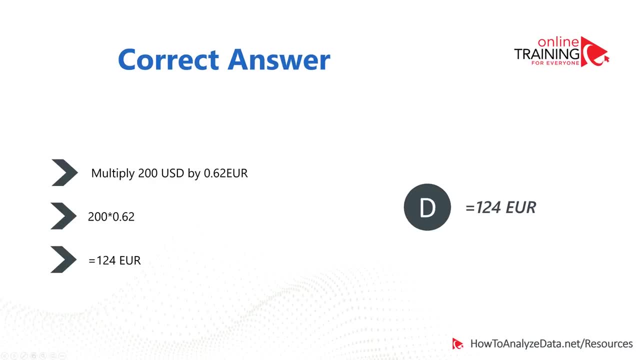 buy 62 euros, Then for $200, you'll be able to purchase double of that, which is 62 euros. Let's recap: To answer this question, you need to multiply 200 by 0.62, which is an equivalent. 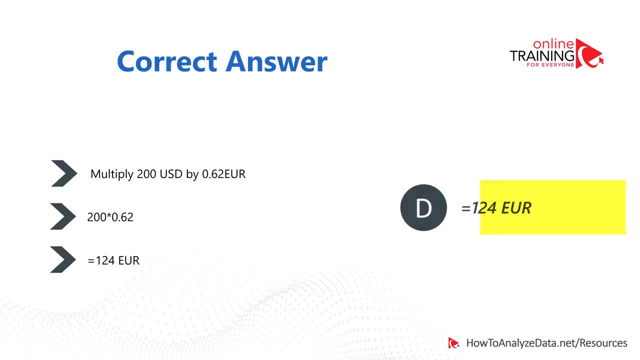 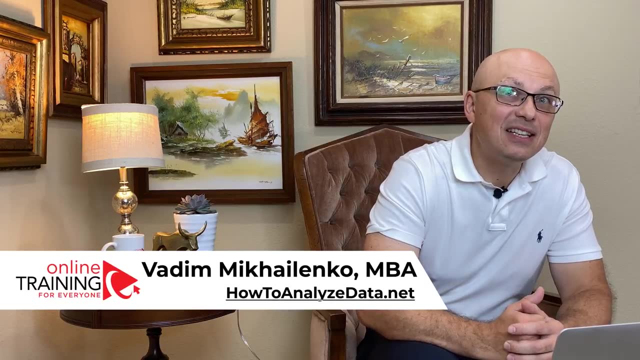 of 124. So choice D is the right answer. I'm pretty sure you nailed this question. A lot of students ask me: what are the smartest ways to learn? Let's look at the different options available to you. Let me share with you some ways to learn new material that work for me. 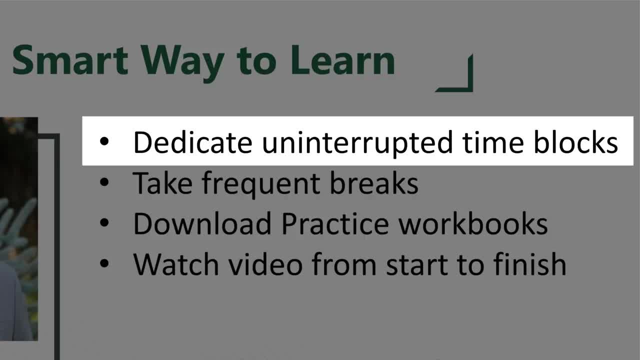 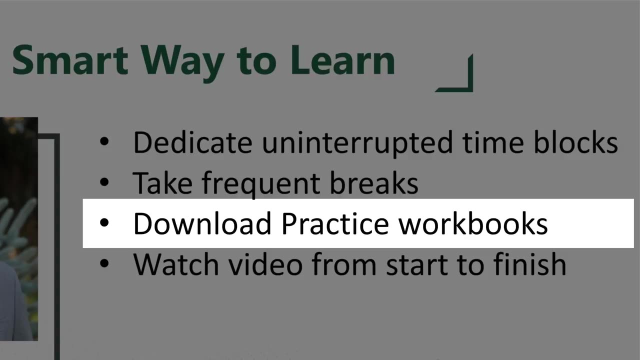 I typically use dedicated, uninterrupted channels. When my attention drifts, I try to take a break and I typically do it every 25 to 30 minutes. I recommend that you download workbooks to practice the hands-on steps, which helps you reinforce the steps and better learn the material. 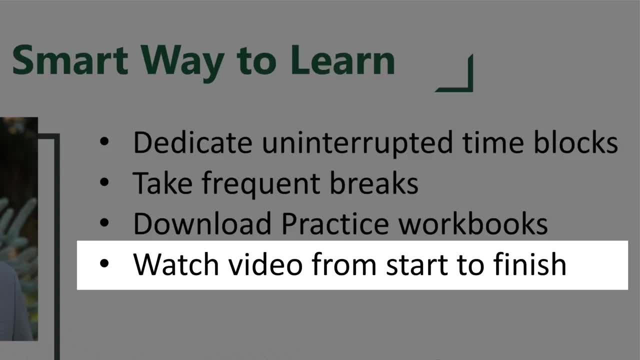 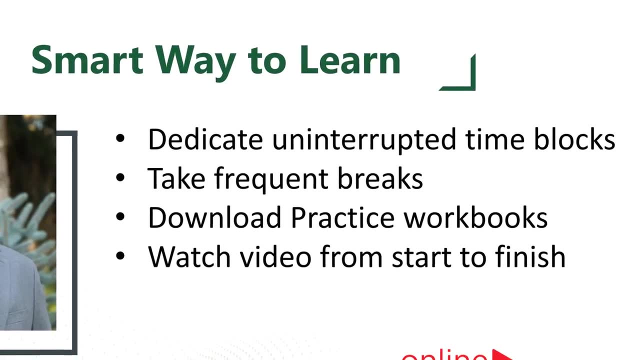 When I try to learn something, I try to watch videos from start to finish in one sitting. I use different playback speed to make sure the material keeps me engaged. I also try to give myself time to absorb the content And if something is not clear I try to pause the video. 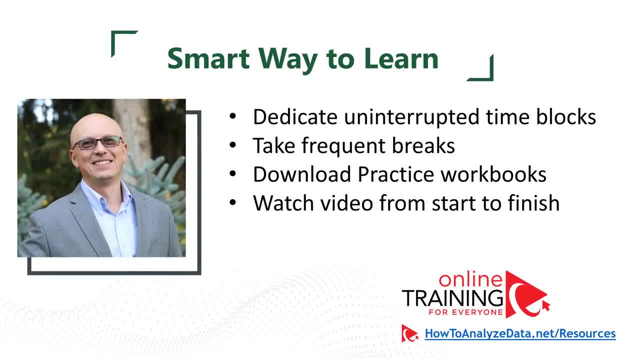 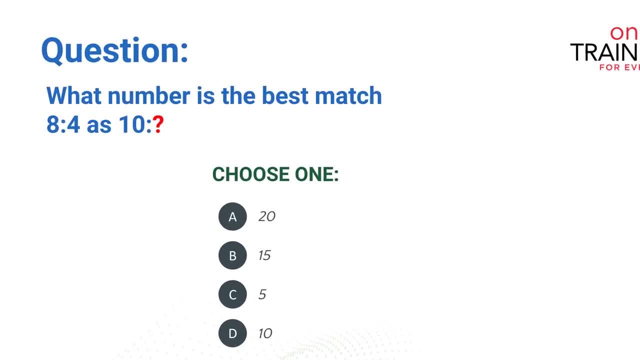 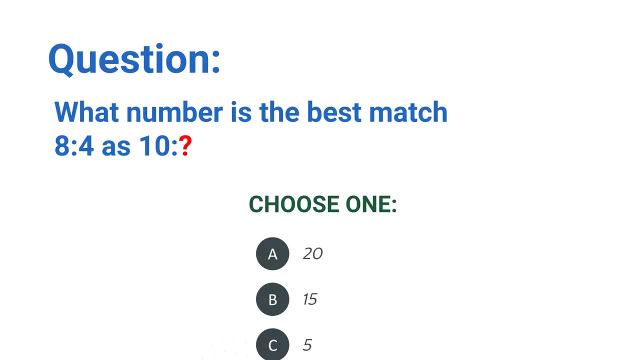 and sometimes I even go back to review material more than once. So let's look at another tricky question: What number is the best match? And we have 8 to 4 would be 10 to question mark. So what do you think is the right one here?